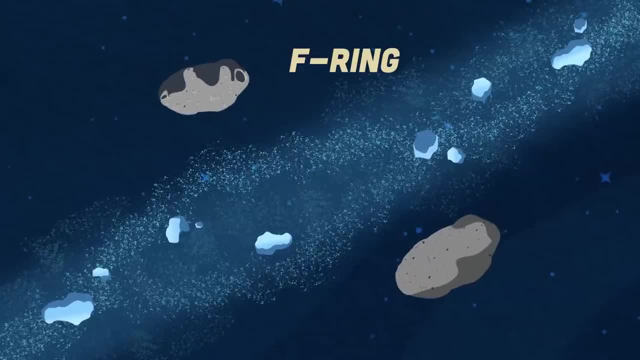 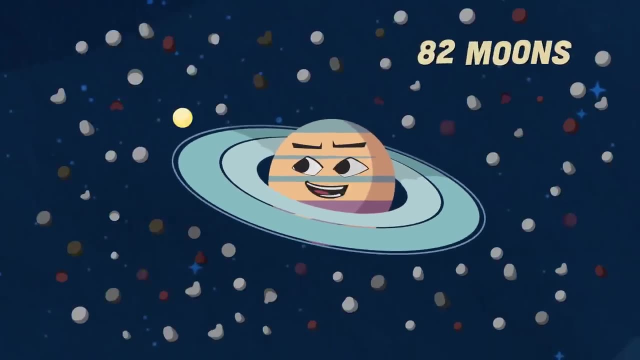 These particles and moons make up my F-ring, a narrow band which is 60 miles Miles wide. I sing, I'm Saturn and I have 82 moons From the date of this song's release. there may be more soon. 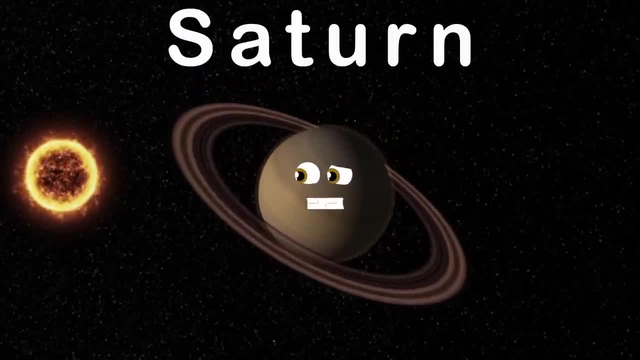 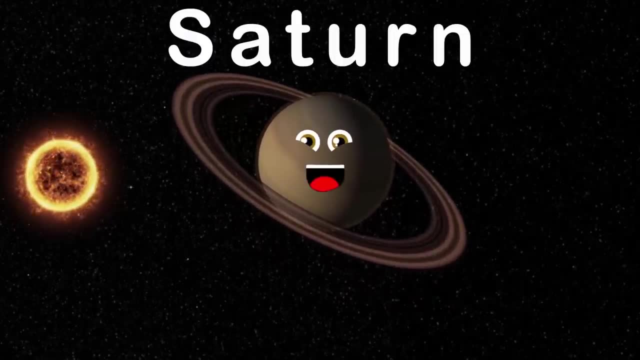 I am Saturn, the sixth planet from the Sun. I'm known for my rings by everyone. I'm the second largest planet in our solar system. Please come sing along until my teachings are done. Out of my 62 moons, 53 are named. I am a gas giant—all astronomers claim. 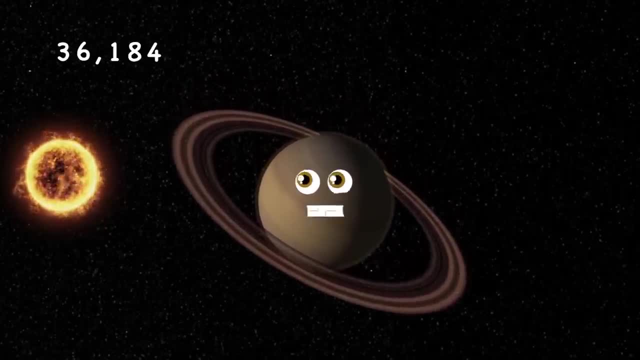 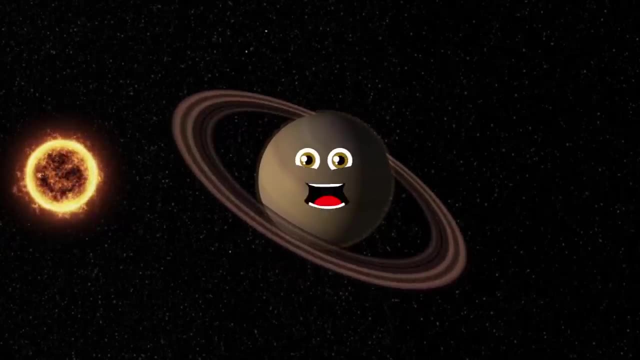 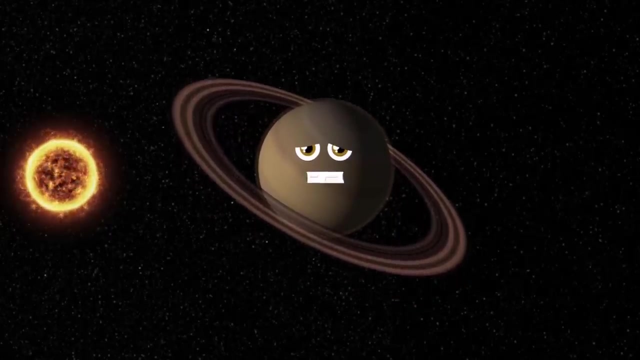 Thirty-six thousand one hundred eighty-four is my radius of miles for you to explore. Ten point forty-four meters, that's per second you drop. That's my gravity pulling towards my surface. top Ten hours and thirty-nine minutes long is the day on my surface. Let's sing this song. 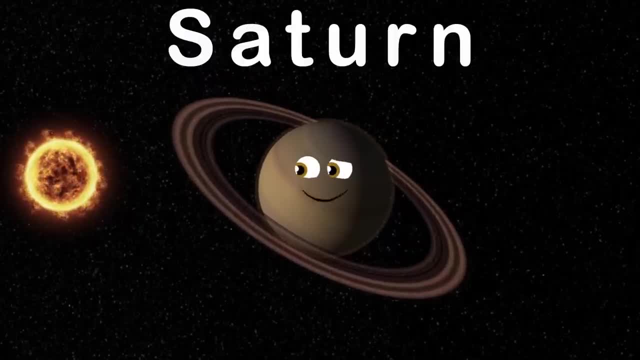 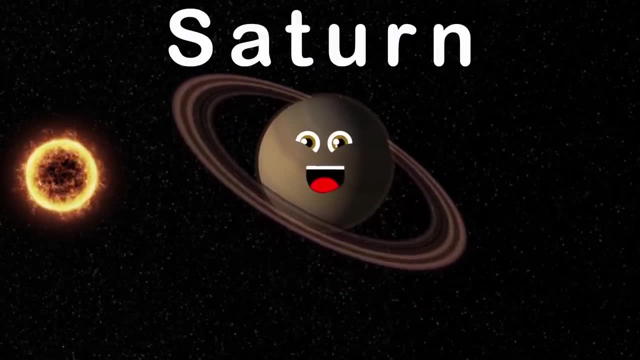 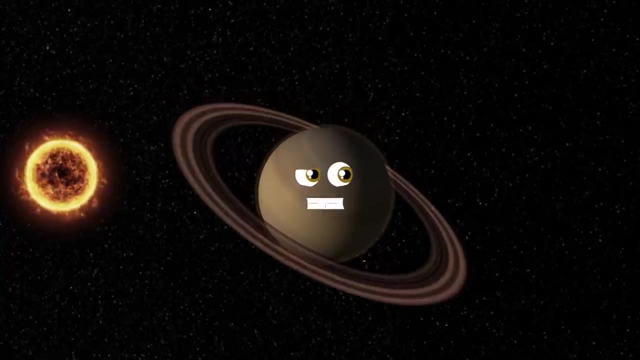 I am Saturn, the sixth planet from the Sun. I'm known for my rings by everyone. I'm the second largest planet in our solar system. Please come sing along and tell my teachings are done. Takes 29 years for me to orbit the sun, And my rings are made up of rock and icy chunks. 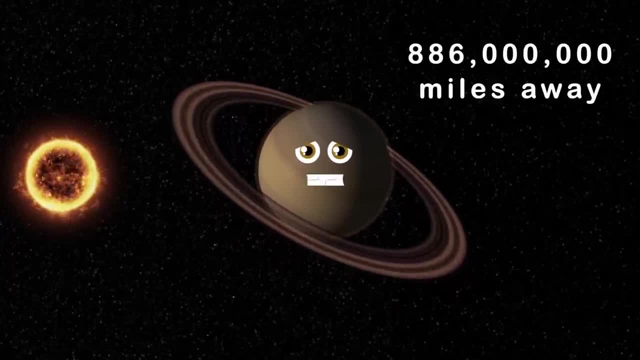 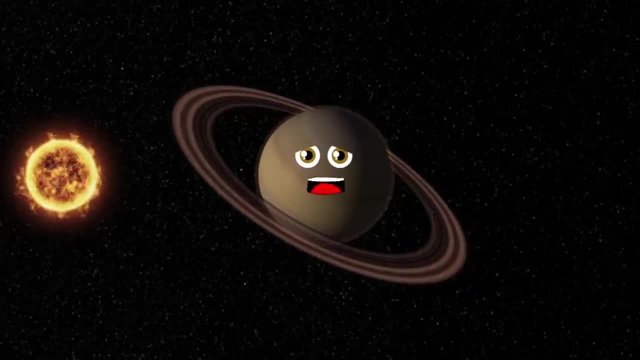 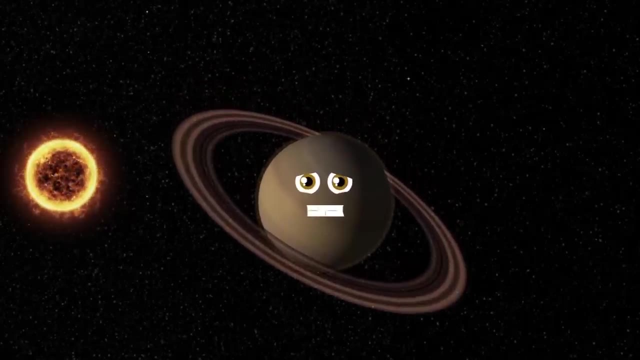 886 million miles away Is my distance from the sun. that is why I'm Chile. Hydrogen and helium are what I'm mostly made of, And my atmosphere from the surface above 26.7 is the amount of degrees I spin on my axis. I'm so cold that you freeze. 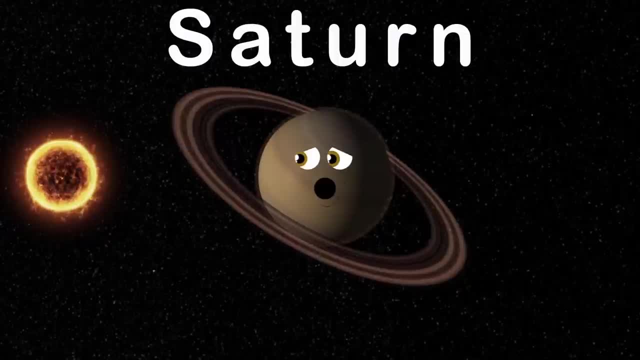 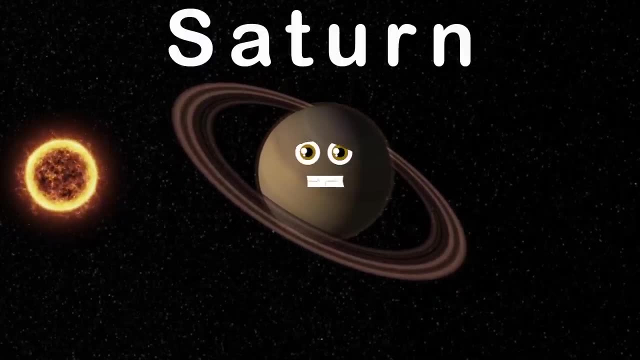 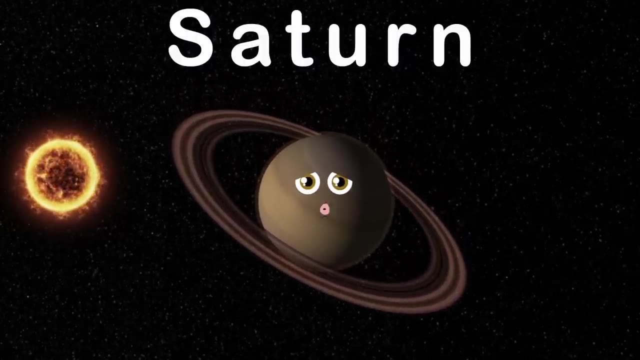 I am Saturn, the sixth planet from the sun. I'm known for my rings by everyone. I'm the second largest planet in our solar system. Please come sing along and tell my teachings are done. I am Saturn, the sixth planet from the sun. I'm known for my rings by everyone. 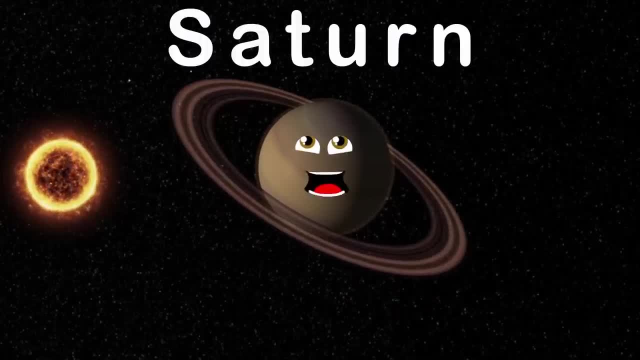 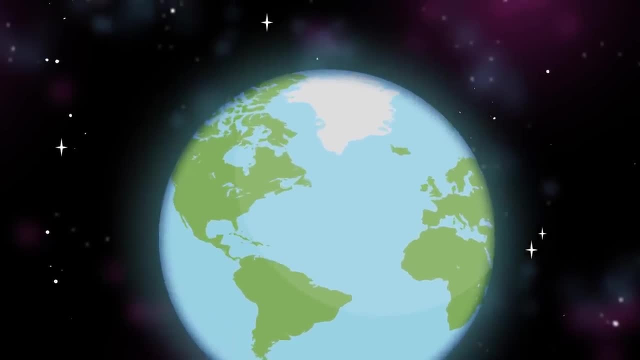 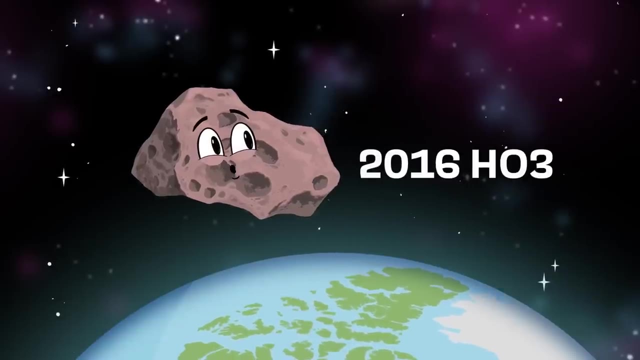 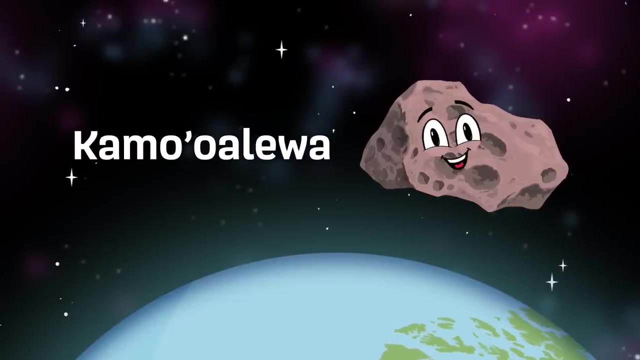 I'm the second largest planet in our solar system. Please come sing along and tell my teachings are done. Earth. as the second moon, It's me. provisionally designated 2016 H03 Camu Abrava is thought to be an asteroid, But that may have changed with new facts that we can avoid. 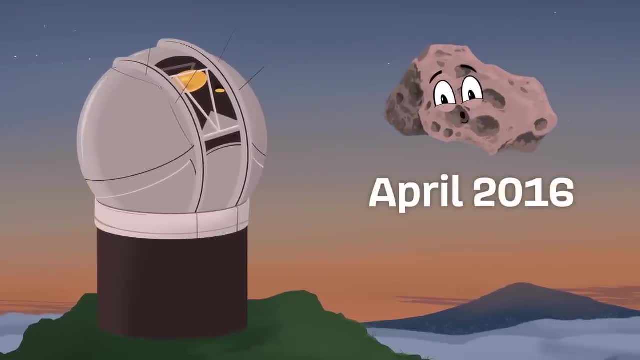 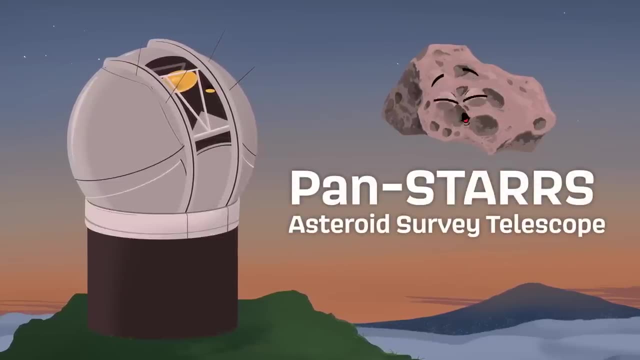 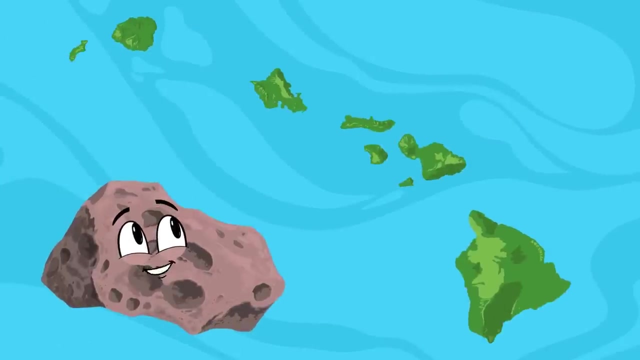 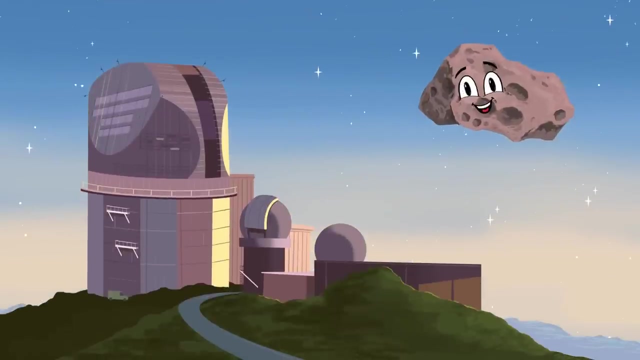 I was first spotted in April of 2016, But I'm the sixth planet from the sun. I'm known for my rings by everyone By Pan-STARRS Asteroid Survey Telescope. You now see, This telescope is located on Haleakala In Hawaii, Which is all part of the 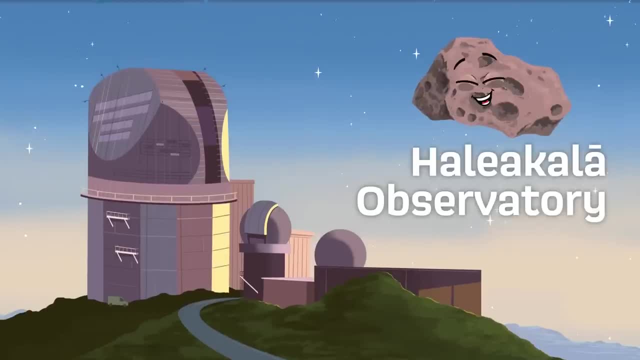 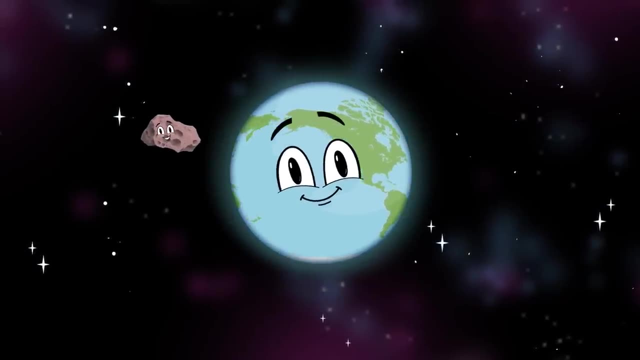 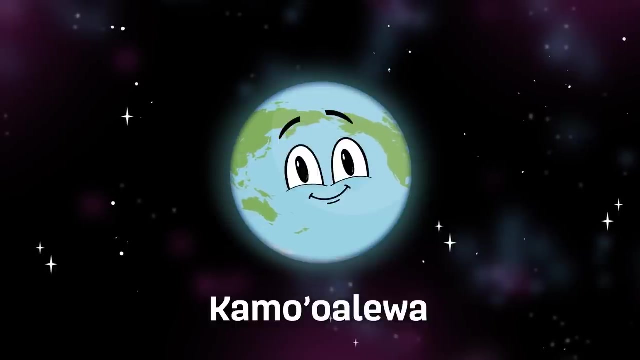 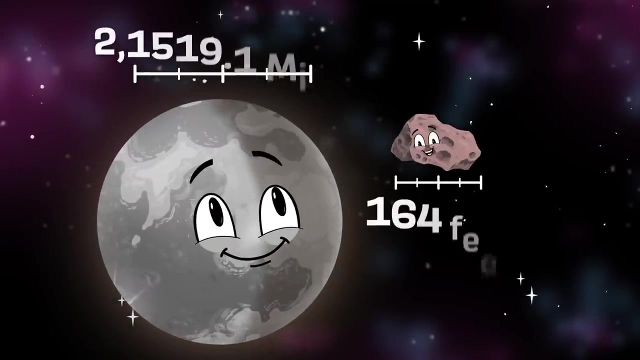 Haleakala Observatory. When I was discovered orbiting the Earth in a weird way, Kambu'u alava was the name they gave me. Even though it is extremely hard to say, I am very small compared to Earth's moon, Measuring 164 feet across. I'm tiny, it's true. 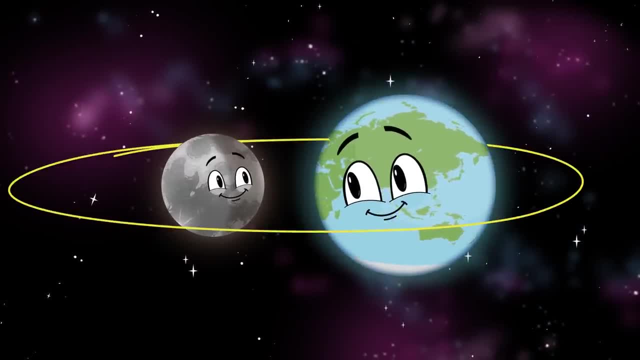 I circle the Earth in a repeating corkscrew like trajectory, Never closer than 4200 times the 239,000 mile distance of the Earth's surface. I am very small compared to Earth's moon, measuring 164 feet across. I'm tiny, it's true. 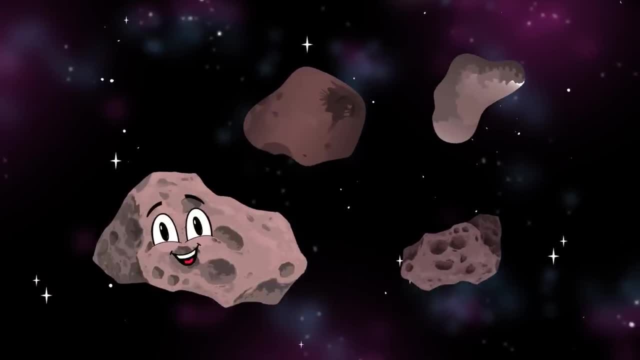 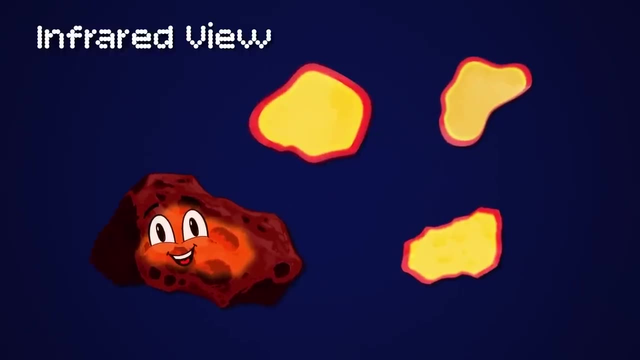 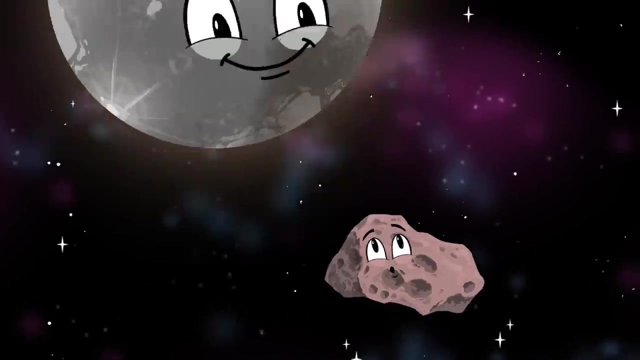 I am very small compared to Earth's moon, measuring 164 feet across. I'm tiny, it's true. I'm odd, and this is why I don't reflect brightly in certain infrared frequencies or to the eye, Like other asteroids do. I'm a quirky satellite, and this is true. Because of this, researchers are starting to 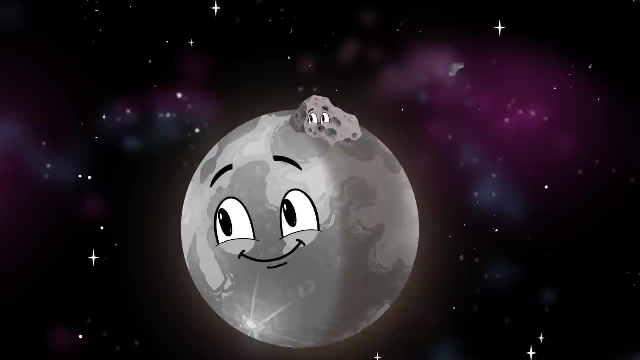 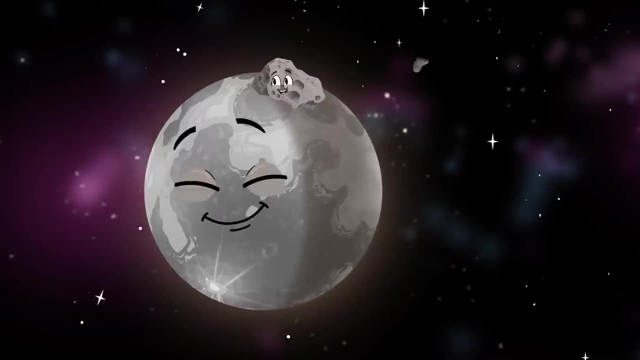 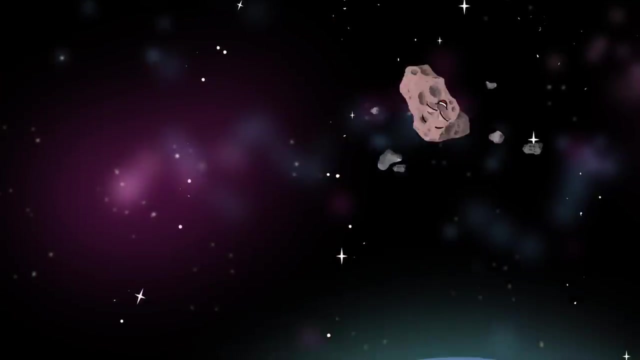 agree, I may be a chip off your known moon flying free. Basically, what you're seeing is a flying silicate Caused by micrometeorite impacts in the space environment. It's possible when space rocks hit the moon at a high degree. When I was ejected into space, I am lunar debris. 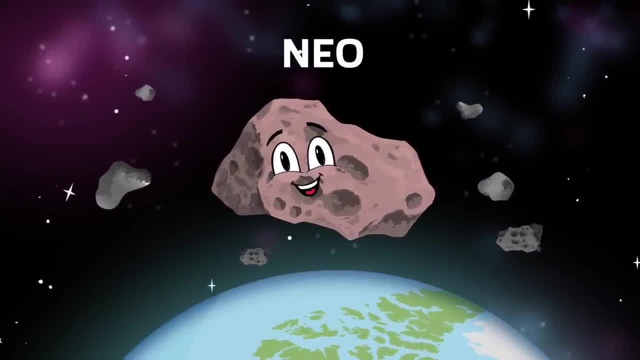 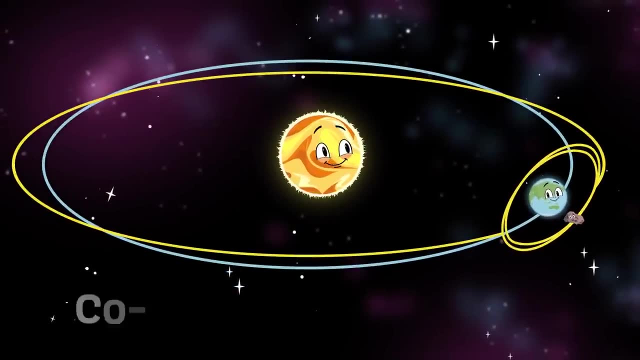 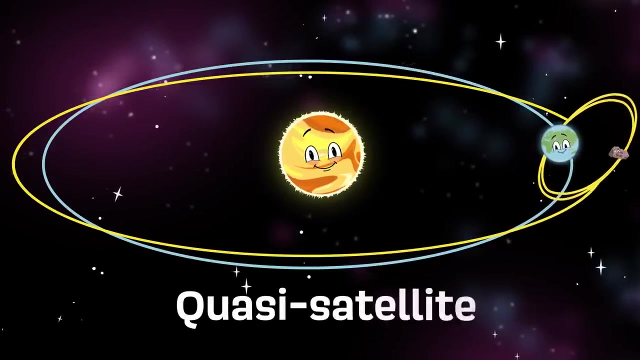 I am a near-Earth object also known as NEO, Part of a group of near-Earth asteroids called Apollo. I'm an object in a specific type of coal orbital configuration with a planet. I'm called a quasi-polar object. I'm called a quasi-polar object. 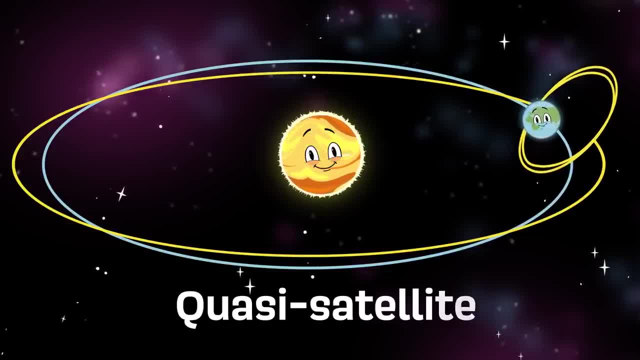 I'm a quasi-polar object, also known as a galactic object Satellite. I know it's weird, But I didn't plan it Earth as the second moon. it's me. Provisually designated 2016 H03. Kamuu. Abrava is thought to be an asteroid, But that may have changed with new facts that. 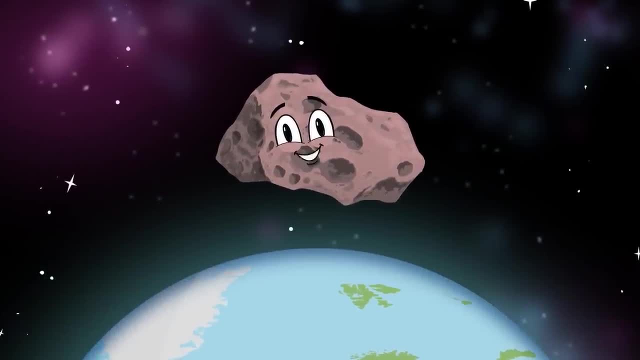 we can avoid. I am a tiny. it's true I'm tiny, it's true. I'm odd and this is why I don't reflect brightly in certain infrared frequencies or to the eye. It's possible when space rocks hit the moon at a high degree. I'm not a chip off your known moon measuring 164 feet across. I'm tiny, it's true. 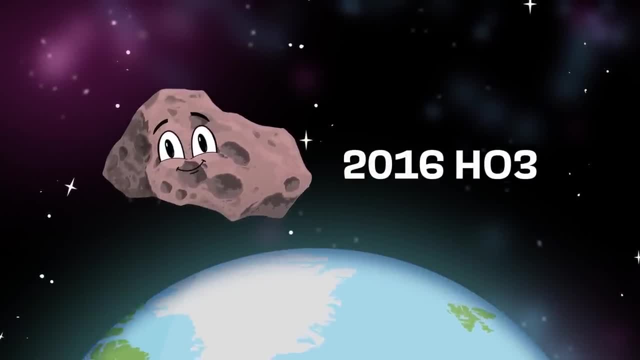 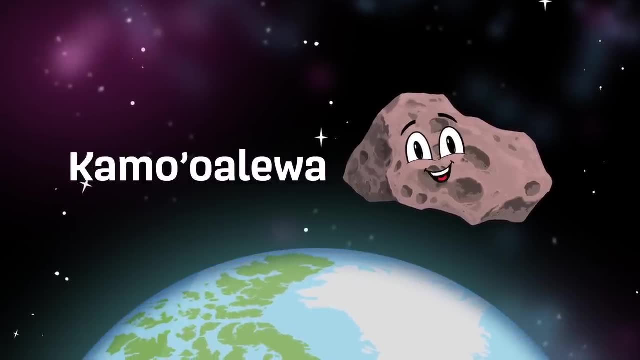 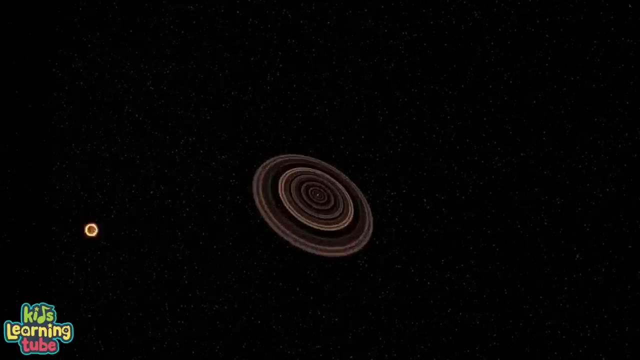 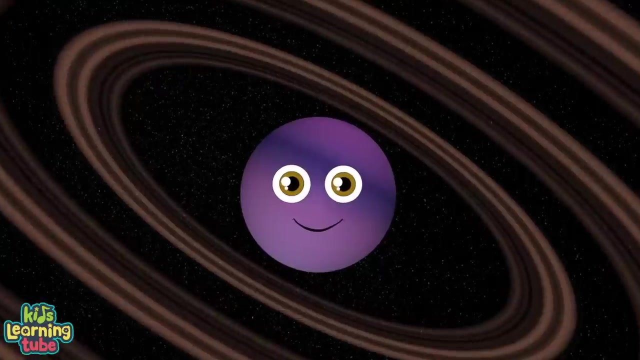 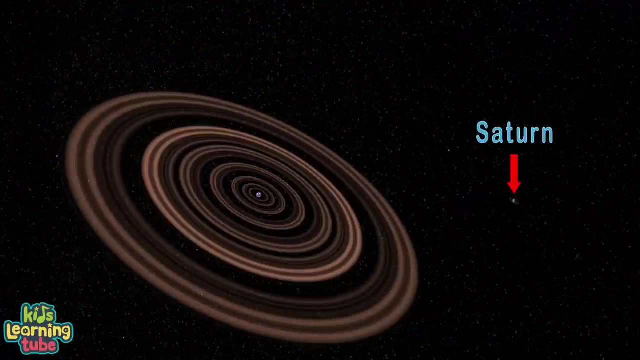 I'm odd, and this is why I don't reflect brightly in certain places. I'm a quasi-polar object, also known as NEO, Part of a group of near-Earth asteroids. My name is J1407B, that's me. I have a ring system bigger than Saturn, you see. 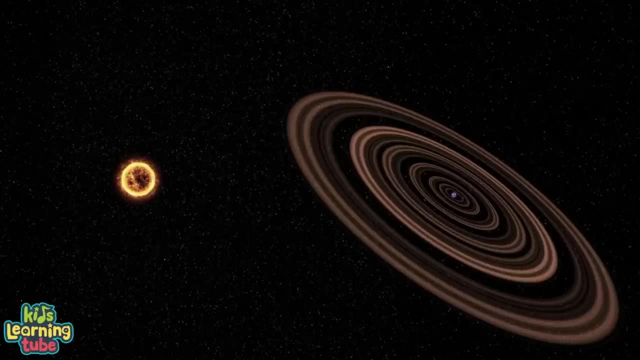 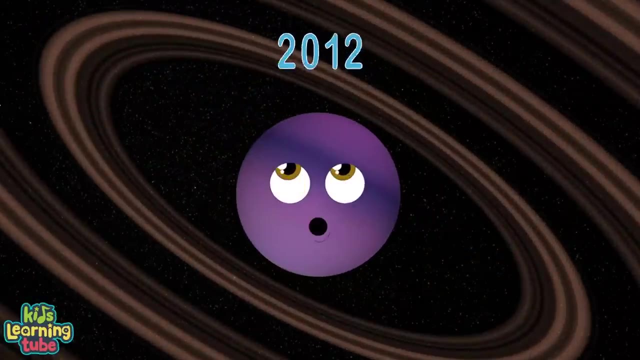 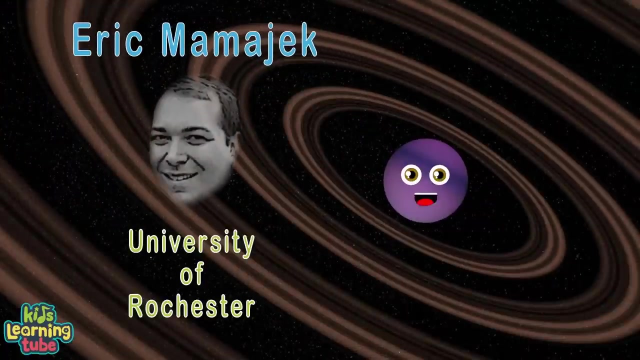 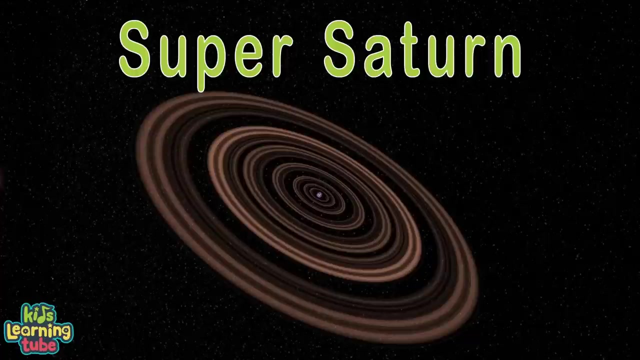 I orbit a young star and we can all agree its name is V1400 Centauri. In 2012,, when I was discovered by Eric Mamajek at the University of Rochester, I earned the name of Super Saturn because of my 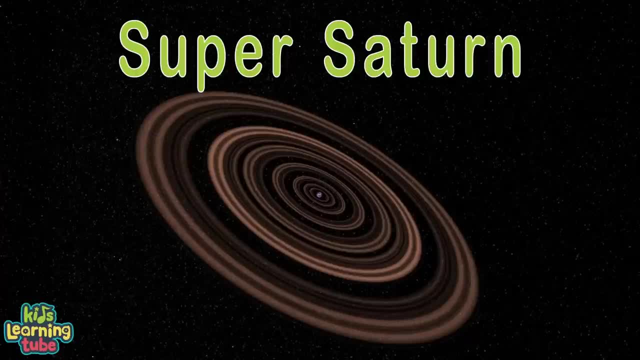 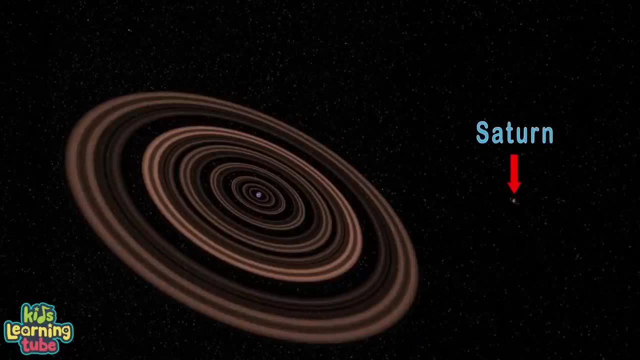 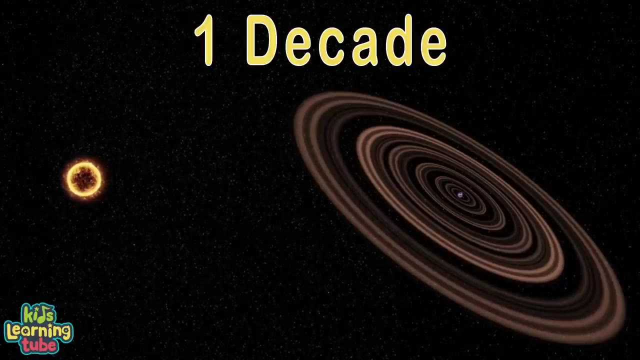 My massive system of circumplanetary rings. for sure, 90 million kilometers is the radius of my rings. That's about 200 times the size of Saturn's rings, which makes me the king. When I orbit my sun, it takes about a decade, which is estimated at about 3,725 days. 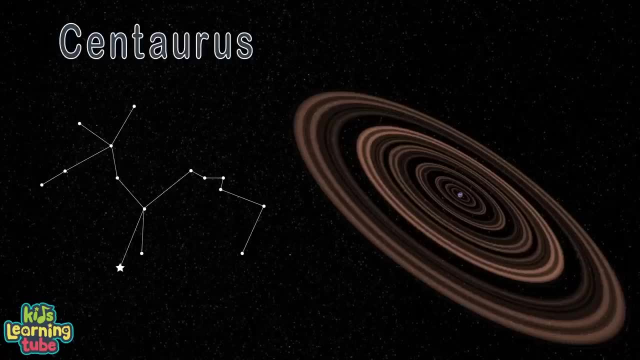 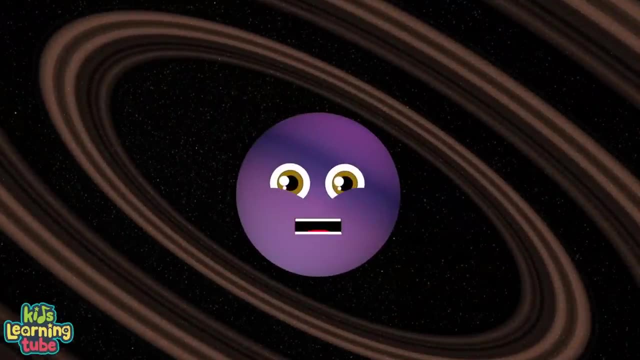 I'm within the constellation of Centaurus. It's about 434 light years. I'm about 3,000 light years from the Earth, but I don't fuss. No one knows if I'm a gas giant or a brown dwarf with rings. 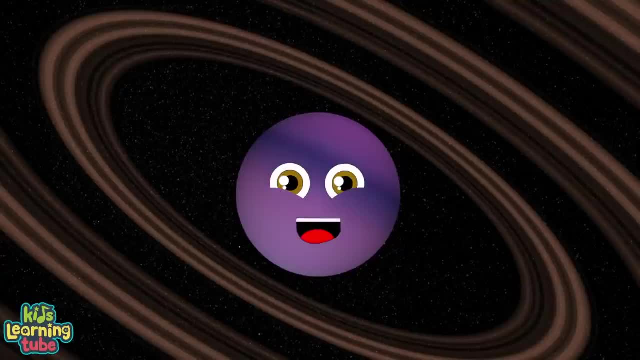 I'm sure you'll find out more about me. while I do my thing, There's a gap in my rings, which probably means one thing: It may have been made by an exomoon of mine about this: I do sing. I also have another name. when I show you, you will see. 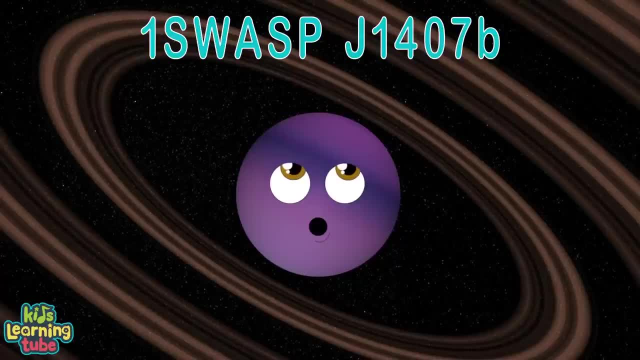 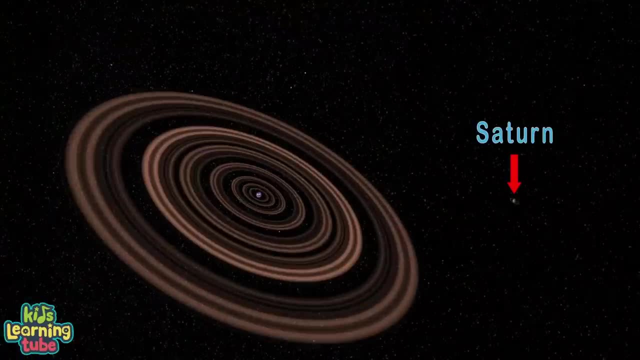 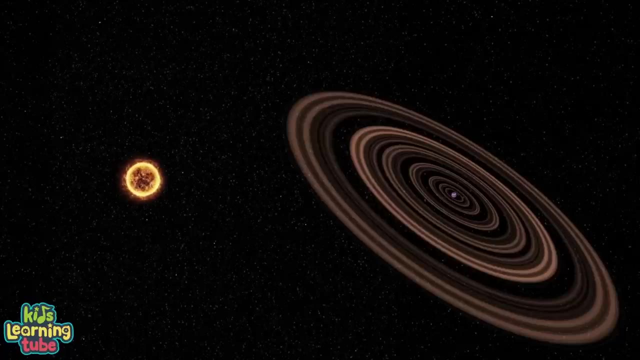 It is 1S Wasp J1407B. My name is J1407B, that's me. I have a ring system bigger than Saturn. you see, I orbit a young star and we can all agree. Its name is V1400 Centauri. 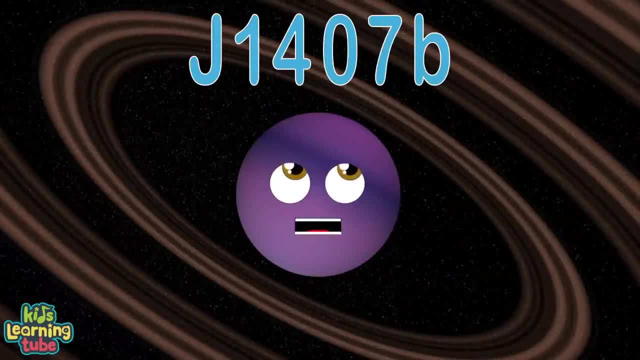 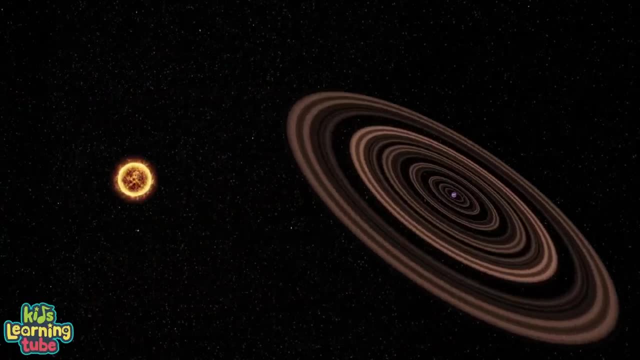 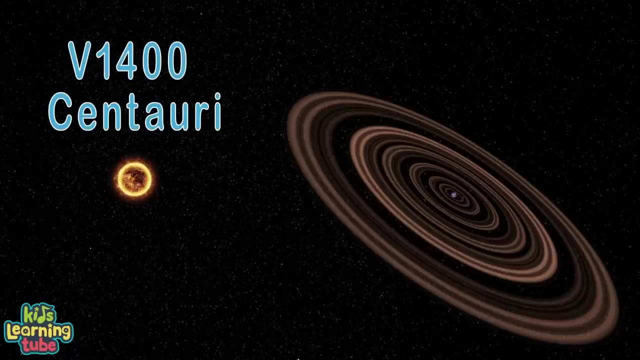 My name is J1407B. that's me. I have a ring system bigger than Saturn. you see, I have a ring system bigger than Saturn. you see, I orbit a young star and we can all agree. Its name is V1400 Centauri. 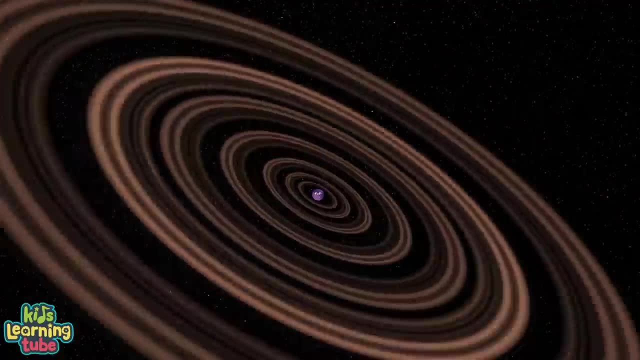 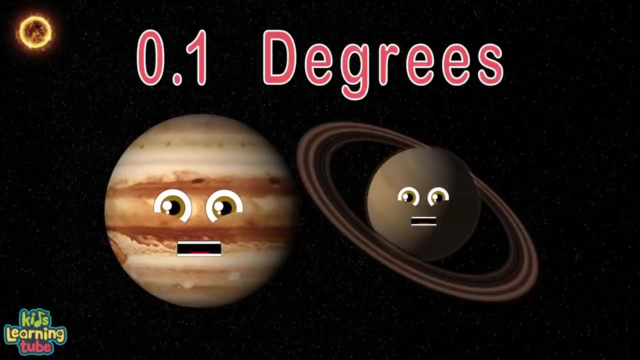 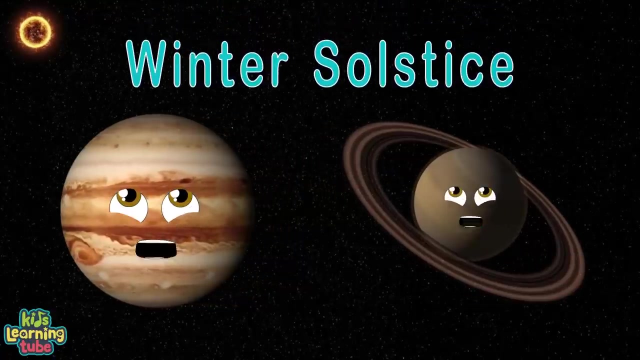 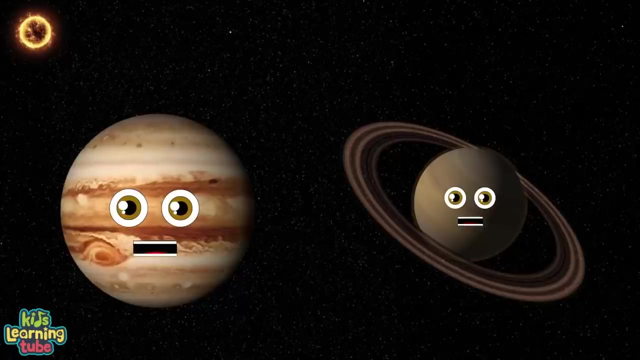 Jupiter and Saturn will come within 0.1 degrees of each other, Forming the first visible double planet in 800 years, will clutter On the winter solstice, December 21st in 2020. Look to the night sky to see this event. the joy it'll bring is plenty. 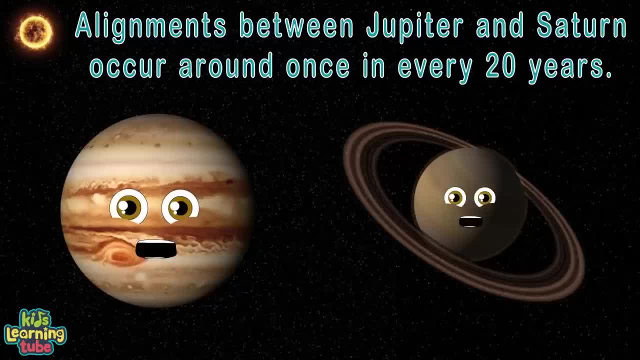 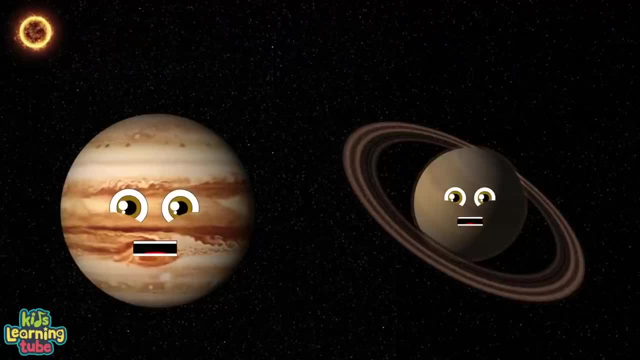 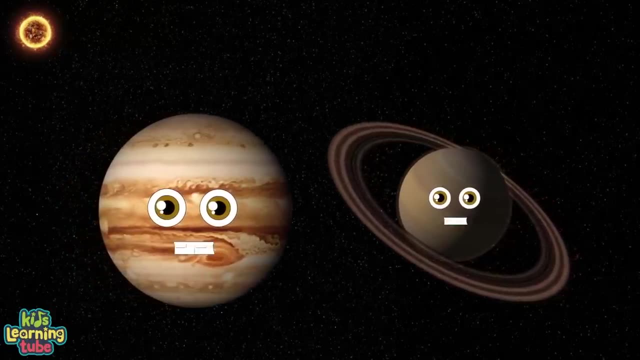 Alignments between Jupiter and Saturn are pretty rare, Only occurring around once in every 20 years. But this upcoming conjunction's exceptionally rare Only because of how close we planets will appear. It's said the sun will rise and the moon will rise. It's said the sun will rise and the moon will rise. 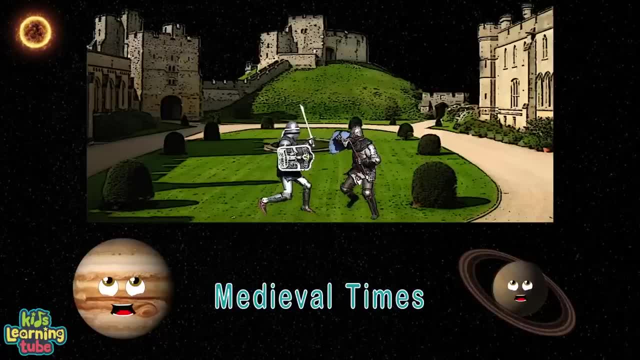 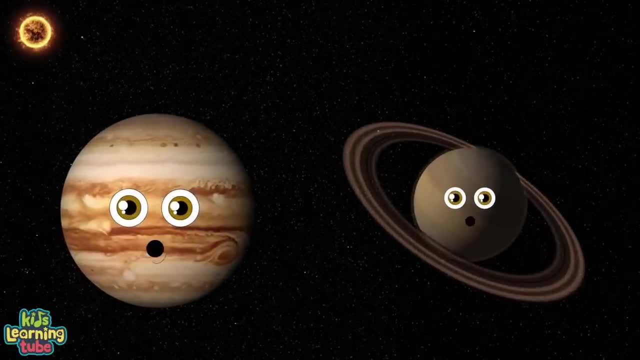 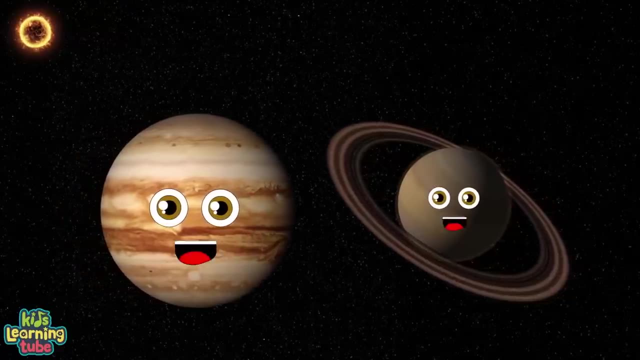 The last time this occurred was in medieval times. In the year of 1226 was the closest that we aligned. Alignments between these two planets happens once every 20 years, But this conjunction will be very rare because of how close we appear. We'll be aligning on the same day as the winter solstice. 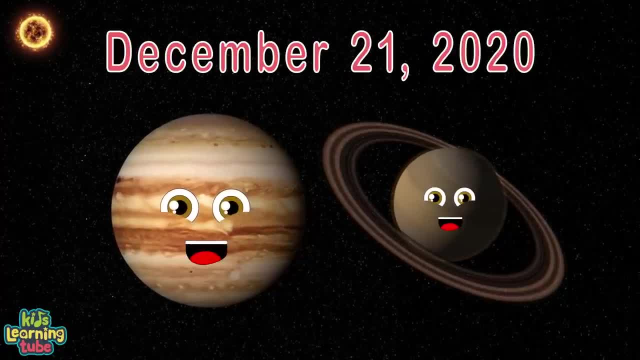 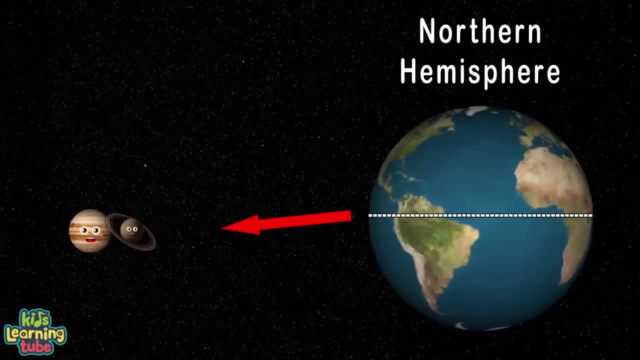 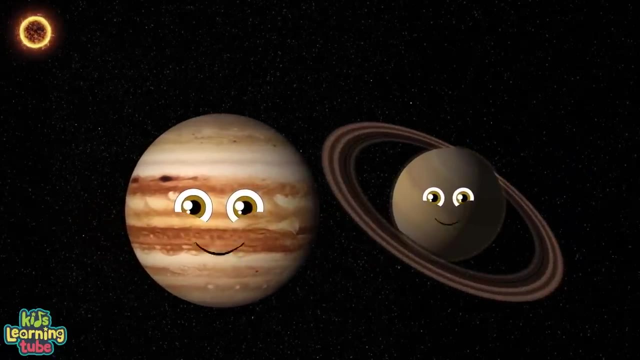 On December 21st 2020,. the whole world can witness this. If you live in the northern hemisphere, you'll see the sun rise. Looking low in the southwestern sky, You can see it shining bright shortly after sunset with the naked eye. We'll appear extremely close for about a month ahead. 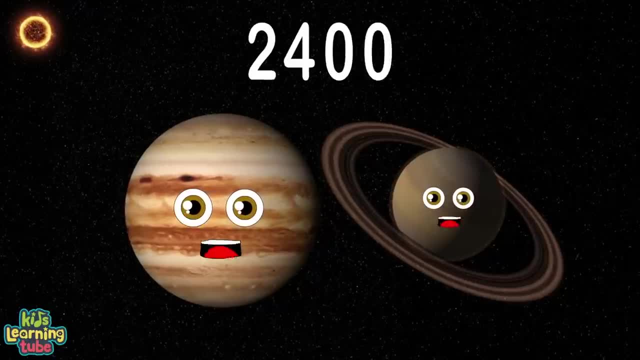 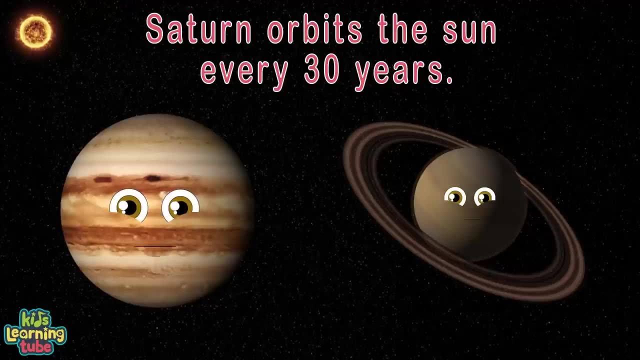 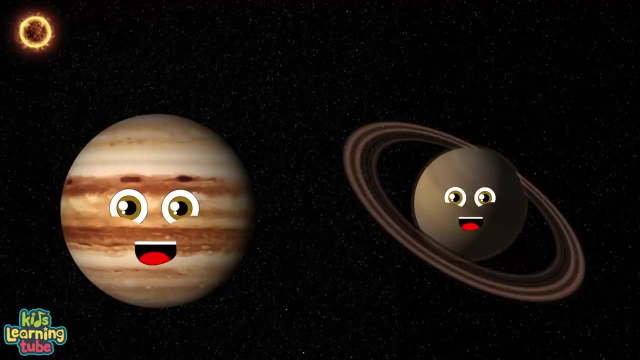 But we won't make such a close approach again until the year 2400. Typically, Jupiter orbits the sun every 12 years. Saturn's orbit around the sun takes about 30 years. Every couple of decades Jupiter laps. Saturn's orbit around the sun takes about 30 years. 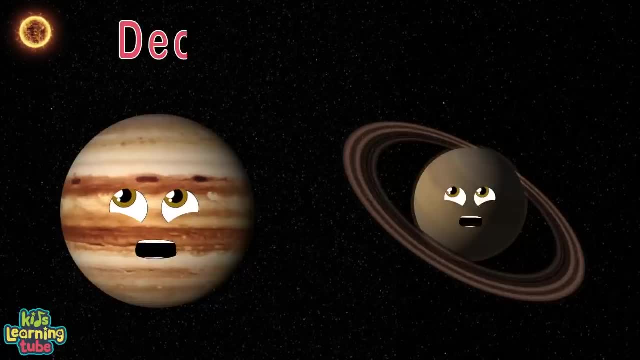 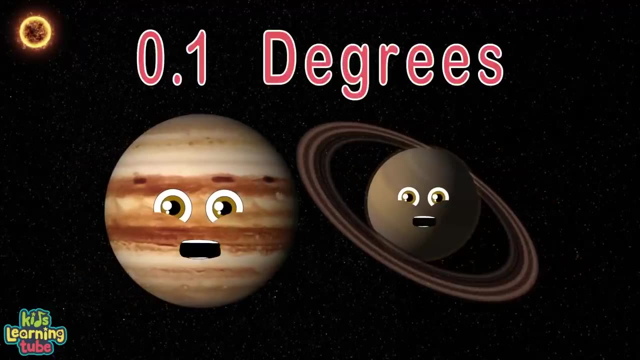 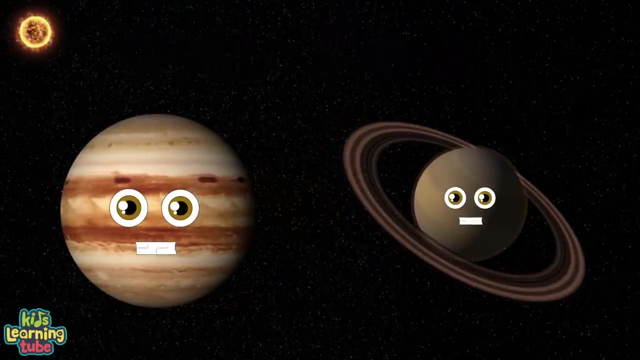 In time. it's 10 years to reach its ideal of a Saturated planet. Jupiter and Saturn will come within 0.1 degrees of each other, Forming the first visible double planet in 800 years. we'll clutter On the winter solstice December 21st in 2020. 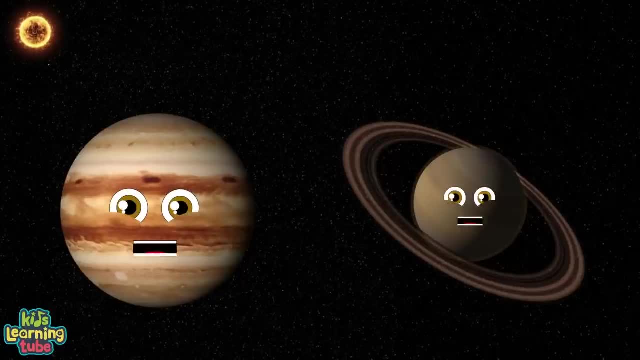 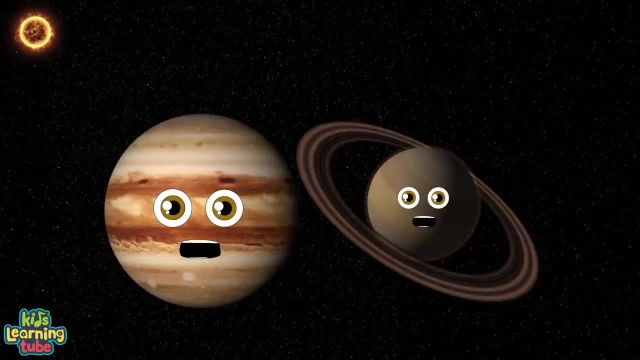 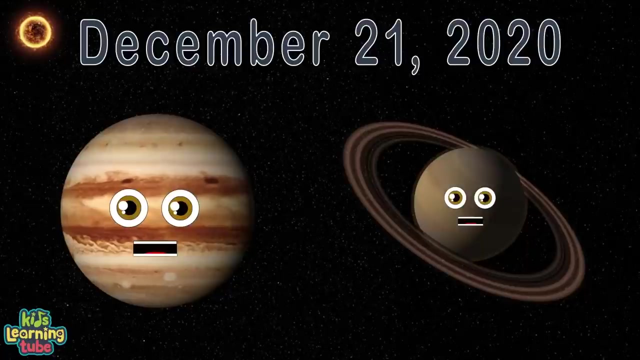 Look to the night sky to see this event. The joy it'll bring is plenty. Jupiter and Saturn will come within 0.1 degrees of each other, Forming the first visible double planet in 800 years will clutter On the winter solstice, December 21st in 2020. Look to the night sky to see this event. 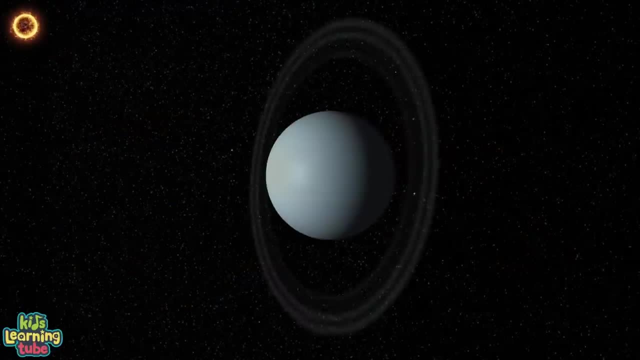 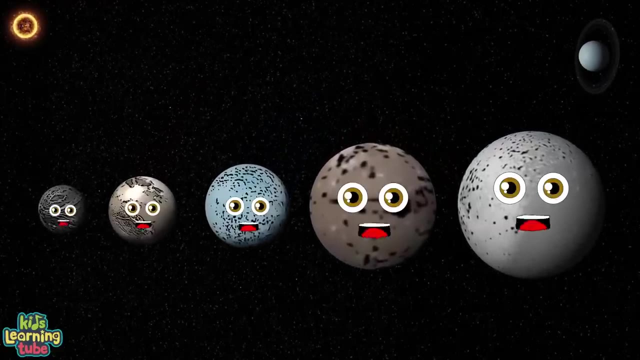 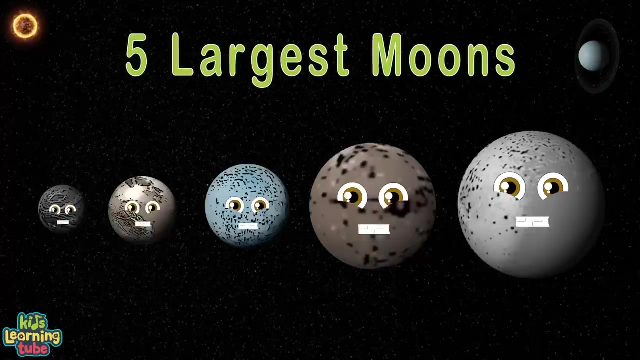 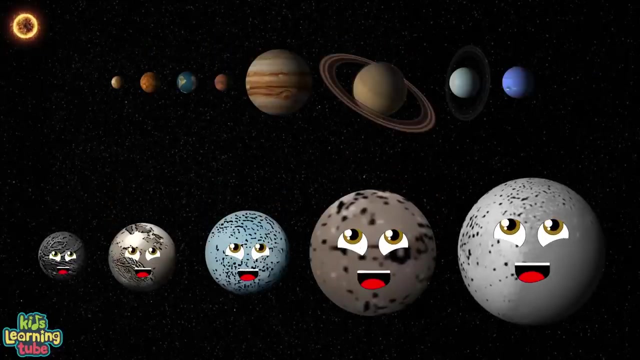 The joy it'll bring is plenty. There are 27 moons of planet Uranus. We're the 5 largest moons. The smallest, two largest. we trust We're the 5 largest moons of planet Uranus, The 7th planet in the solar system. let's not rush. 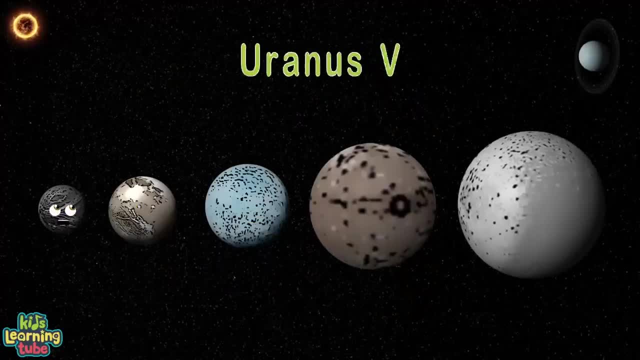 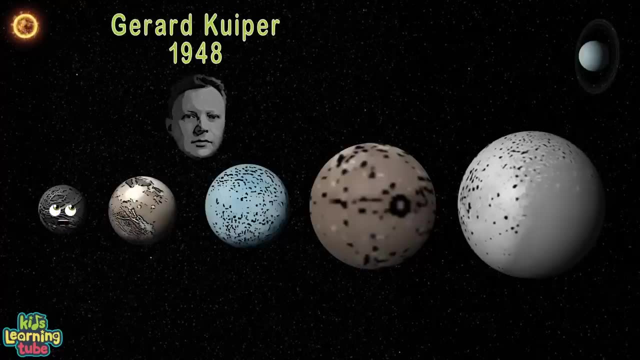 I am Miranda, also designated Uranus 5 And the smallest of the innermost 5 round satellites. I was discovered by Gerard Kuiper in 1948 At the McDonald Observatory. it must have been fate. I'm Ariel, I rotate, I fly. 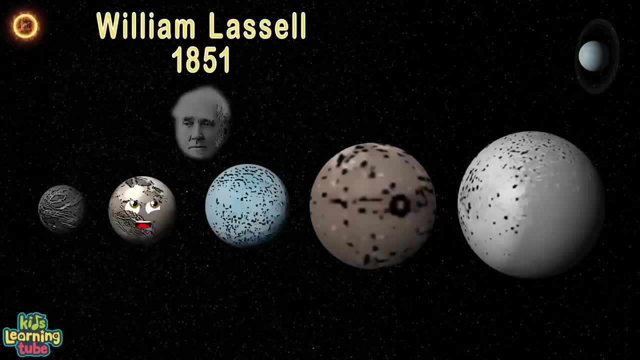 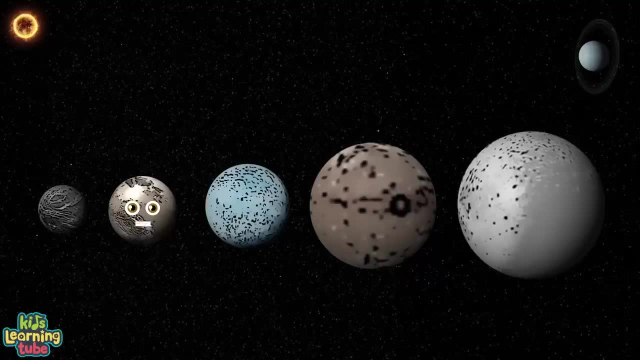 On Uranus's equatorial plate, Discovered in 1851 by William Lasso. as I explain, I'm the 4th largest of Uranus's 27 moons. Maybe someday you'll become an astronomer, So I will see you soon. I'm Umbriel, discovered at the same time as Ariel. 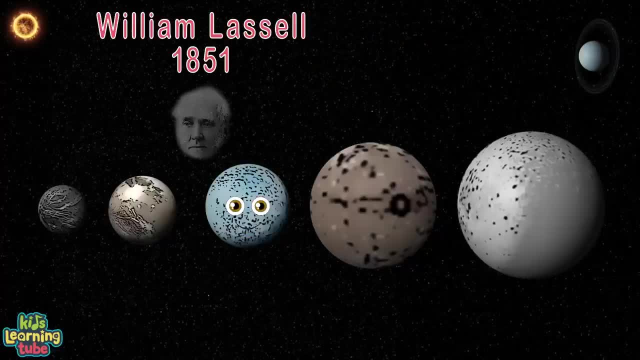 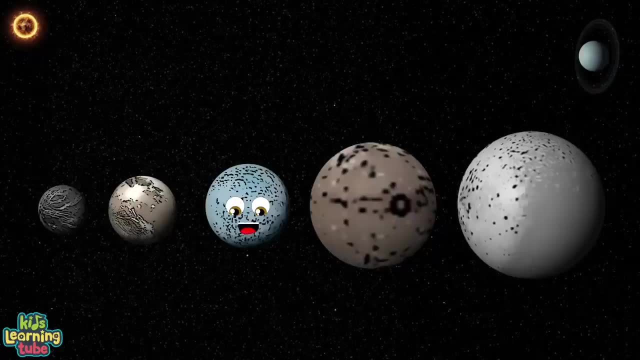 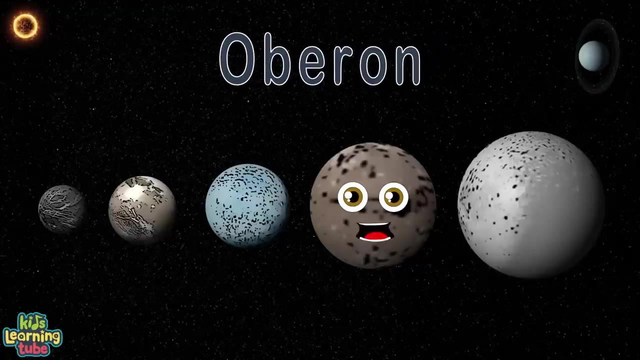 By the famous astronomer William Lasso. My surface is the darkest among Uranian moons. I have a lot of space. I have a lot of impact craters. I hope to see more soon. I am the Oberon moon, also called Uranus 4. I'm the outermost major moon of Uranus. that's 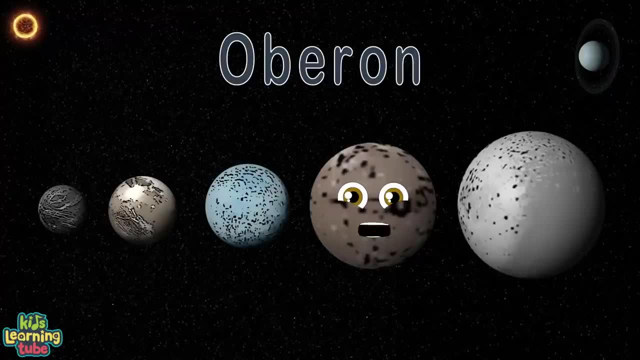 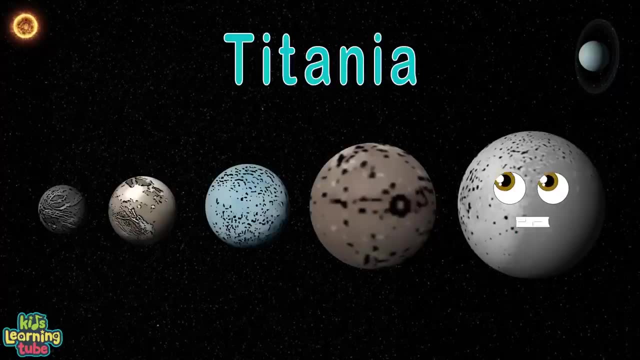 for sure. I'm the 2nd largest and 2nd most massive of Uranian moons. With a size like mine, to see me is opportune. My name's Titania, designated Uranus 3, The largest of Uranian moons and 8th in the. 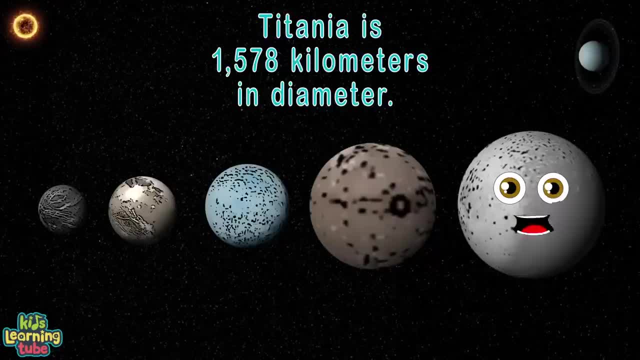 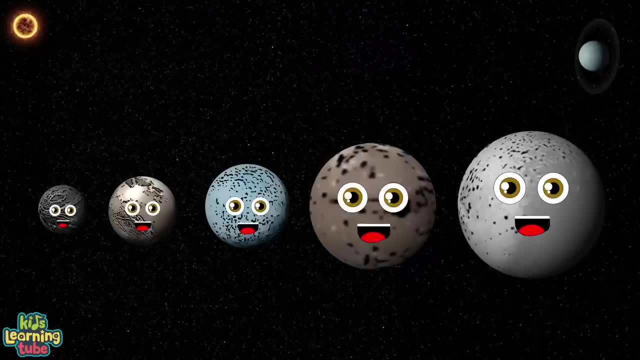 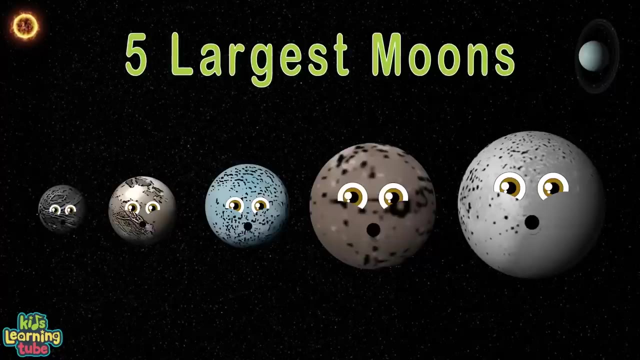 solar system. see 1578 km in IB diameter. In 1787 Williamerschild discovered me. There are 27 moons of Planet Uranus. We're the 5 largest moons, Smallest to largest. we trust We're the 5 largest moons of. 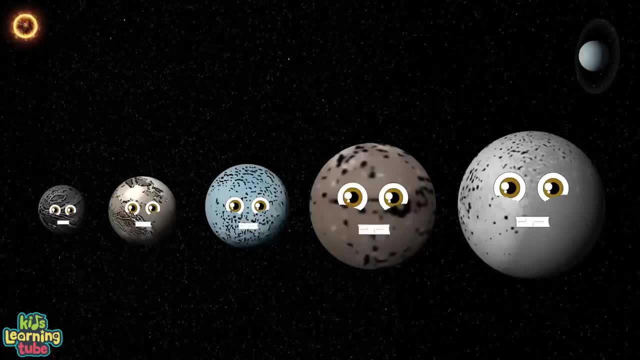 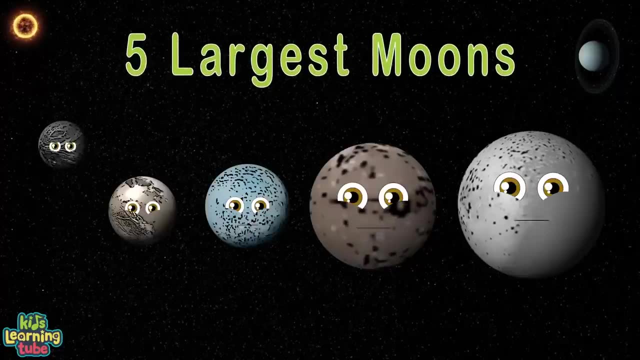 Planet Uranus, The 7th planet in the solar system. Let's not rush. There are 27 moons of Planet Uranus With a large outer crust. Planet Uranus: we're the five largest moons, smallest to largest. we trust we're the five. 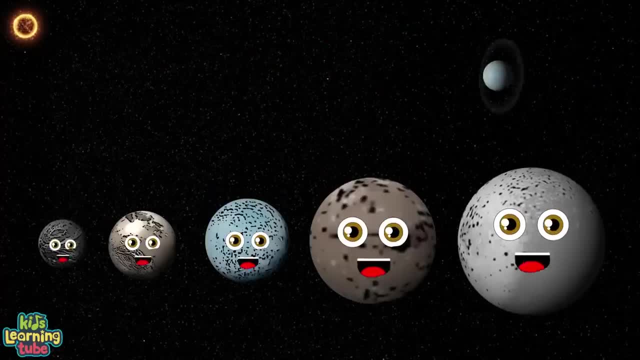 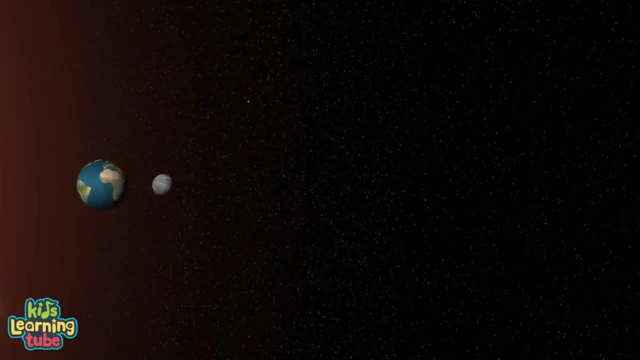 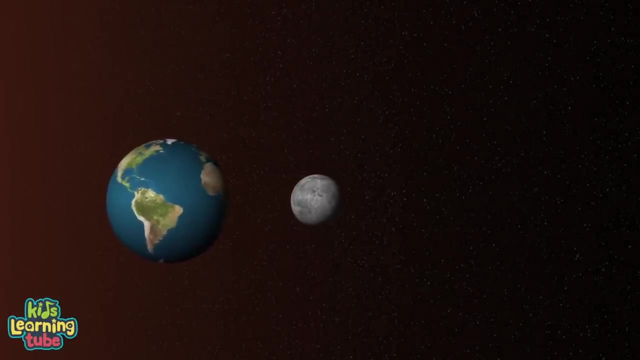 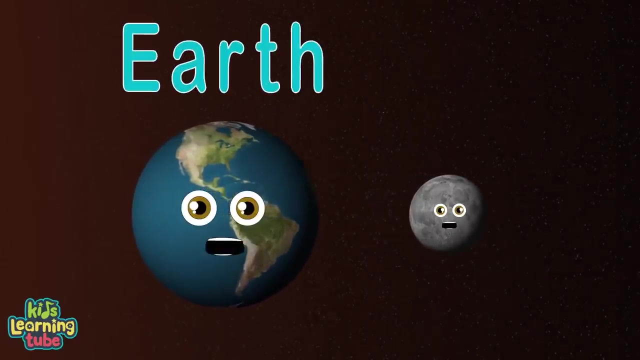 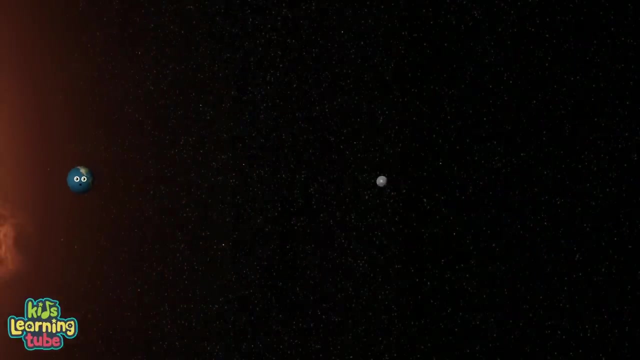 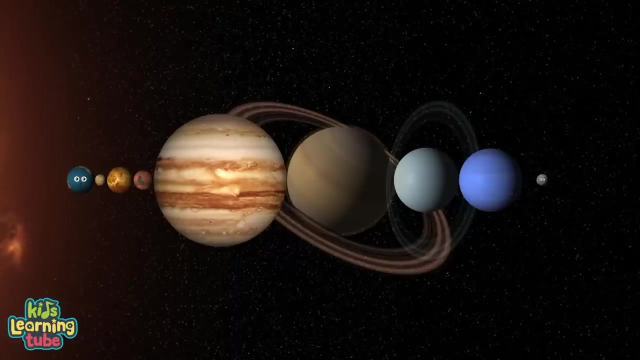 largest moons of Planet Uranus, the seventh planet in the solar system. let's not rush. We are the Earth and the Moon and you will learn really soon. you can fit the planets in our solar system between us. this is true. we are the Earth and the Moon. we meant to. 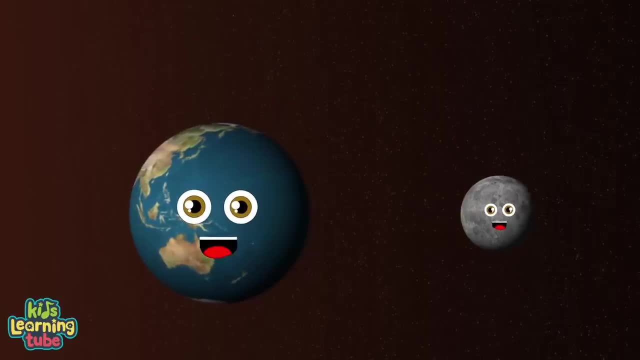 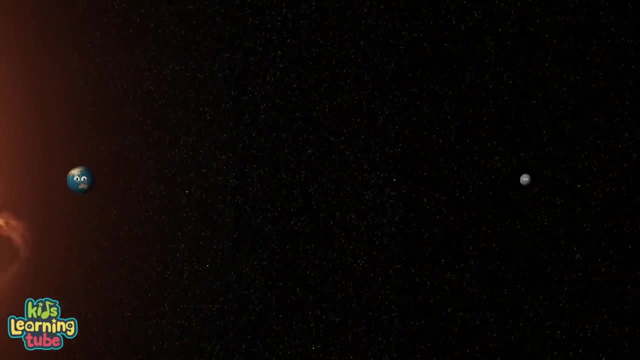 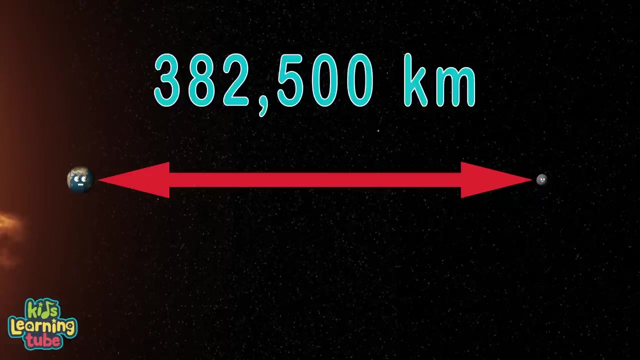 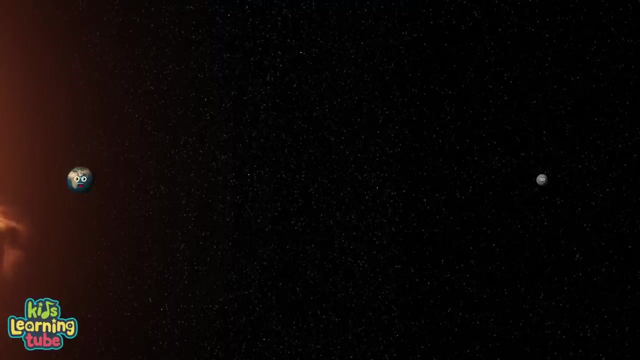 tell you for a while the average distance between us. we will explain to you With a smile. the average distance between the Earth and the Moon is 382,500 kilometers. here's the other seven planets fit between us, explaining who they are with some cool. 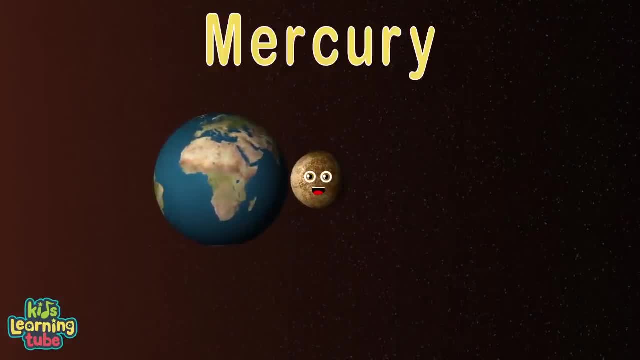 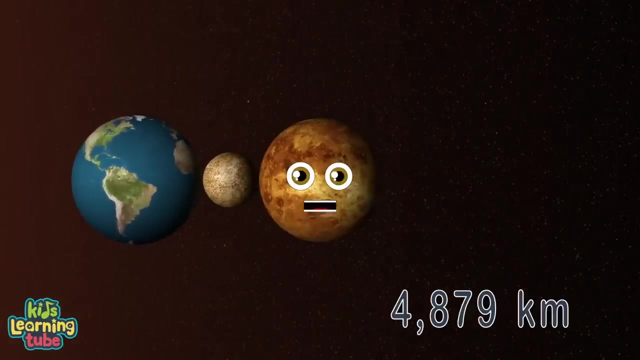 features. I am Mercury, the first planet from the Sun. I'm the second oddest planet on my run. my average diameter, we do know, is 42.. 40.. 4,879 kilometers. add these up as they are shown. I am Venus, the hottest planet, and 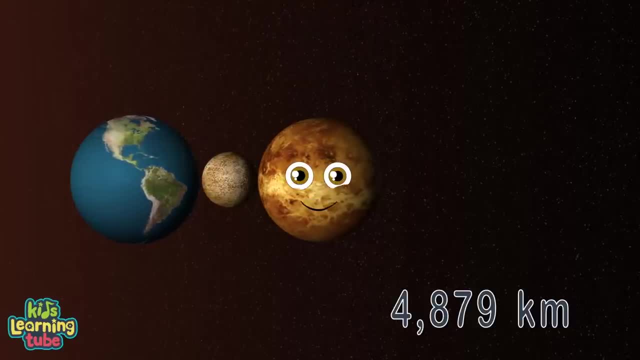 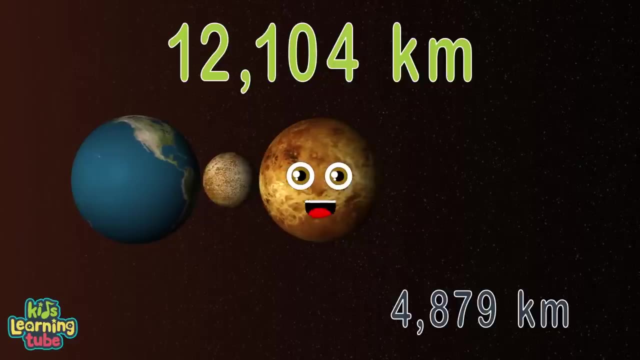 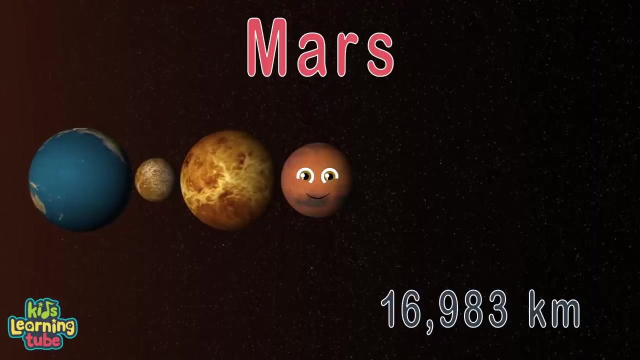 the second from the Sun. I have an average diameter of 12,104 kilometers in the solar system. hi, I am Mars, the fourth planet from the Sun. you should know I have an average diameter of 12,104 kilometers. add these up as they are shown. I am Venus, the hottest. 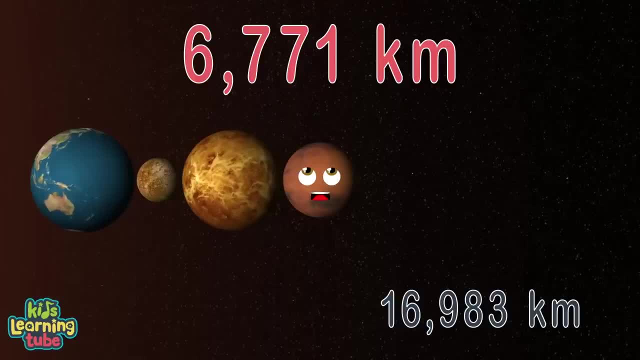 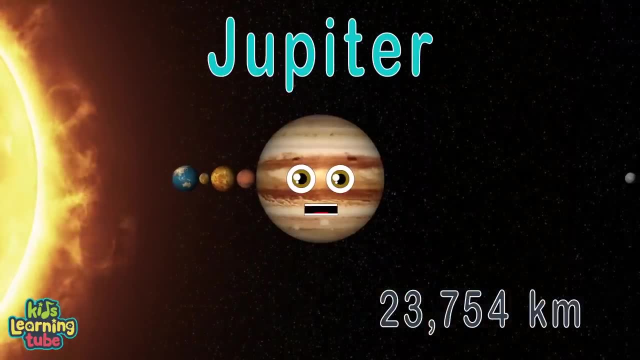 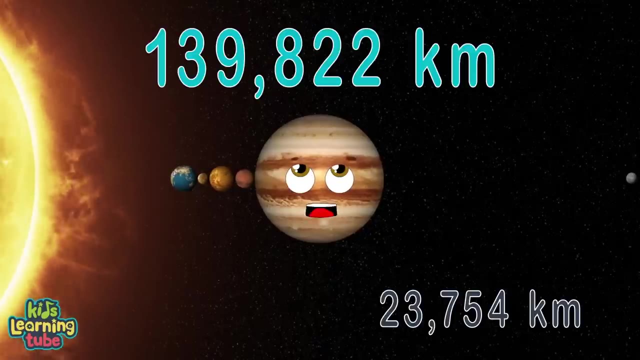 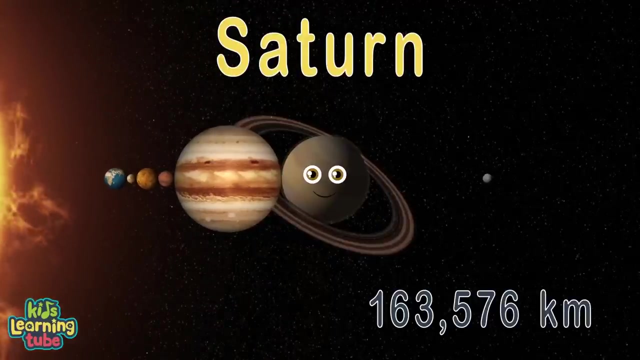 planet from the Sun. you should know, I have an average diameter of 6,771 kilometers. as I did show, my name is Jupiter, the largest planet, and from the Sun, I'm number 5,. my average diameter is 139,822 kilometers. as I thrive, I'm the planet with the prominent. 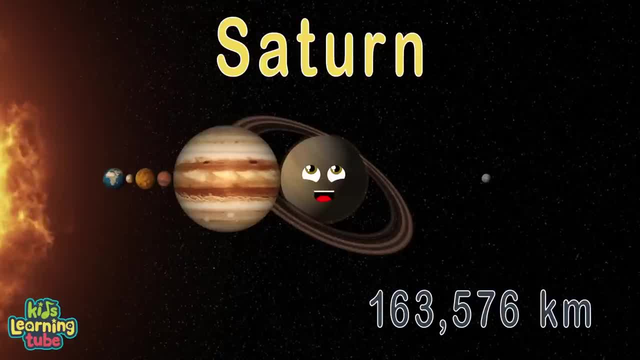 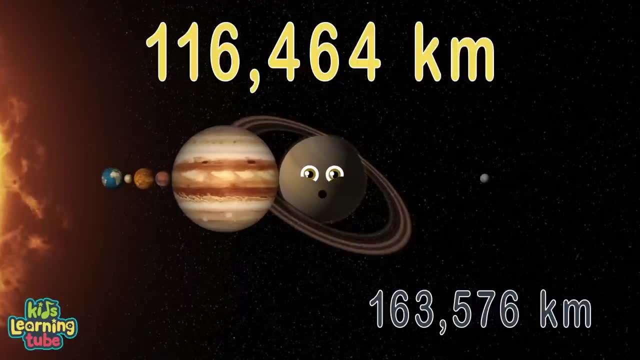 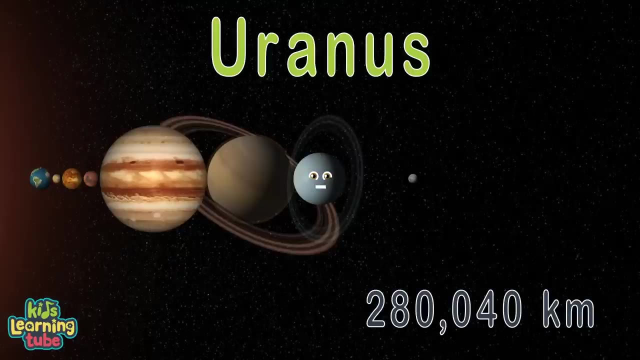 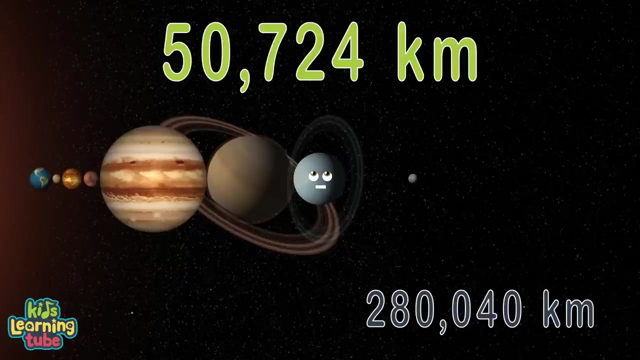 rings. the sixth one called Saturn. My average diameter is 116,464 kilometers. while I turn, I am Uranus. I am the seventh planet from the solar system's Sun. I have an average diameter of 50,724 kilometers. I'm. 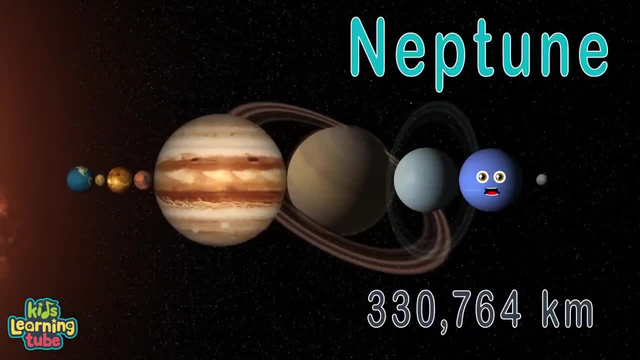 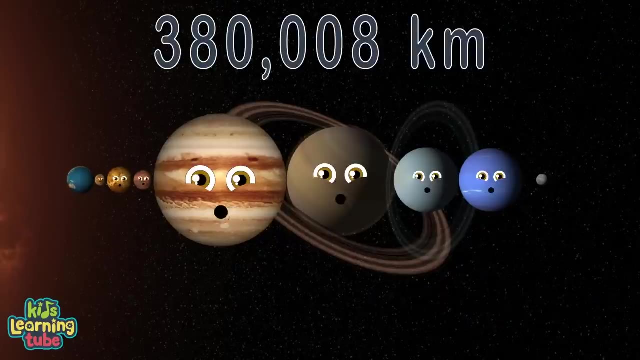 a frozen one. I am Neptune, the eighth and last planet in the solar system's Sun. I have an average diameter of 12,104 kilometers. as far as we know, I have an average diameter of 49,244 kilometers. I'm blue, as shown our total planet diameter size when added up. 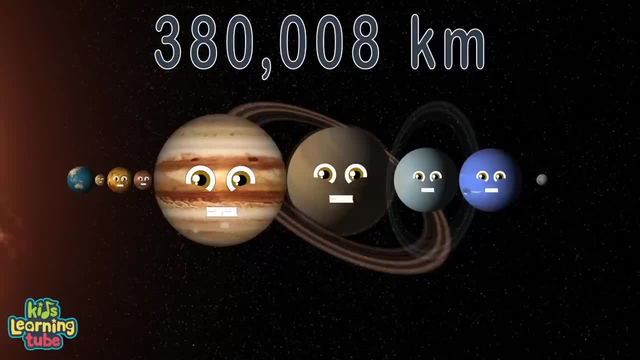 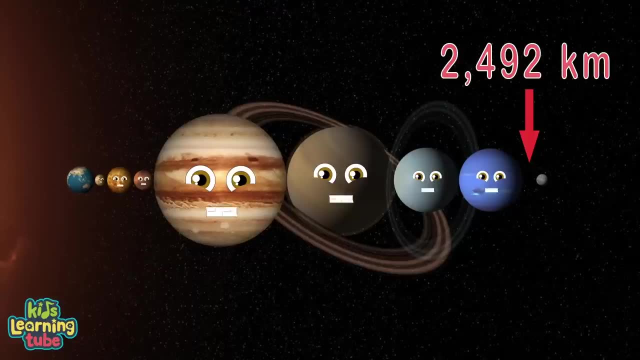 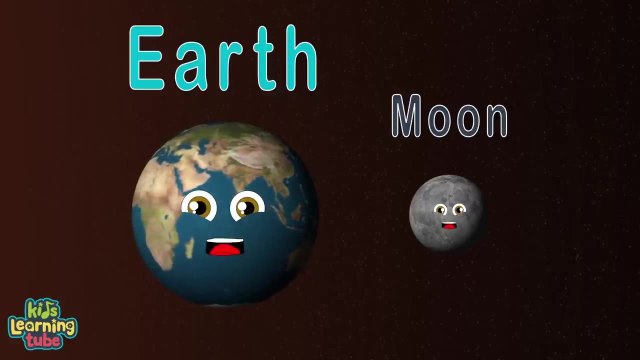 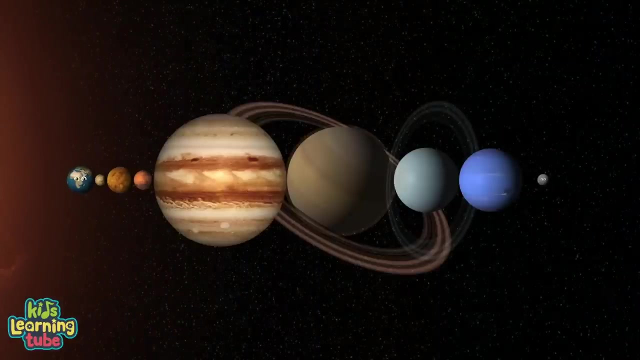 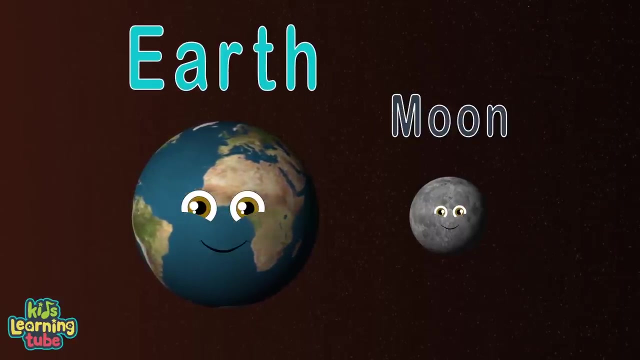 is 380,008 kilometers we share. we still have 2,492 kilometers of space to spare. we are the Earth and the Moon And you will learn really soon. you can fit the planets in our solar system between us. this is true. we are the Earth and the Moon. we meant to tell you for a while the 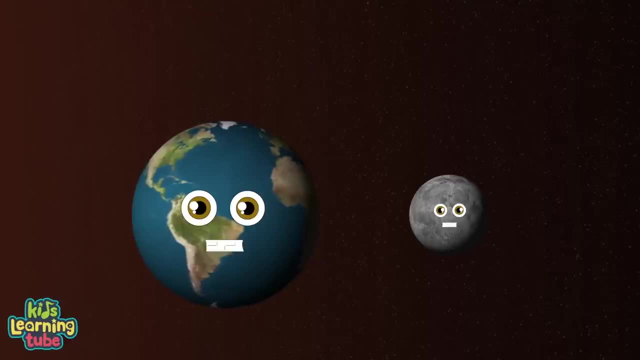 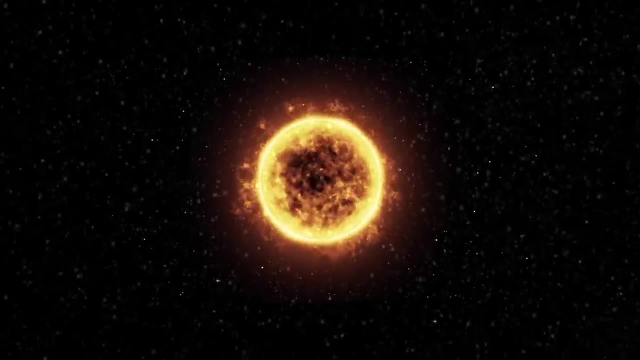 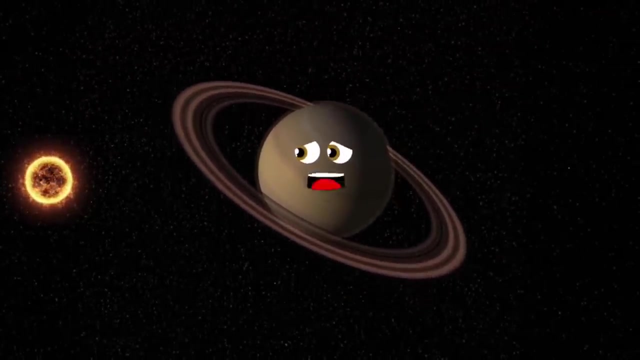 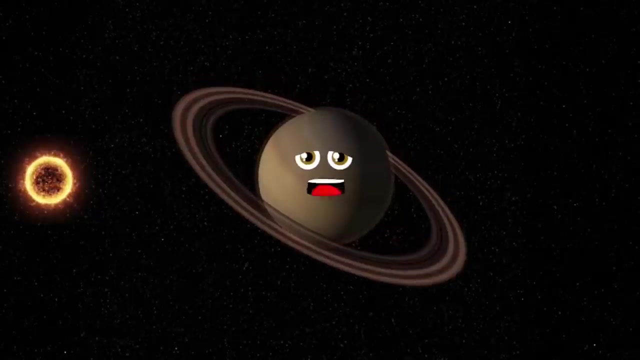 average distance between us. we will explain to you with a smile. I am Saturn, the sixth planet from the sun. I'm known for my rings by everyone. I'm the second largest planet in our solar system. Please come sing along until my teachings are done. 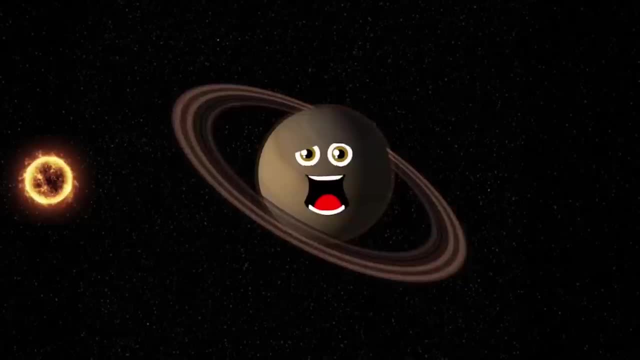 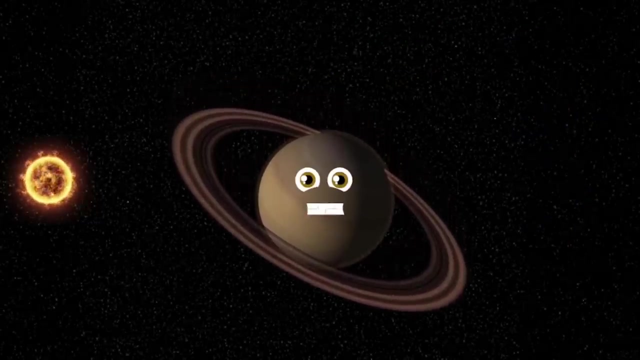 Out of my 62 moons, 53 are named. I am a gas giant. all astronomers claim 36,184 is my radius in miles for you to explore. 10.44 meters that's per second you drop. That's my gravity pulling towards my surface top. 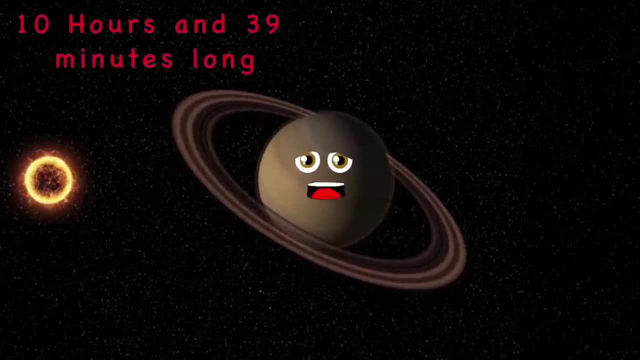 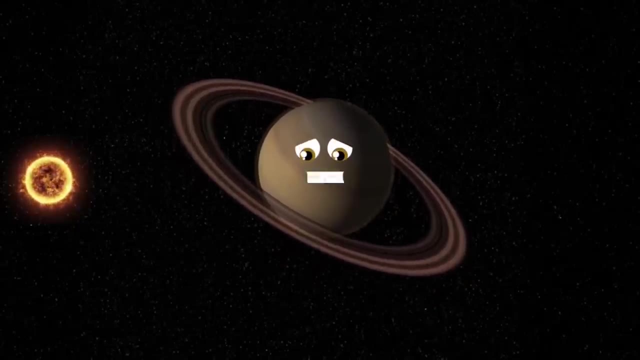 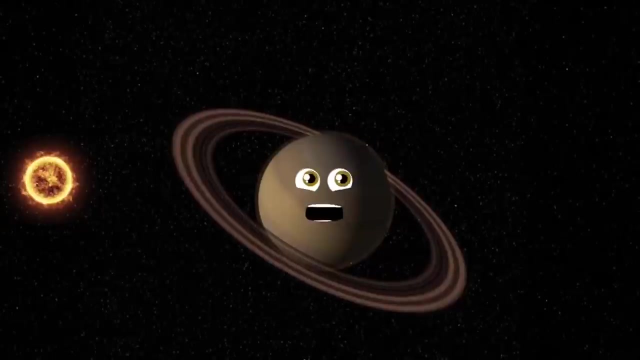 10 hours and 39 minutes long is the day on my surface. let's sing this song. I am Saturn, the sixth planet from the sun. I'm known for my rings by everyone. I'm the second largest planet in our solar system. Please come sing along until my teachings are done. 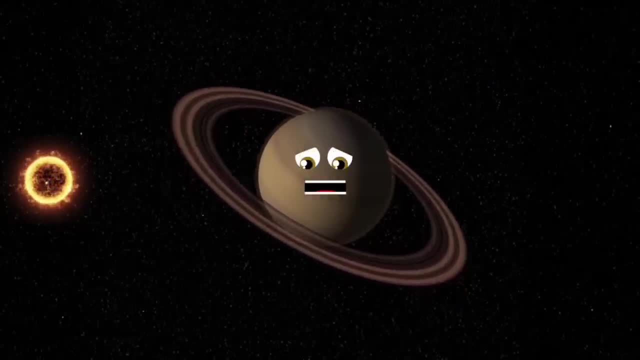 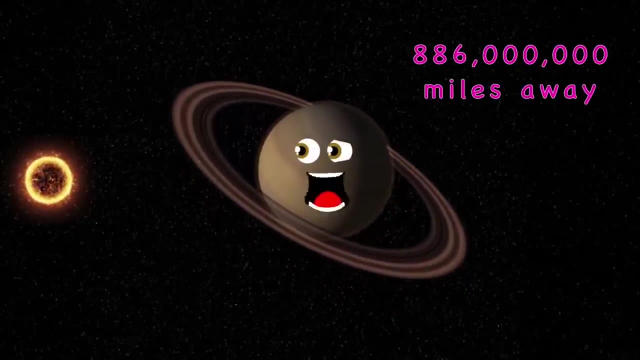 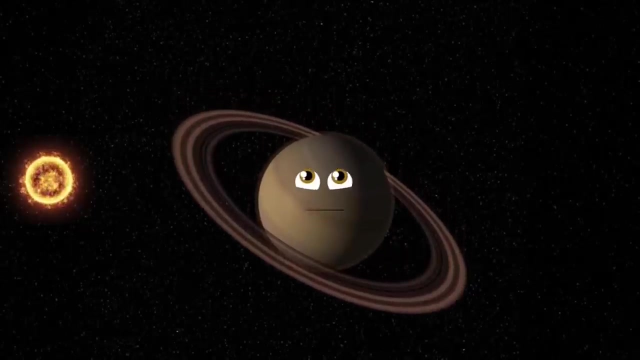 Takes 29 years for me to orbit the sun, And my rings are made up of rock and icy chunks. 886 million miles away is my distance from the sun. that is why I'm Chile. Hydrogen and helium are what I'm mostly made of, And my atmosphere from the surface above. 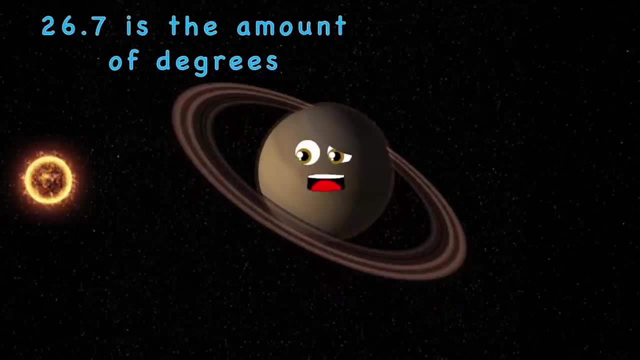 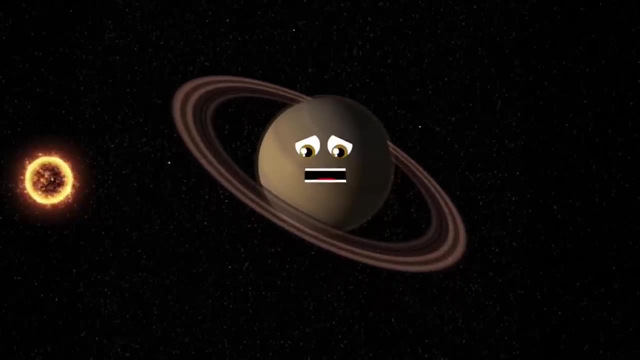 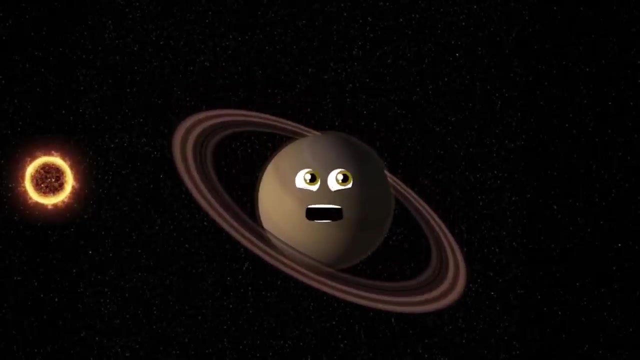 26.7 is the amount of degrees I spend on my axis. I'm so cold that you freeze. I am Saturn, the sixth planet from the sun. I'm known for my rings by everyone. I'm the second largest planet in our solar system. Please come sing along until my teachings are done. 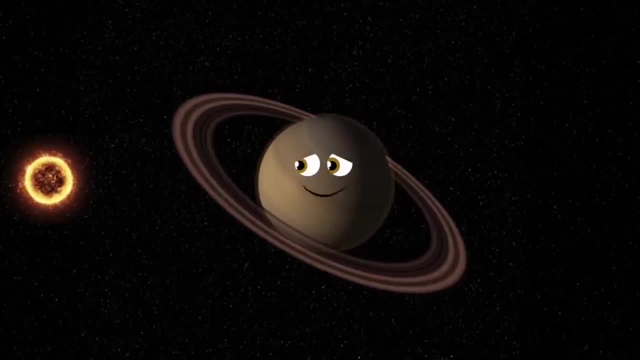 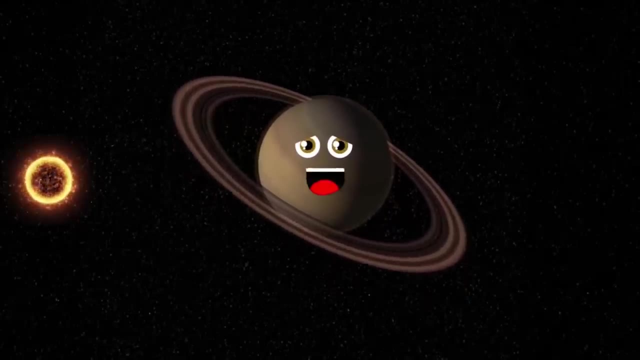 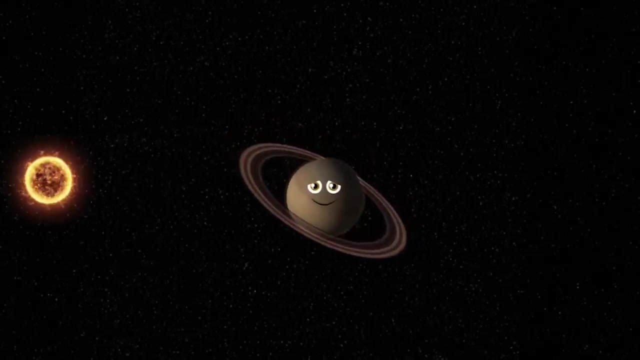 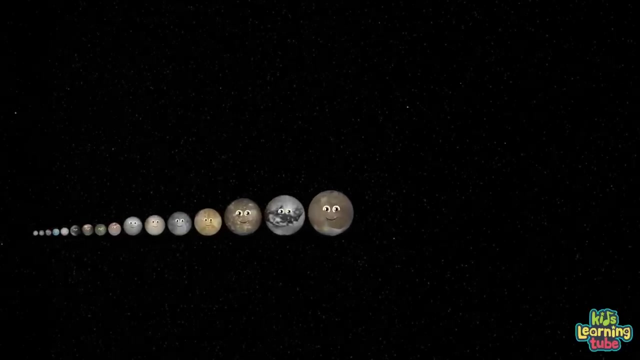 I am Saturn, the sixth planet from the sun. I'm known for my rings by everyone. I'm the second largest planet in our solar system. Please come sing along until my teachings are done. Here's a moon-sized comparison in our solar system. Here's a moon-sized comparison in our solar system. 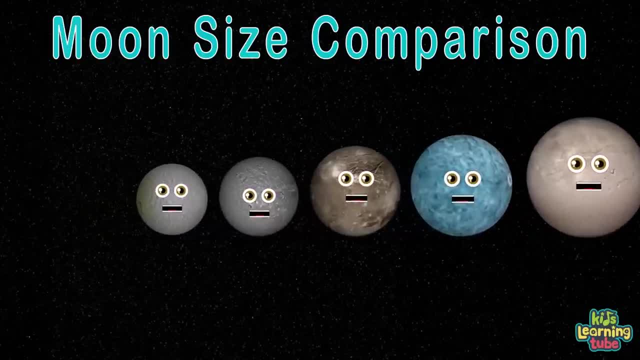 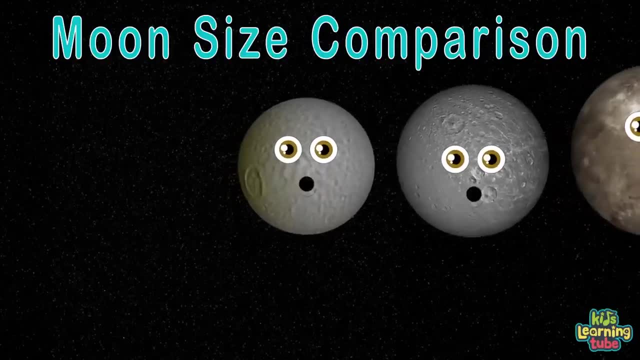 We're happy to be a part of a community. We're happy to be a part of a community. If you'd shed some light on us. until we are done. We're measured by our radius. you'll hear in a bit. We'll also tell you the planet in which we orbit. 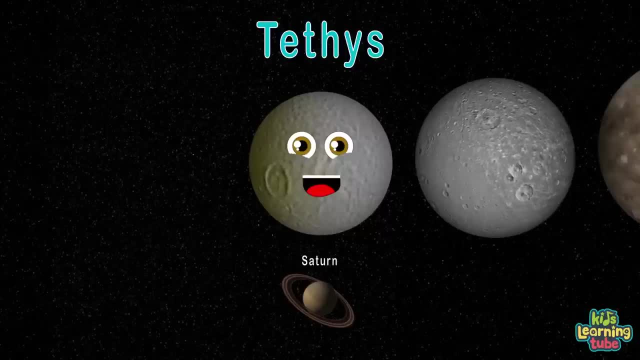 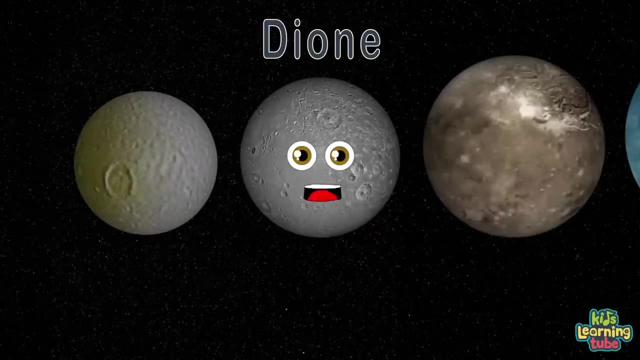 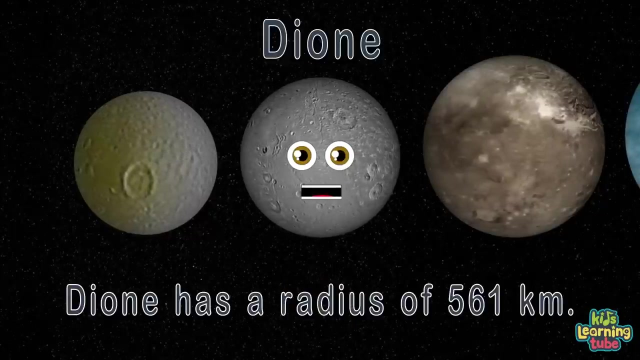 My name is Tethys. I'm one of Saturn's 82 moons. My radius is 531 kilometers. it is true, I am Dion. I orbit Saturn. you do see, My radius is 561 kilometers. that is me. Ariel is my name. Uranus is what I orbit. 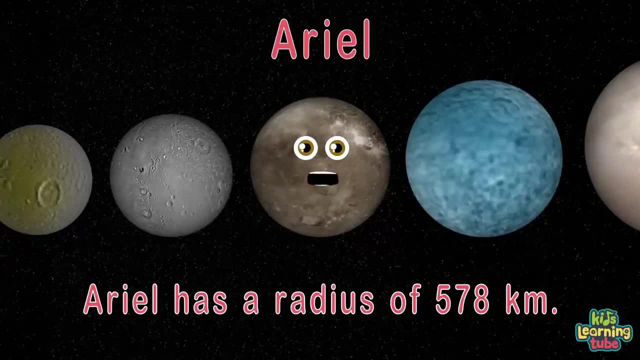 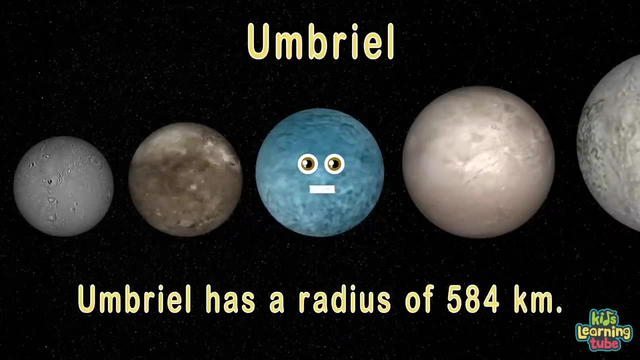 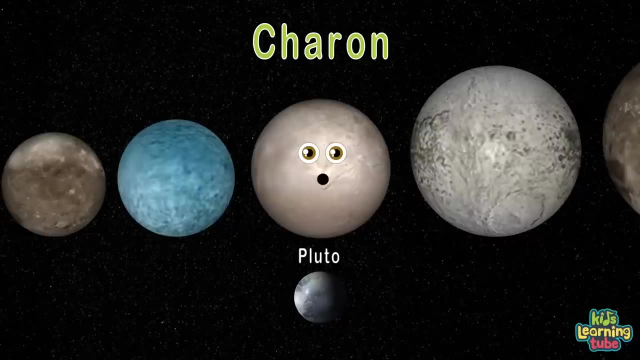 My radius is 578 kilometers. I'm third on the list. Hi, I'm Umbrio. Uranus is where I'm from. My radius is 584 kilometers. I am spun. I'm the moon of Charon. I float in orbit. Pluto Radius is 606 kilometers. this I do know. 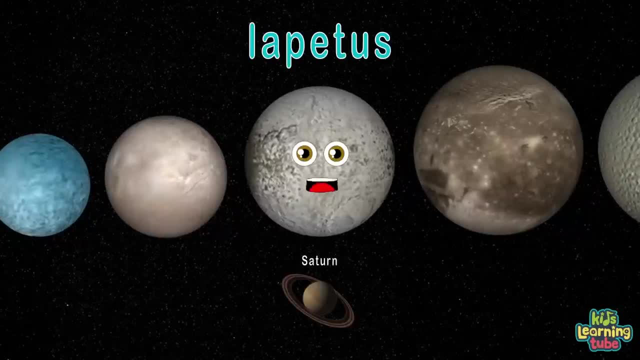 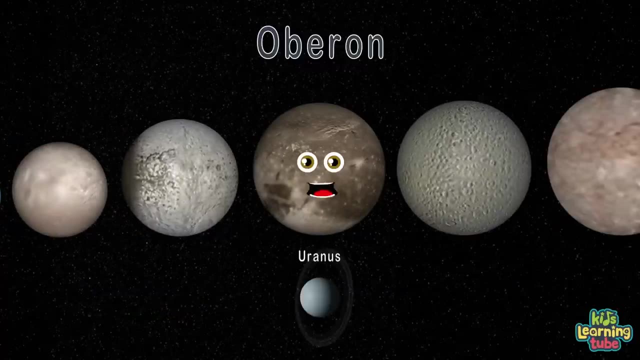 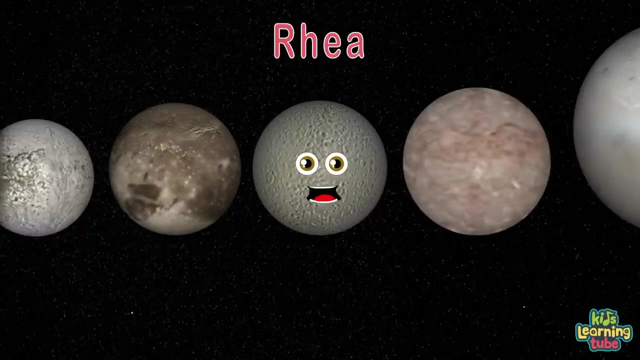 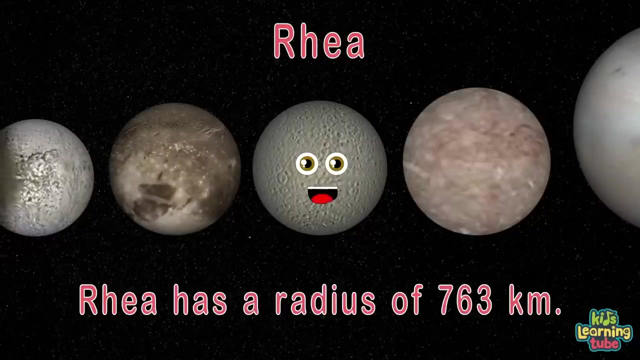 I'm Iapetus, a moon of Saturn, Radius of 734 kilometers. as I turn, Oberon is my name. outermost moon of Uranus. 761 kilometers is my radius. I am Rhea, Saturn's second largest moon, Radius of 763 kilometers. see you soon. 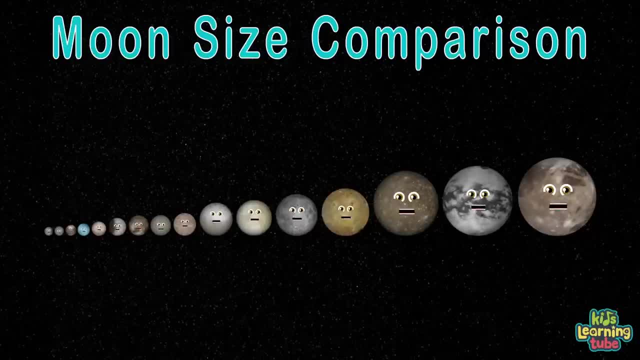 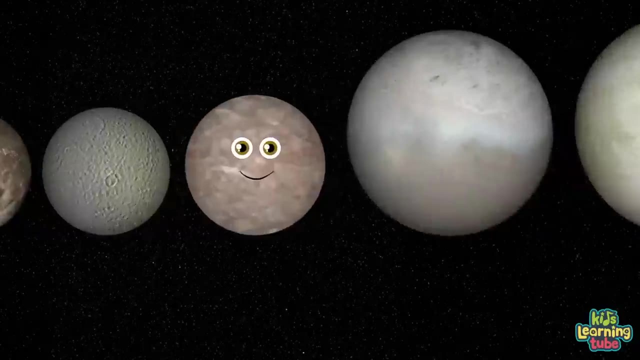 Here's a moon-sized comparison in our solar system. We're happy if you'd shed some light on us Until we are done. We're measured by our radius. you'll hear in a bit. We'll also tell you the planet in which we orbit. I'm Titania, the largest moon of Uranus. 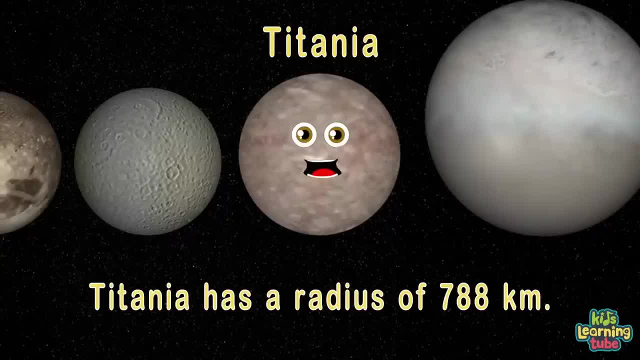 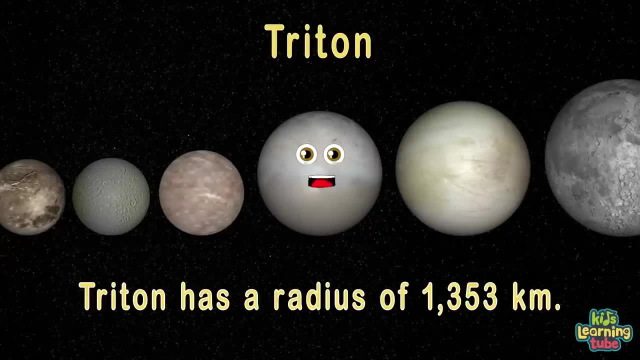 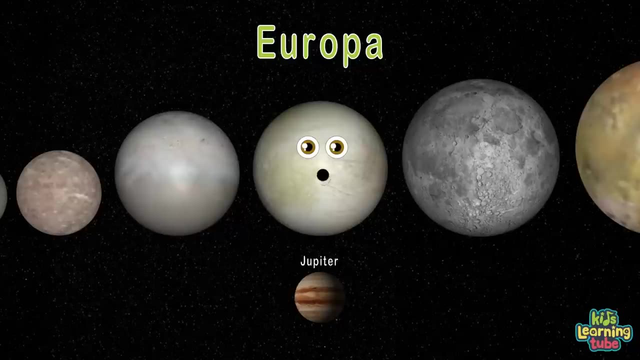 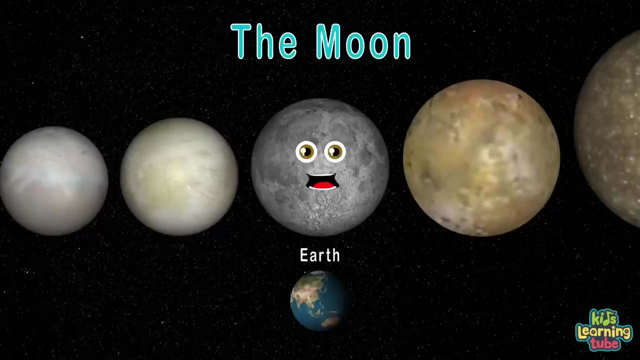 788 kilometers is my radius. The name is Triton, the largest moon of Neptune. I'm 1353 kilometers in radius. in this tune, Europa is frozen. I'm a moon of Neptune And a moon of Jupiter. My radius is 1560 kilometers. I am the moon of the planet Earth. 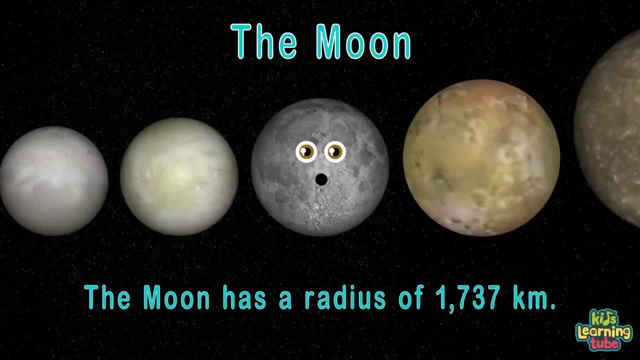 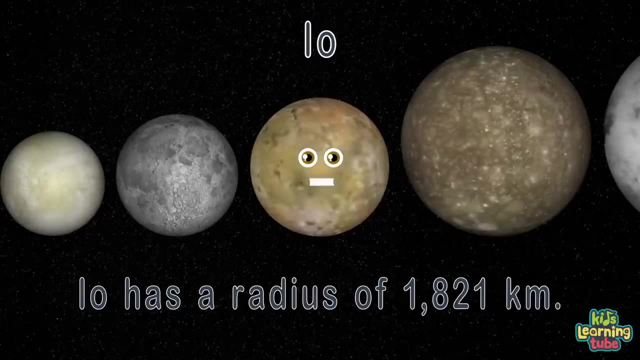 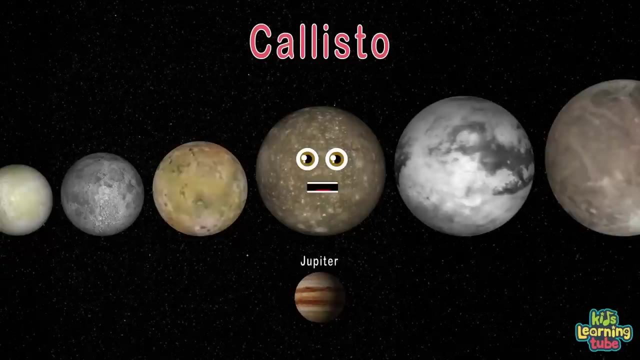 My radius is 1737 kilometers for what it's worth. Hello, I'm Io, the strangest moon of Jupiter With a radius of 1821 kilometers. I'm Callisto. I orbit Jupiter. you see, My radius is 2400 kilometers in radius. 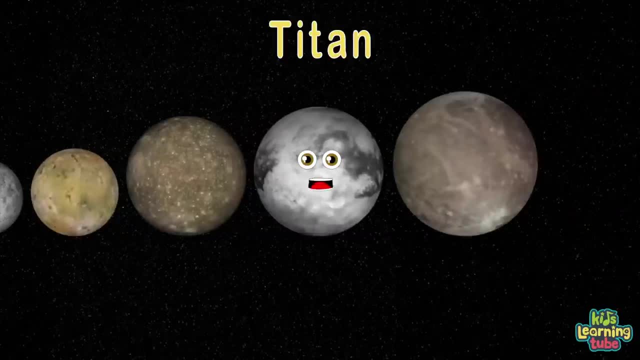 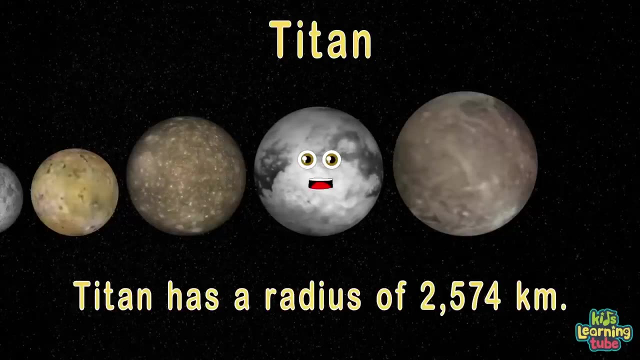 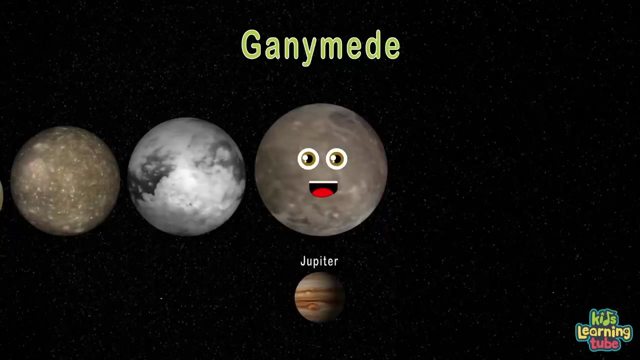 That's all on me. Titan is my name, Saturn's my claim to fame. 2574 kilometers is my radius. I claim I'm Ganymede, the largest moon in the solar system. Jupiter is what I orbit. yeah, that's where I'm from. 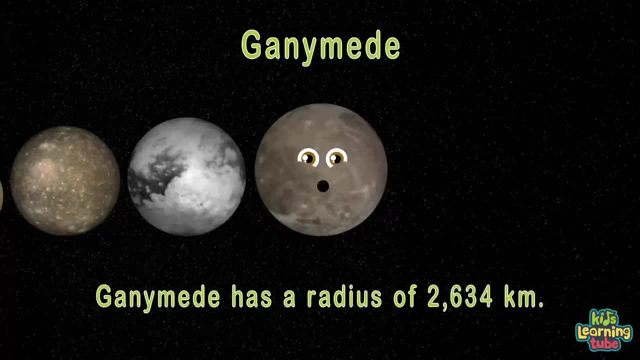 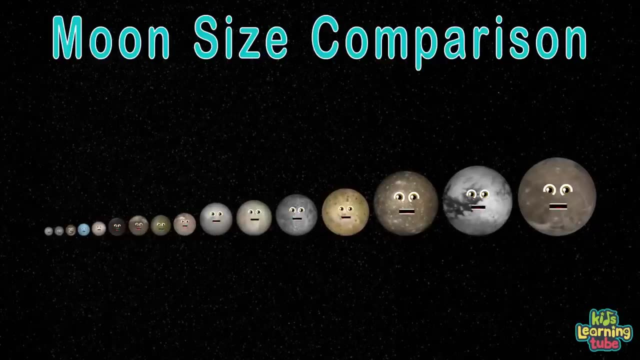 My radius is 2634 kilometers. Now let's listen to the chorus while the moons take a bow. Here's a moon-sized comparison in our solar system. We're happy if you'd shed some light on us. until we are done, We're measured by our radius. you'll hear in a bit. 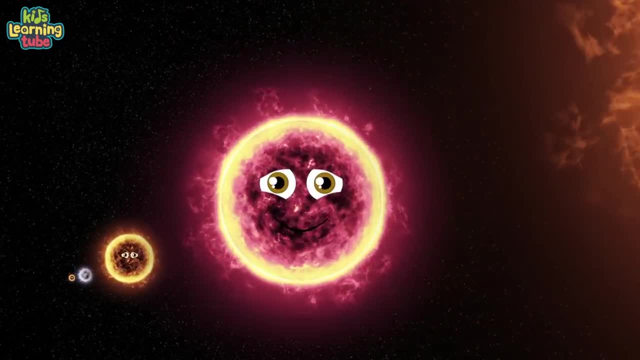 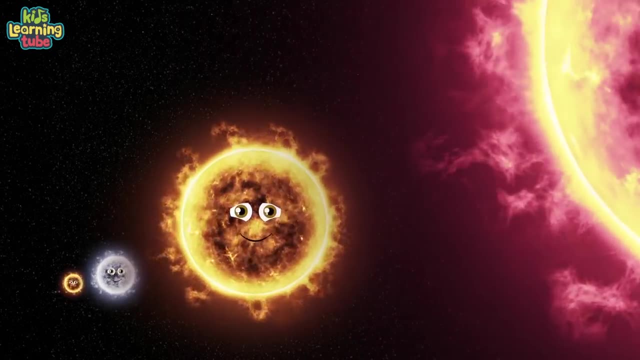 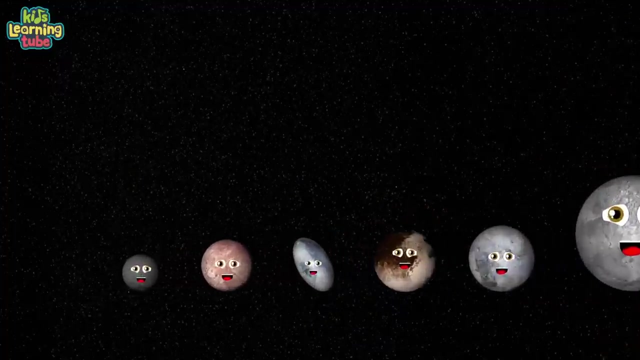 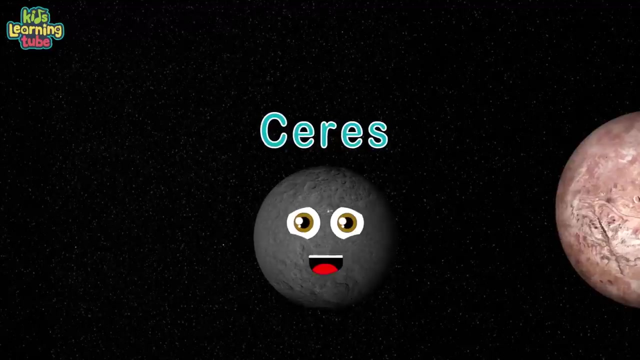 We'll also tell you the planet in which we orbit. This is a size comparison of objects in our universe. We'll start with the smallest And go to the largest, most well-known objects we know. of course, I am Ceres, I am a dwarf planet. 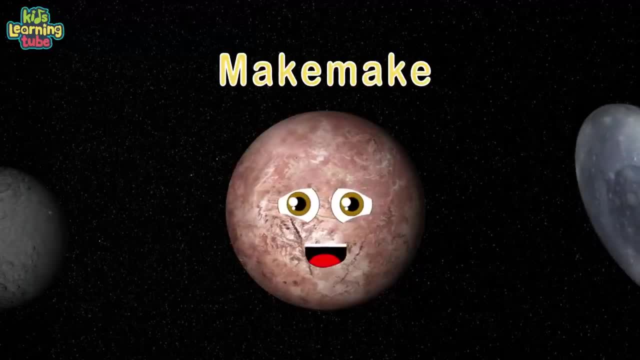 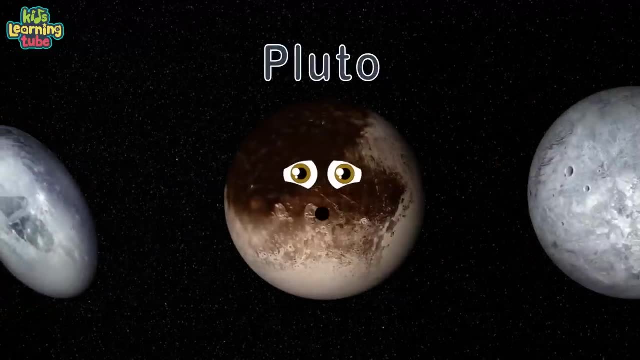 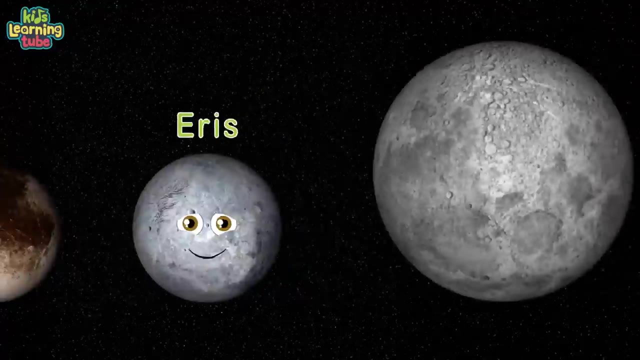 Maki. Maki's a dwarf planet as well, but didn't planet. I am Hamea, a dwarf planet in this group. Pluto is a dwarf, but used to be a planet, it's true. Aries is a dwarf planet in this mix. The Earth's moon is where your eyes are transfixed. 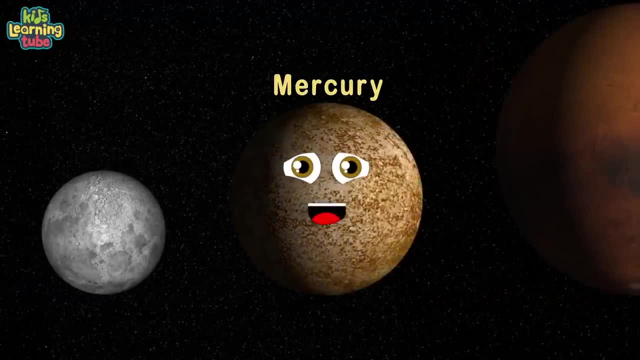 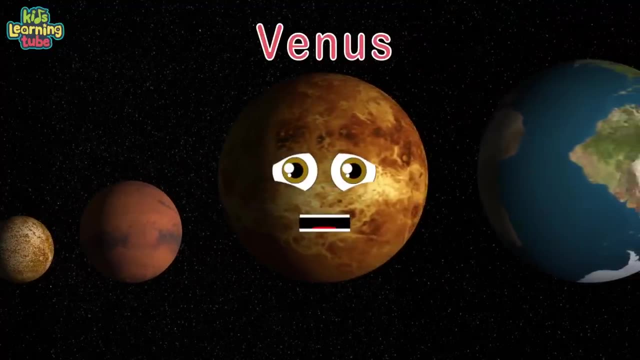 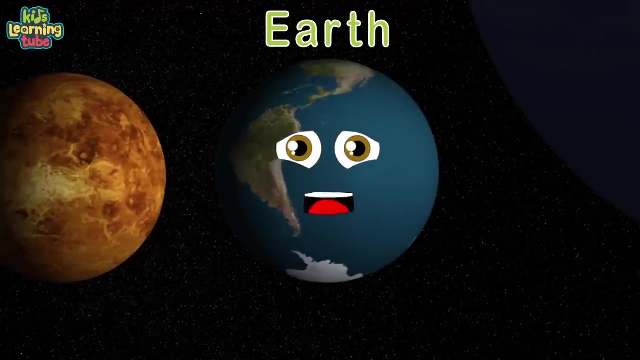 Mercury is here an official planet. I'm the planet of Mars. I'm sure you all know this. I'm planet Venus. my size, you may think, is large. Planet Earth is next and the humans think that they're in charge. Neptune's a planet in our solar system. wow. 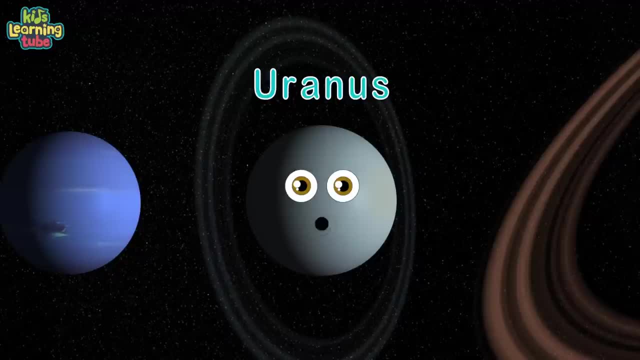 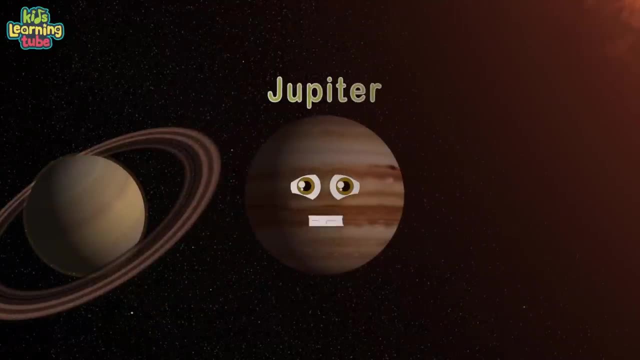 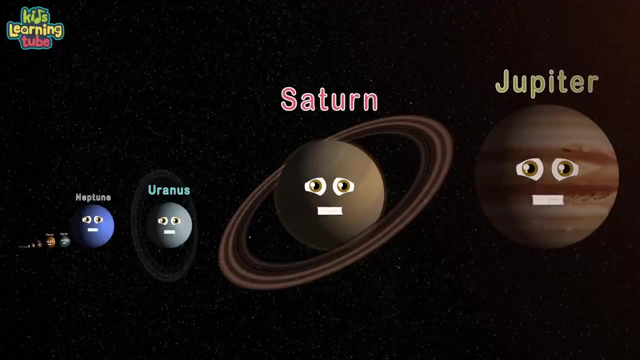 Planet Uranus is here. I wish I could take a bow. Planet Saturn has rings. if you think I am big, Check out planet Jupiter. I hope you can dig. This is a size comparison of objects in our universe. We'll start with the smallest and go to the largest most well-known objects. 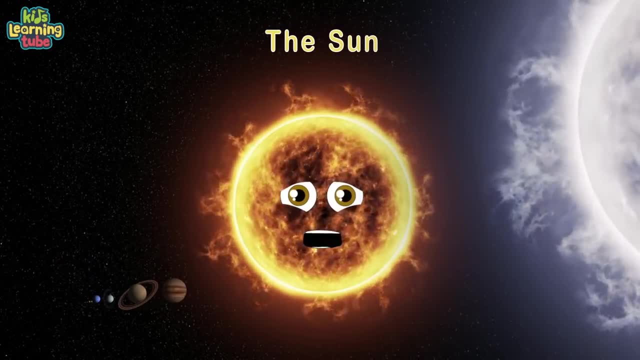 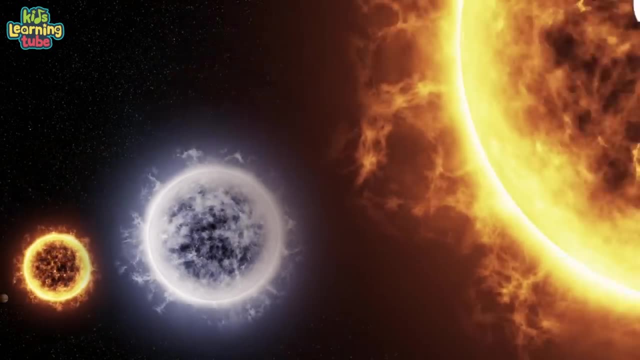 We know. of course I am Ceres. I am a dwarf planet. Of course I am the sun, a yellow dwarf, that isn't far. I am Sirius A, a main sequence star. My name is Pollux, a red giant star, it's true. 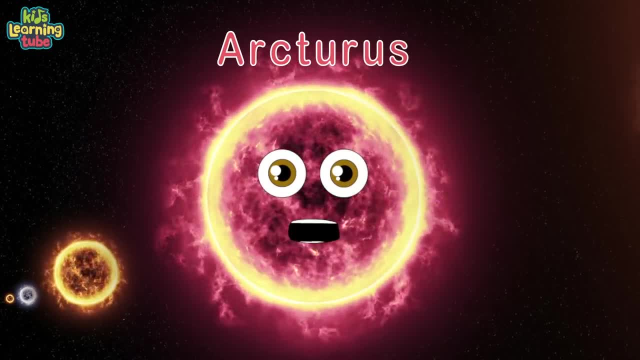 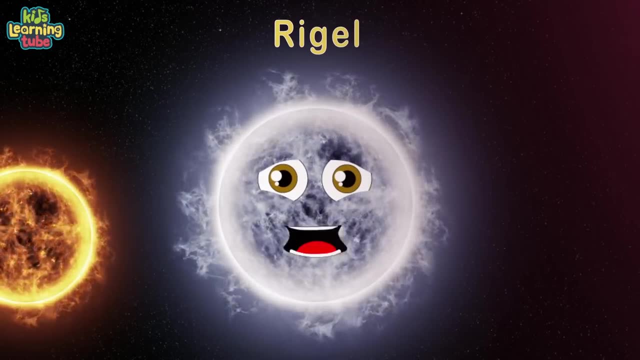 Arcturus is a red giant star. this I thought you knew. I'm Aldabra and a red giant star. that's me. Hi, I'm Rigel, a blue-white super giant. you see, I am Betelgeuse and I'm a red super giant. I'm in Tauris. I'm a red super giant that won't last. VY Canis Majoris, a red hyper giant star. I'm UY Scutai, the biggest red super giant this far. I am the Milky Way galaxy and you live in me. 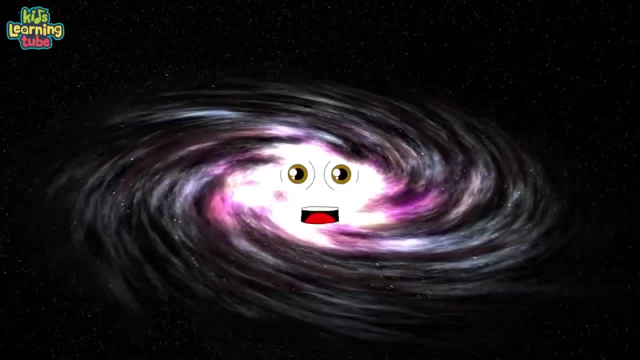 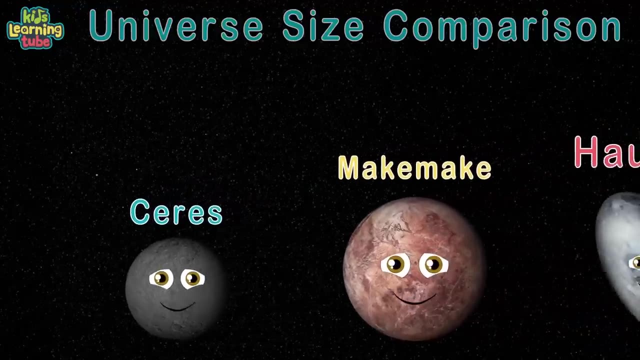 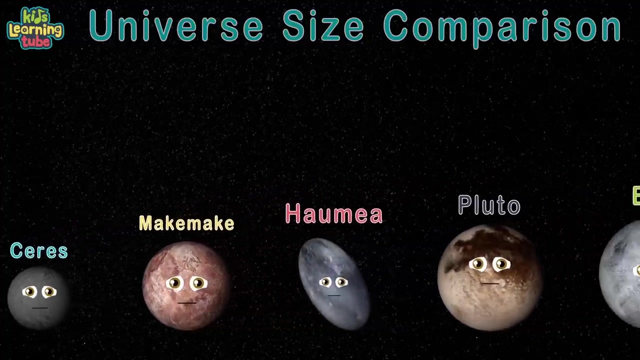 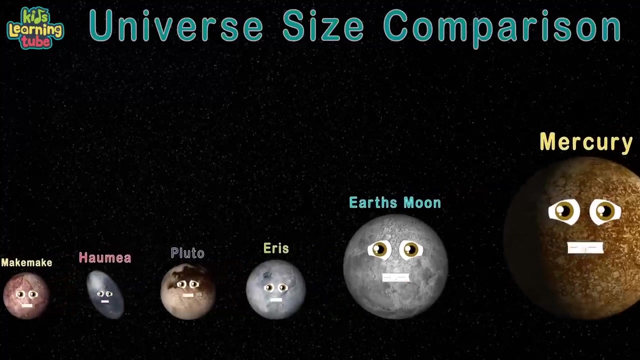 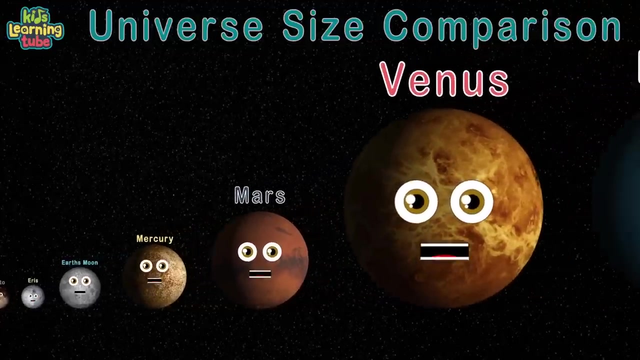 Now let's all sing the chorus together with glee. This is a size comparison of objects in our universe. We'll start with the smallest and go to the largest Most well-known objects we know. of course, This is a size comparison of objects in our universe. We'll start with the smallest and go to the largest. 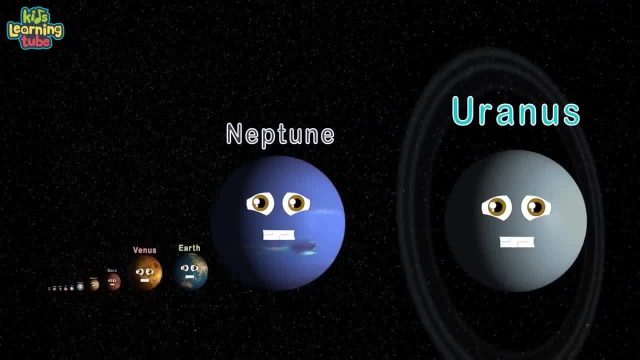 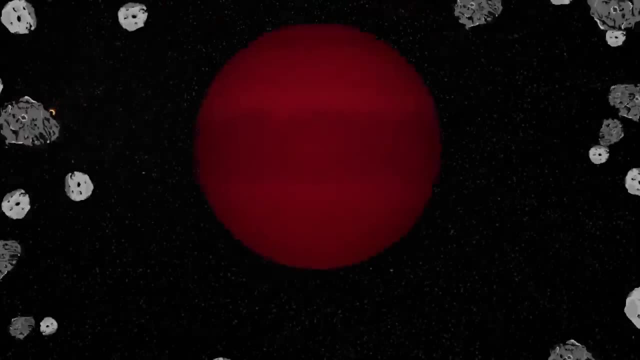 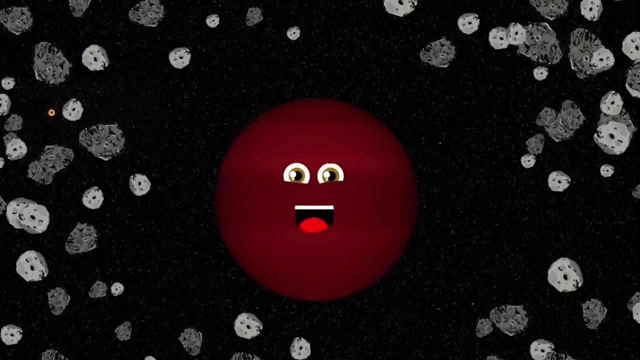 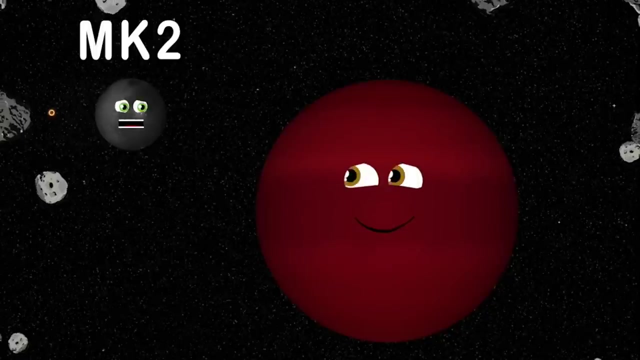 Most well-known objects. we know, of course, Most well-known objects in our universe. Most well-known object you're familiar with. Most well-known objects still, in effect, Most well-known objects in the gueney, Most well-known objects remind you of what it looks like. Most well-known objects are number zero. 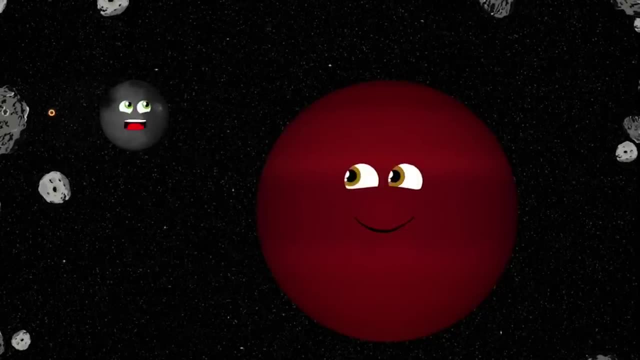 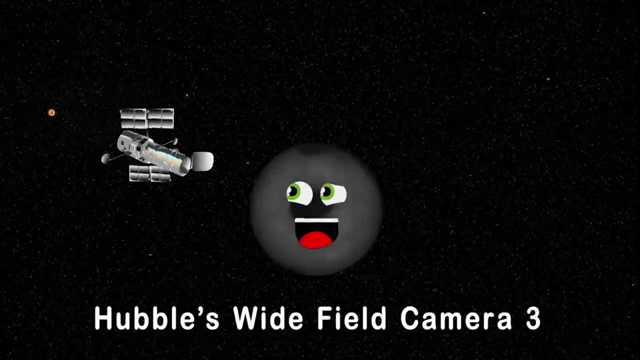 But most well-known objects, Bien Silence, Most well-known objects have a great homeownershub. That's why you're just a MARKIMOKE. Anyways, I ended into Hey nuclear star, Although I think the classes do have products on the list. Camera 3, the Southwest Research Institute led by Mark Bowie. 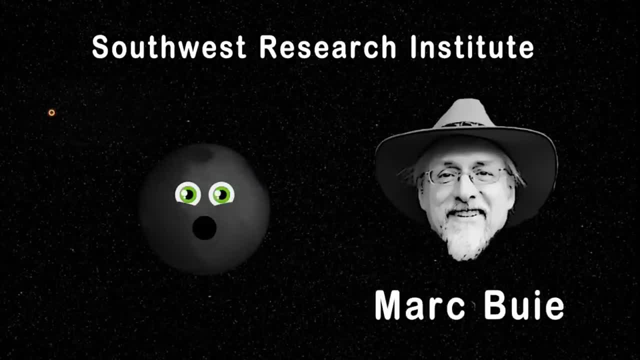 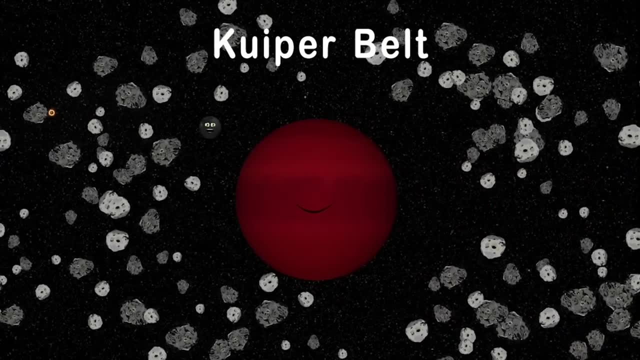 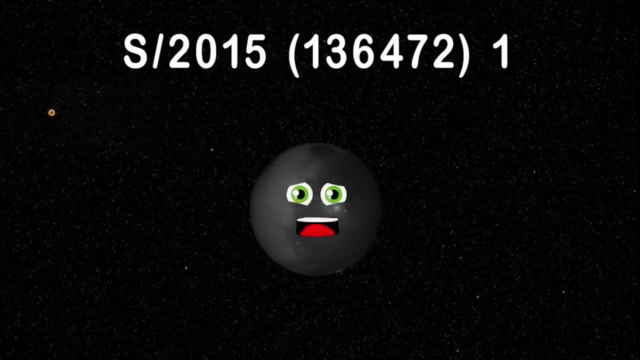 Are the first scientists in the world to ever notice me. I'm very hard to see because I'm in the Kuiper Belt And my charcoal-colored surface certainly doesn't help. As 2015,, 13,, 64,, 72,, 1 is what I was provisionally designated. 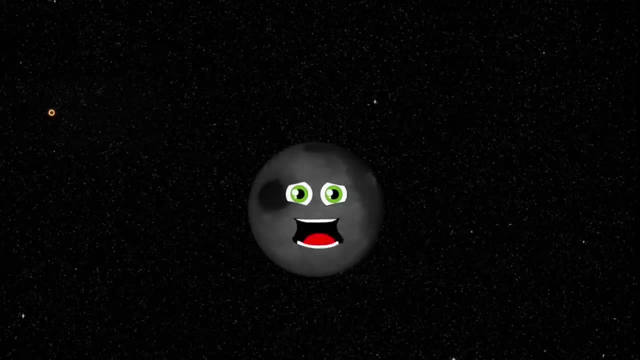 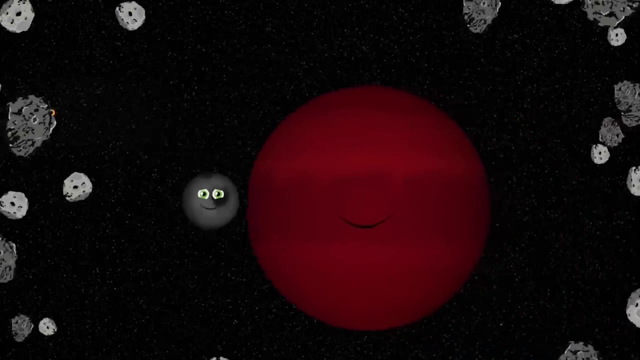 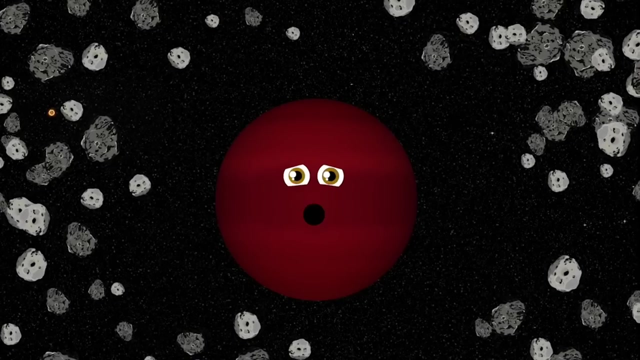 But not much fun. They officially nicknamed me with the name MK2. I'll tell you more about me after the chorus you'll hear is through. I'm Mikey. Mikey, I have an official new moon. Let me introduce MK2 to all the world and you. 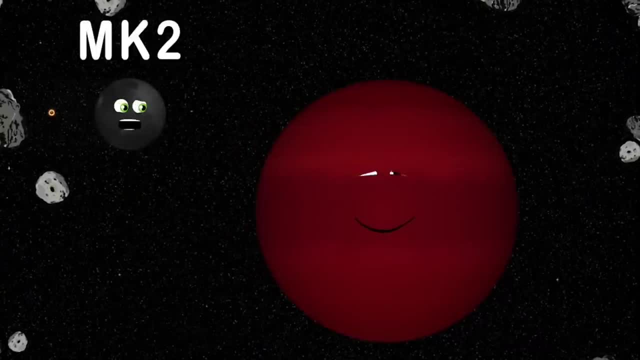 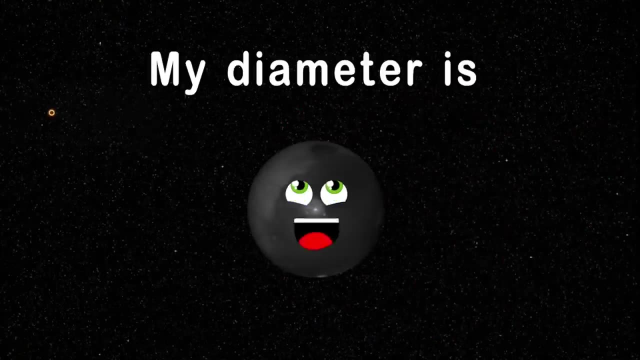 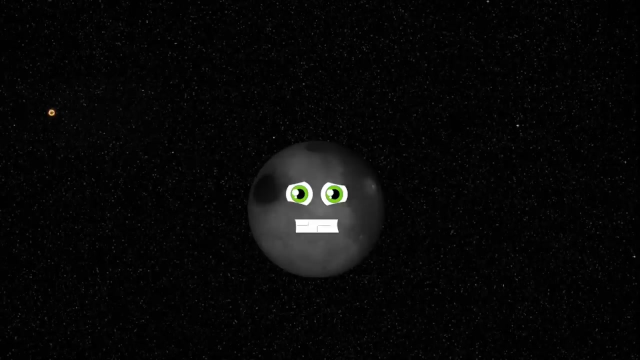 Hello, I'm MK2, a satellite of Mikey Mikey. I was noticed one year ago. now an official moon I'll be. It's estimated my diameter's 100 miles Across. that's an estimate only from a bunch of astronomers. I'm 1300 times more faint than dwarf Mikey Mikey. 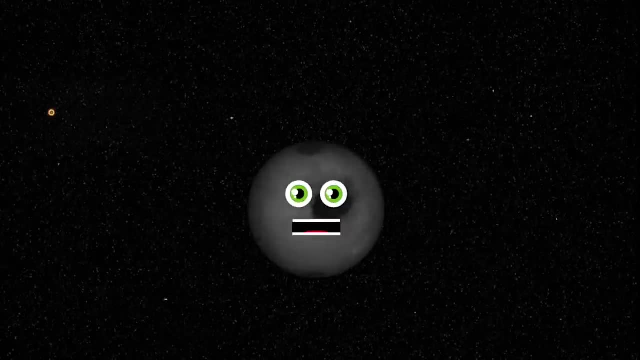 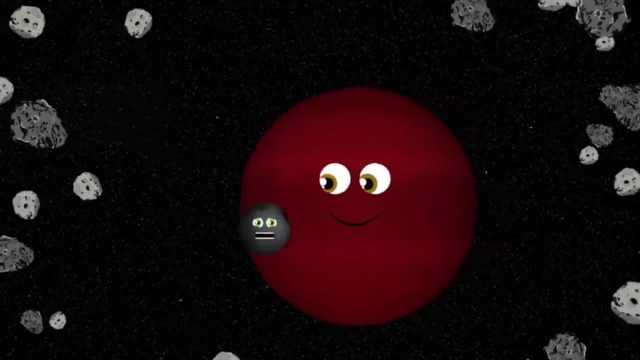 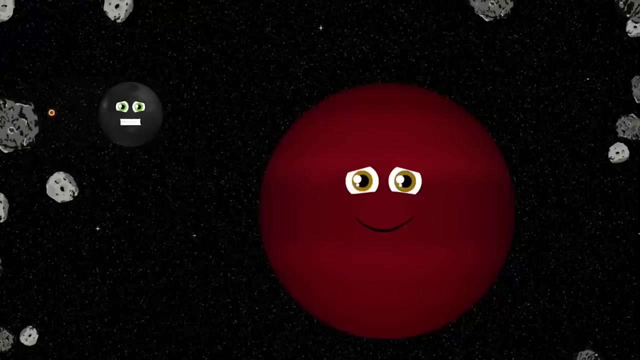 When a telescope gets closer, they will see me more clearly. I'm 13,000 miles from my dwarf planet, so bright, And I'm called a moon because I'm a natural satellite, Mikey. Mikey had what scientists thought were dark worm spots. Now they think it was me. 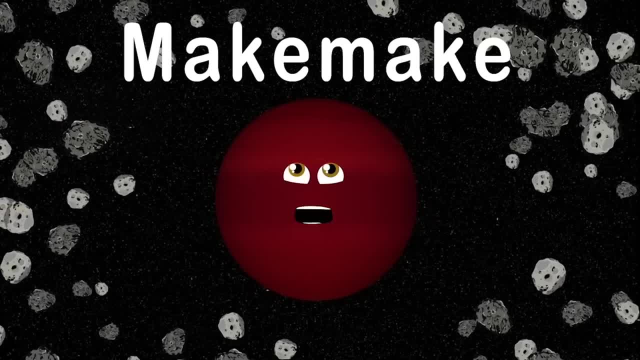 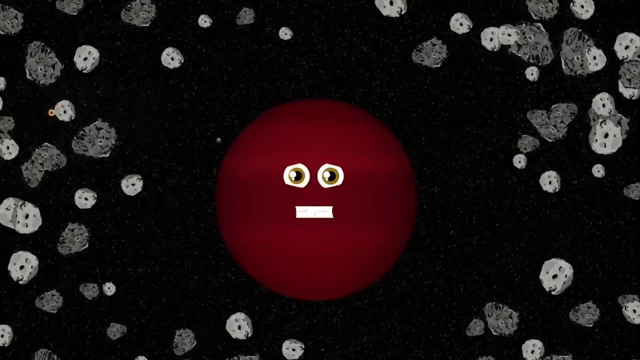 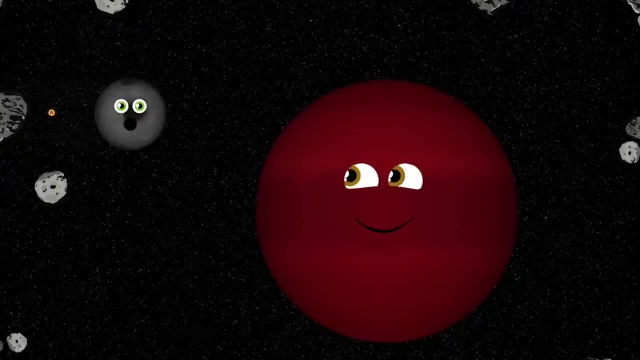 Making those moon-satellites look like stars, Worm dots. I'm Mikey Mikey. I have an official new moon. Let me introduce MK2 to all the world and you, Hello, I'm MK2, a satellite of Mikey Mikey. I was noticed one year ago. now an official moon. I'll be. 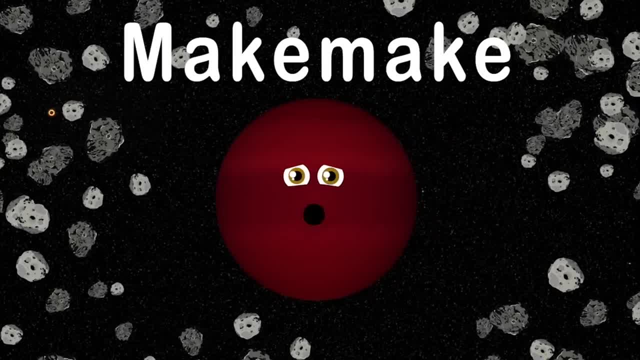 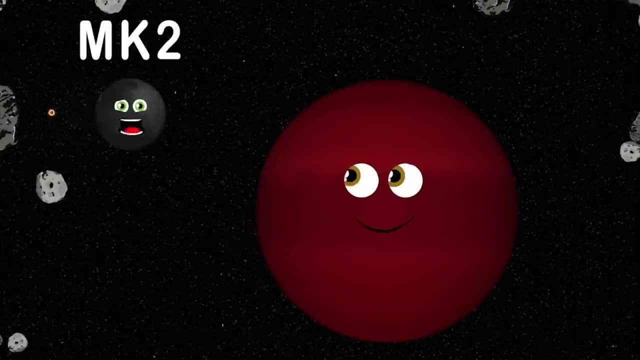 I'm Mikey Mikey. I have an official new moon. Let me introduce MK2 to all the world and you: Hello, I'm MK2. I'm MK2, a satellite of Mikey Mikey. I was noticed one year ago. now an official moon. I'll be. 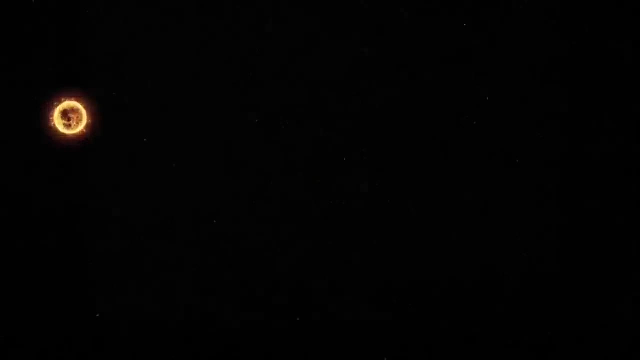 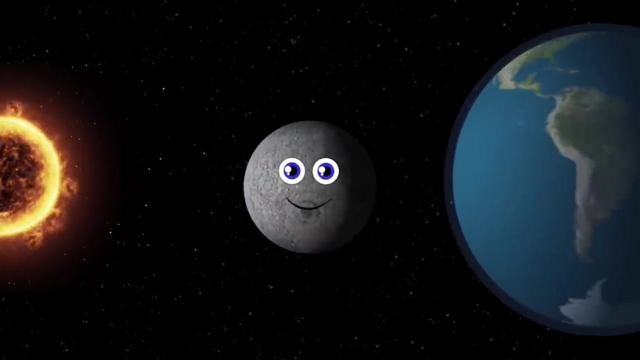 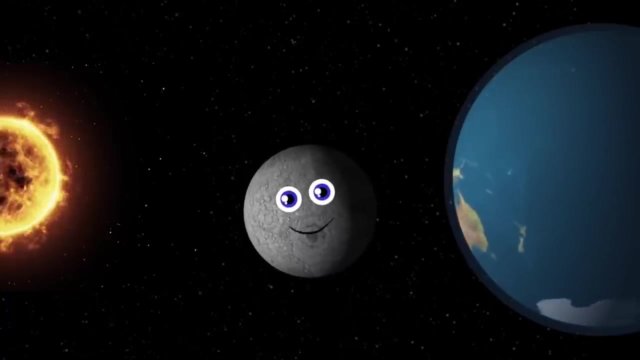 I'm Mikey Mikey. I have an official new moon. I was noticed one year ago now- an official moon. I'll be On the moon, Earth's natural satellite. I'm Mikey Mikey. I have an official new moon. I'll be. 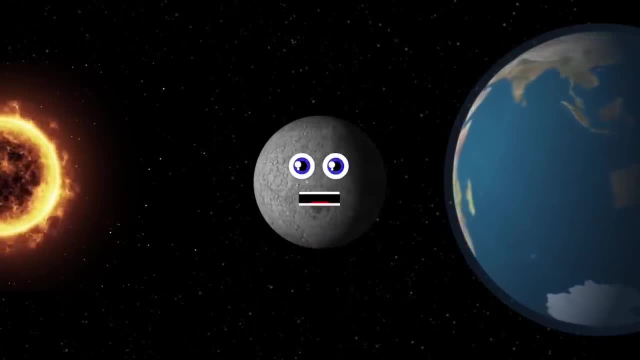 satellite. I rotate the same speed as the earth and I'm a natural source of light. I'm the moon. My appearance is gray and white. You only see one half of my surface, whether it's day or night. It's believed I was created 4.5 billion years ago, When a Mars-sized body collided with earth. 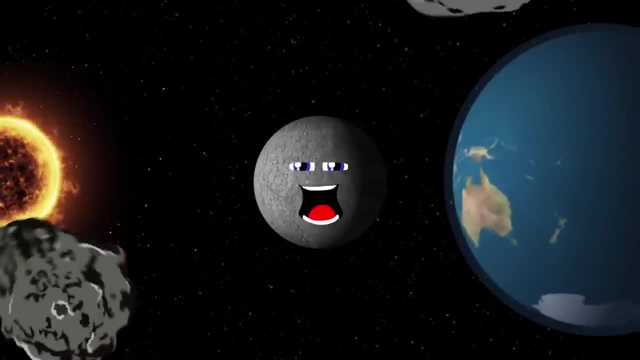 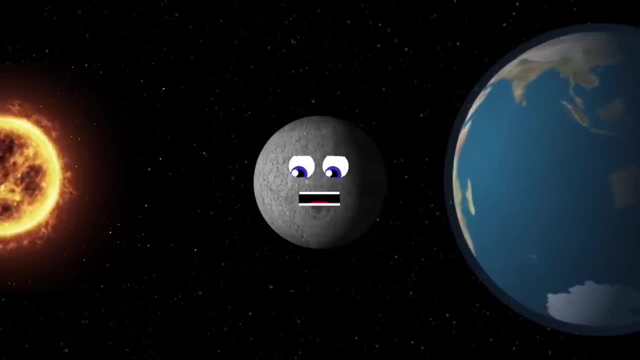 their debris formed me real slow. Meteors, asteroids and comets struck my surface for a billion years, due to the fact that they don't burn up in my thin atmosphere. If you wonder what a moon is, it's a natural satellite, One that orbits a single planet. 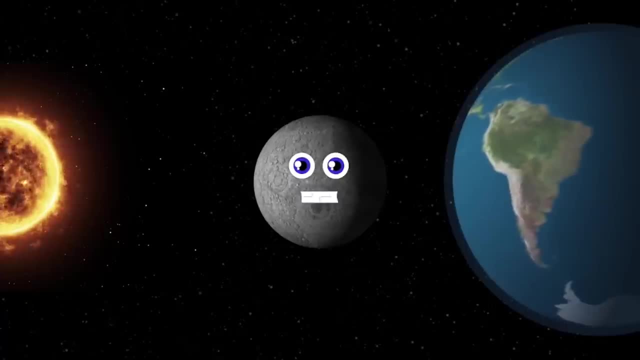 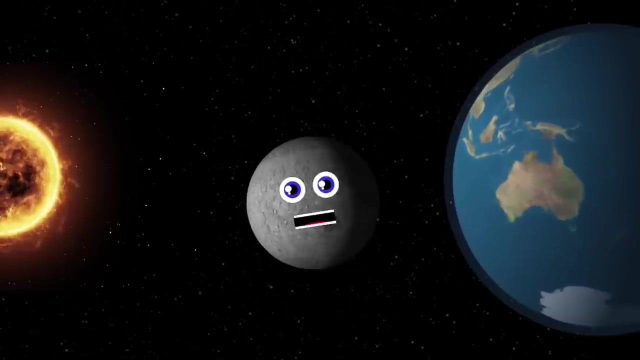 The planet orbits a star so bright. Scientific observations were first made in 1610 by Galileo Galilei, the astronomer Italian. I'm the moon, Earth's natural satellite. I rotate the same speed as the earth and I'm a natural source of light. 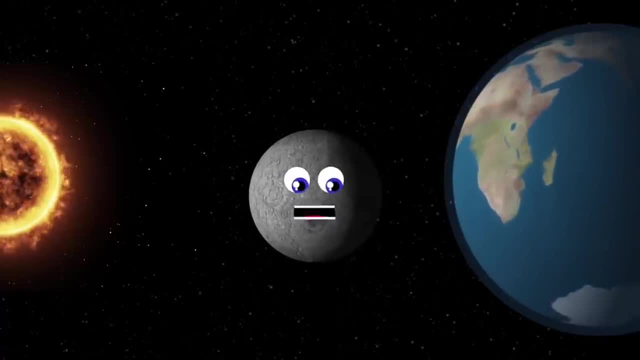 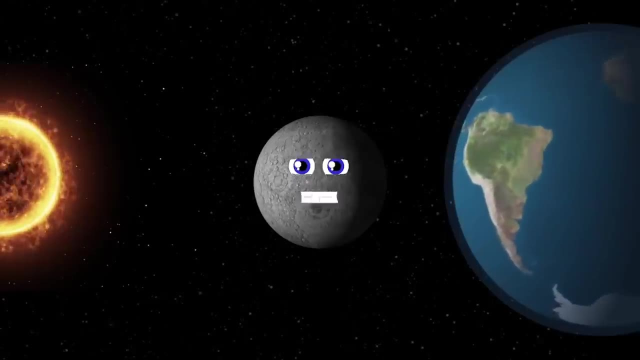 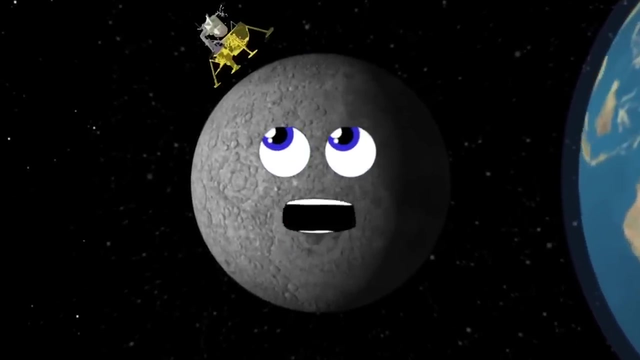 I'm the moon. My appearance is gray and white. You only see one half of my surface. whether it's day or night, When the earth spins on its axis, ocean levels stay the same. Then the moon's gravitational pull creates the tides that we see change. 238,900 miles from the earth is the 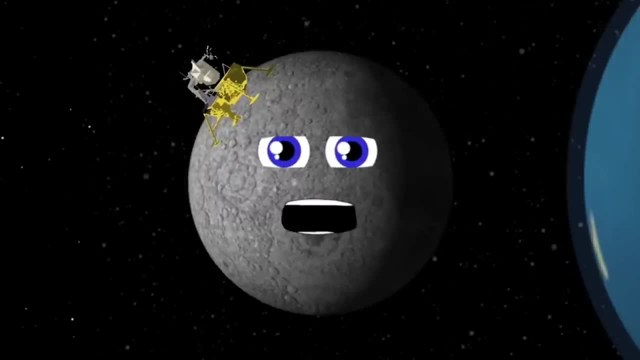 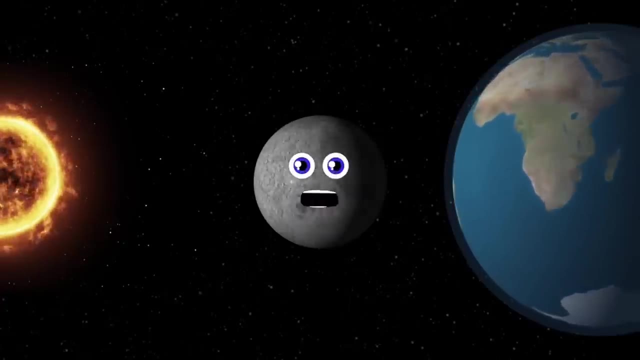 perfect distance measured when the first spaceship landed on my turf. The reason you see one half of my surface all the time is because my rotation's the same speed as the earth. thought in this rhyme, It takes 27 earth days for me to rotate. 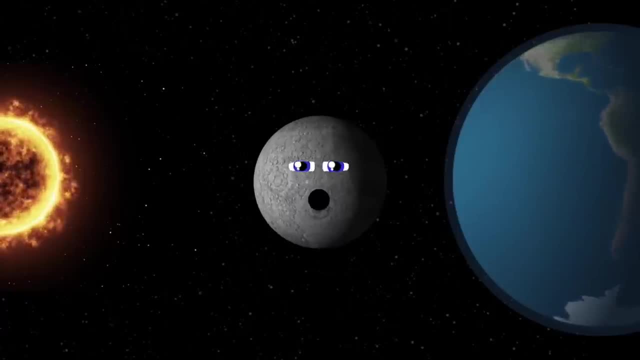 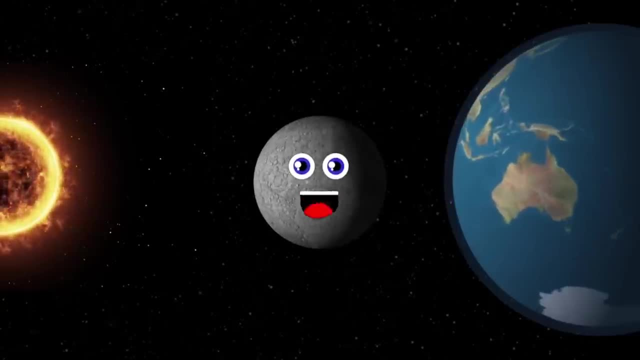 MONTH, enough to make me feet almost a veya log as increased byatively when step start. and why don't you notice that the screen is a90histoire higher than my disco quality? lightでは the earth and i'm a natural source of light. i'm the moon. my appearance is gray and white. 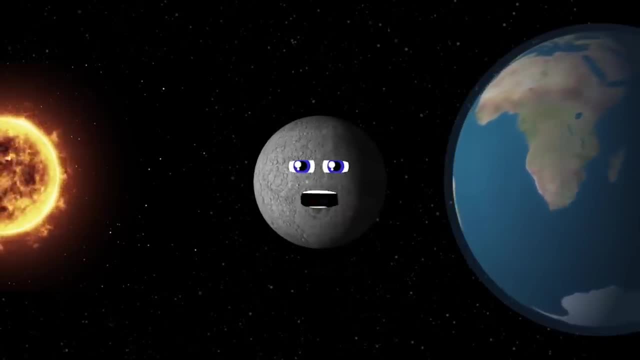 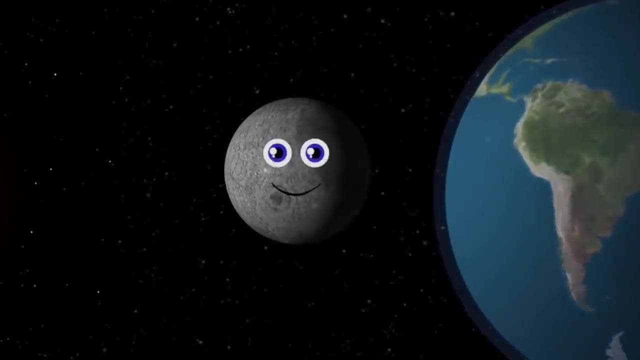 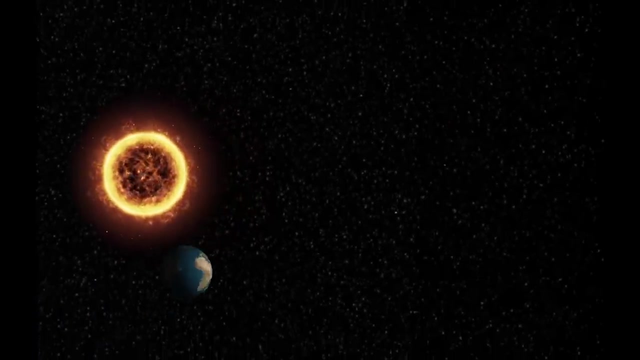 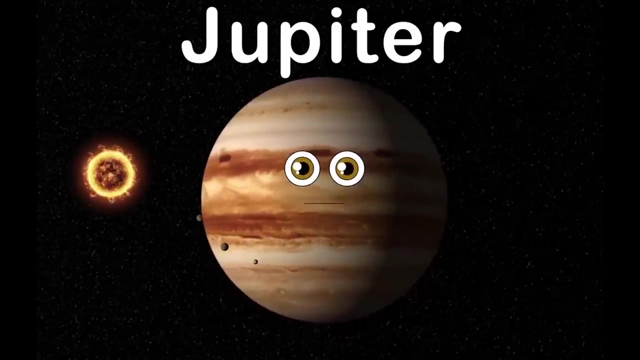 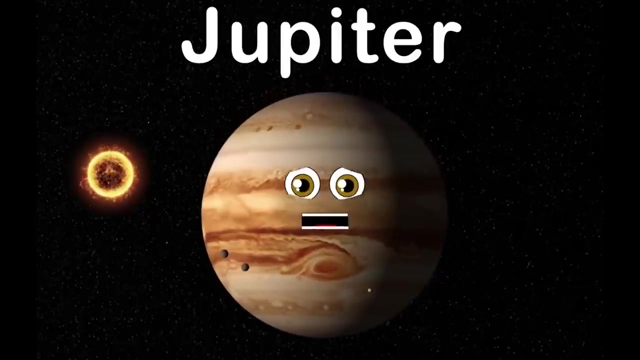 you only see one half of my surface, whether it's day or night. my name is jupiter, the biggest planet you see. no planet in our solar system is bigger than me. my name is jupiter, a windy planet i'd be, and i have six to seven. moons and i'm a natural source of light. i'm the moon. my appearance is gray and white. you only see one half of my surface, whether it's day or night. my name is jupiter, a windy planet you see. no planet in our solar system is bigger than me. 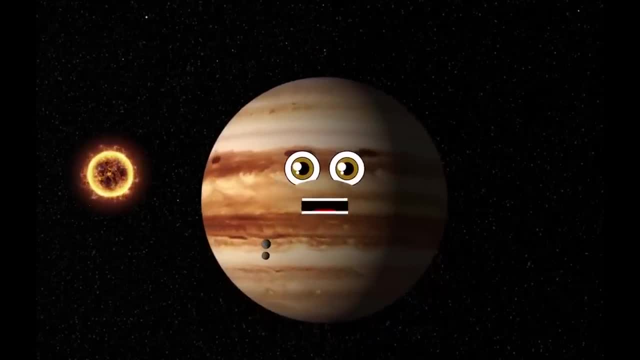 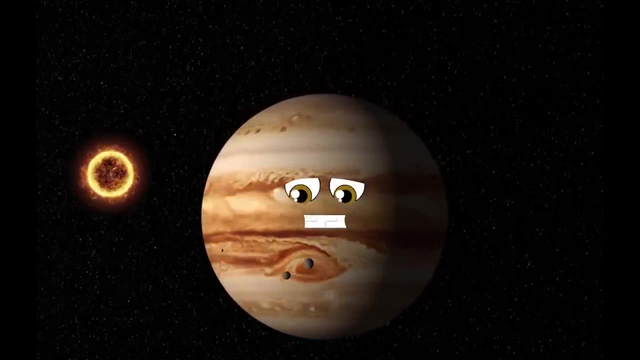 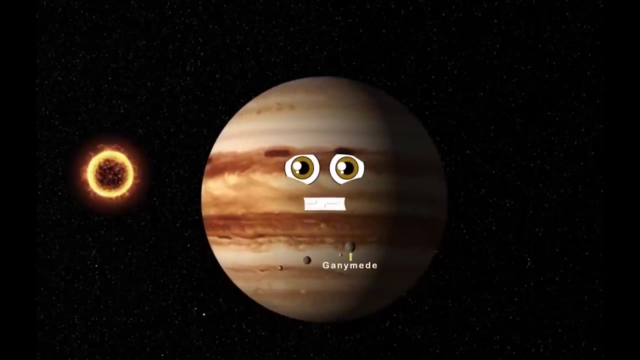 my name is jupiter, a windy planet. i'm the moon. my appearance is gray and white. the Romans gave me my name after their king of the gods because my size is so massive. in the sea of the stars, Callisto, Europa got a meaning. I owe all my four biggest moons found by Galileo. 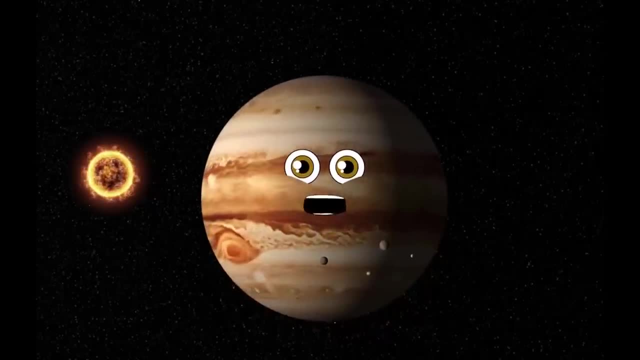 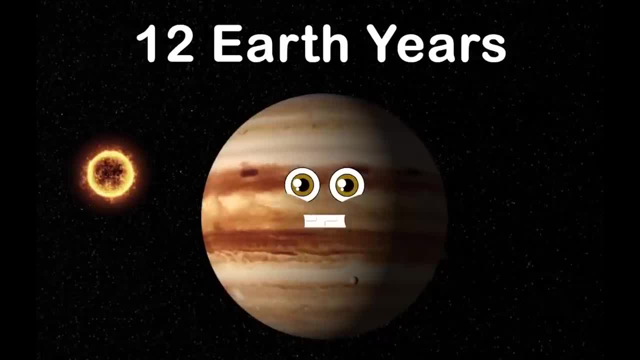 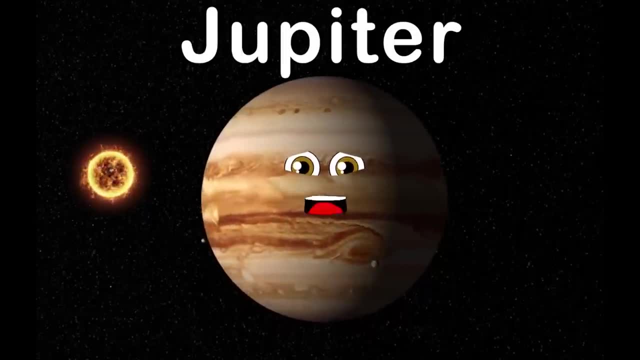 it takes twelve earths to make me a moon, five years for me to orbit the sun- that makes one year on my surface. that's a really long run. my name is jupiter, the biggest planet you see. no planet in our solar system is bigger than me. 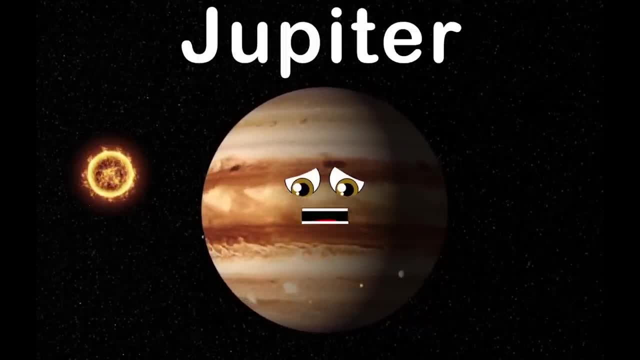 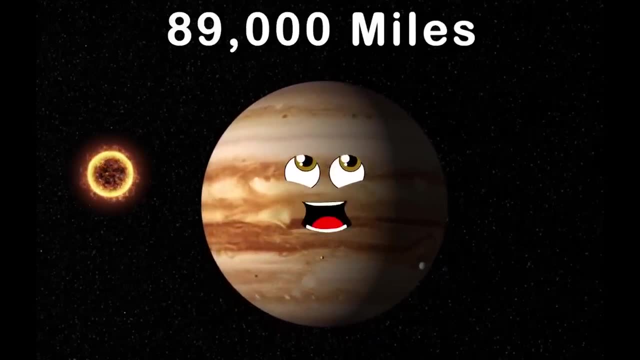 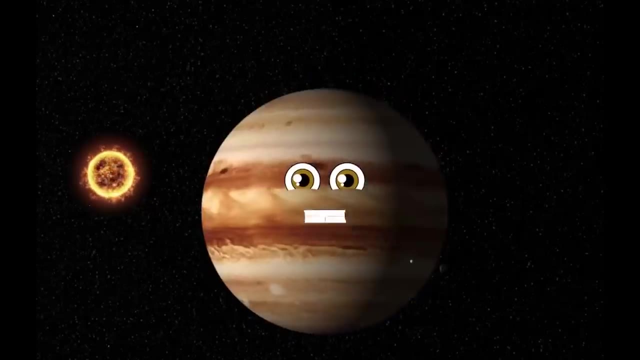 my name is jupiter. a windy planet i'd be, and i have six to seven moons that rotate round me, so free. eighty-nine thousand miles is the amount that I'm wide. I'm so big, I'm so big, I'm so big, you can fit one thousand earths inside. 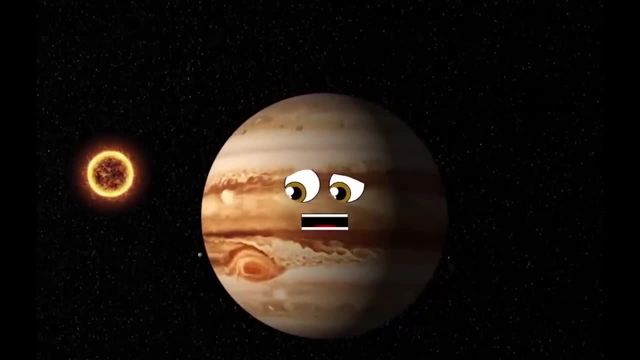 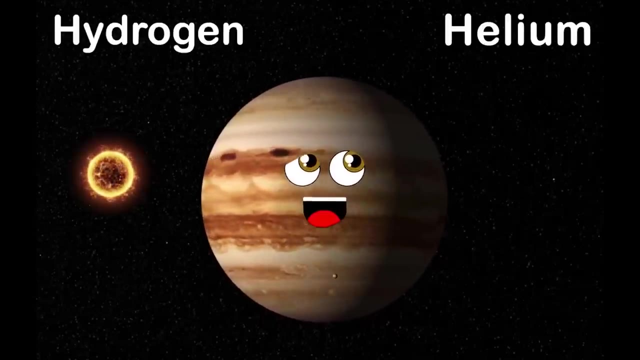 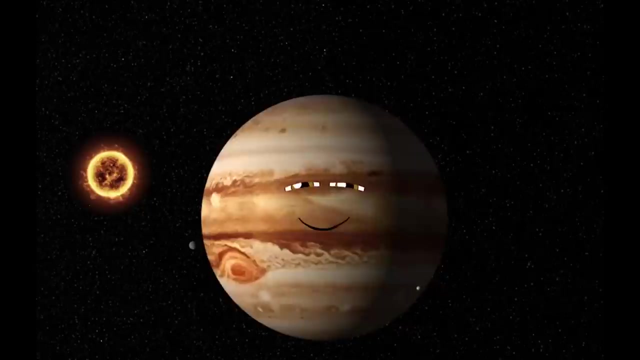 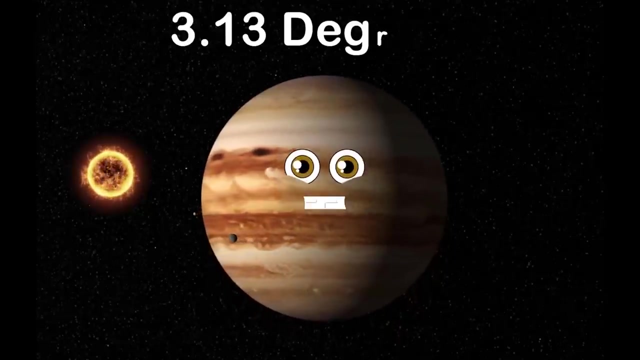 I've got a giant red spot. it is a raging storm. scientists think four hundred years ago is when it took form. hydrogen and helium make up most of my atmosphere. I am a gas giant in an impressive sphere. three point thirteen is the amount of degrees that I tilt on my axis. let's sing the chorus, please. 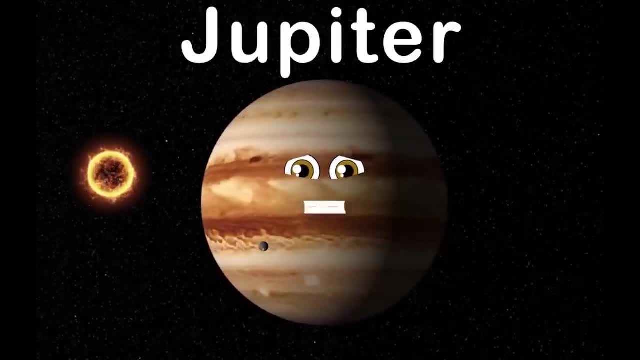 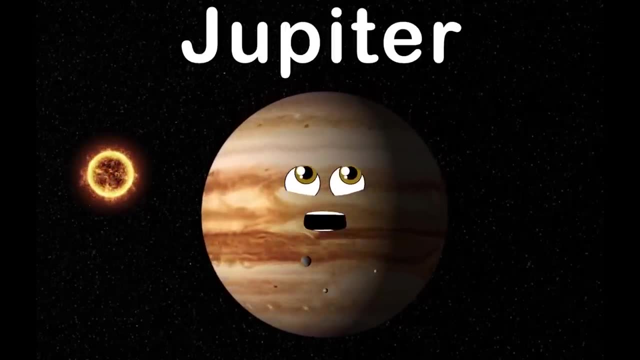 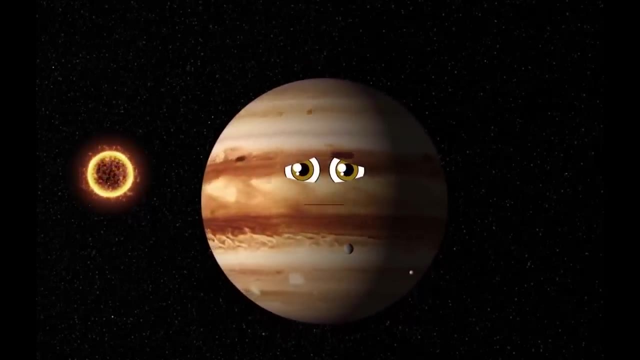 my name is jupiter, the biggest planet you see. no planet in our solar system is bigger than me. my name is jupiter. a windy planet i'd be, and i have six to seven moons that rotate round me, so free. if I were eighty times more massive, I would have become a star. 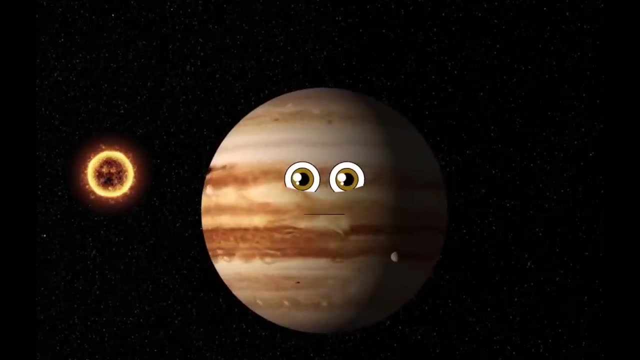 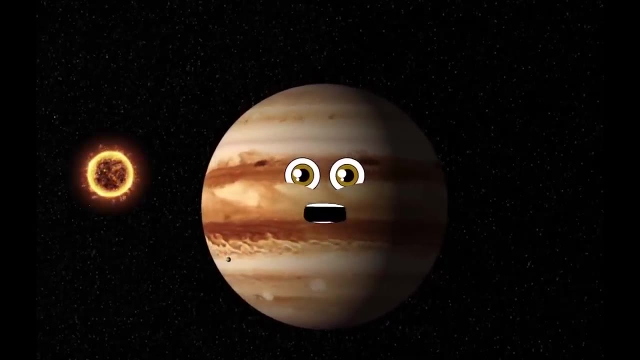 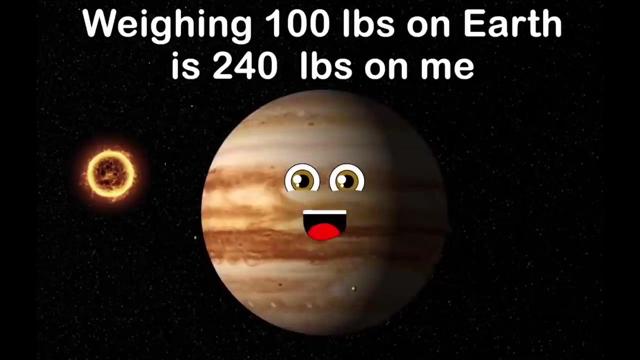 because I'm made of the same elements as the sun. how bizarre. that much mass would cause the pressure and temperature within me to snowball than me to cause hydrogen to fuse with helium, creating energy. my gravity's 2.4 times more than earth. so what does that mean? weighing a hundred pounds on earth is 240 pounds on me. my name is. 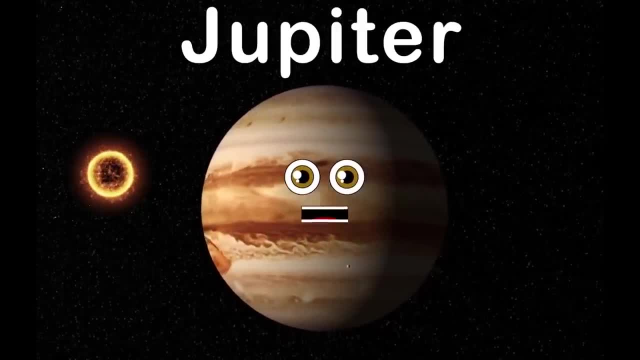 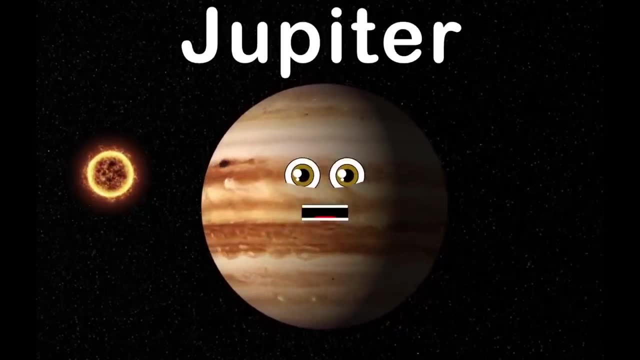 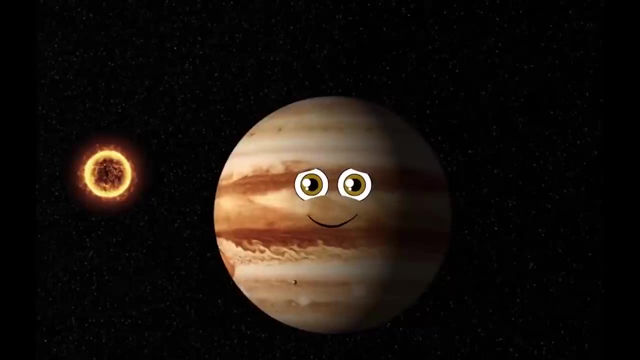 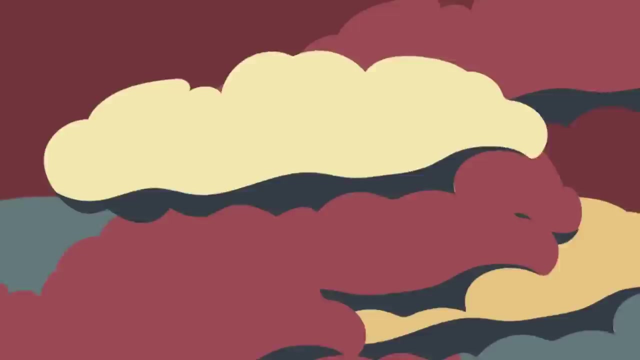 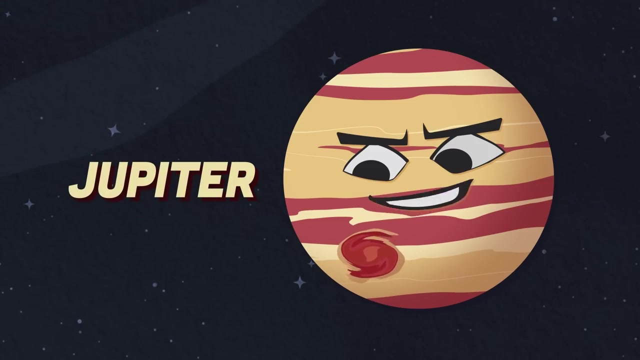 jupiter, the biggest planet you see. no planet in our solar system is bigger than me. my name is jupiter- a windy planet i'd be, and i have 67 moons that rotate around me, so free. one of the biggest storms in our solar system is the great red spot on the fifth planet from. 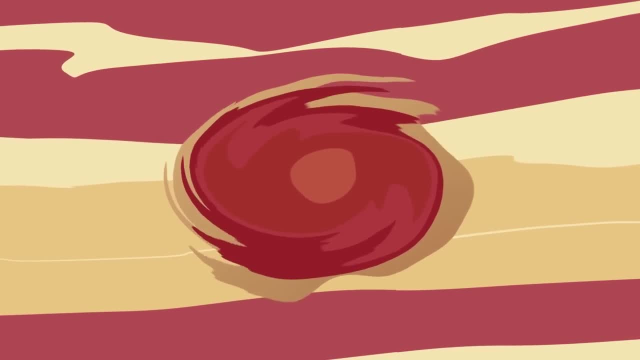 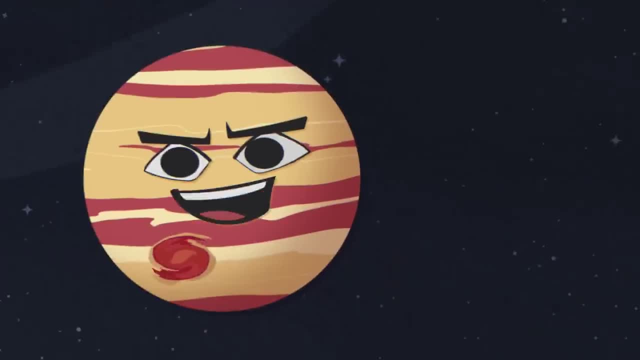 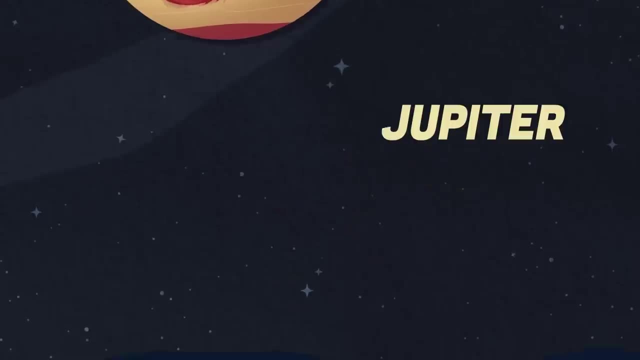 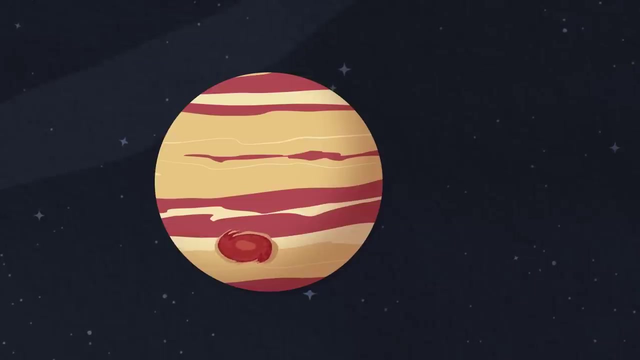 earth's storms that are strong in the atmosphere on the fifth planet from the sun, on the planet jupiter, is where the storm begun. in the 17th century, astronomers turned their telescopes to planet jupiter with nothing but a hope. they said they saw a spot in the planet's atmosphere, but it. 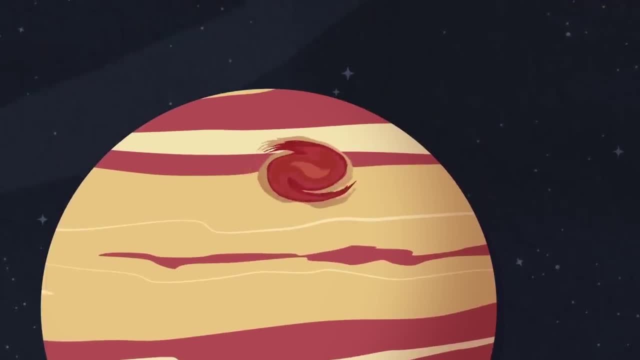 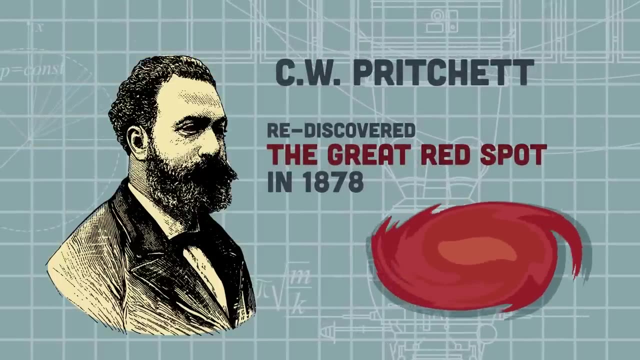 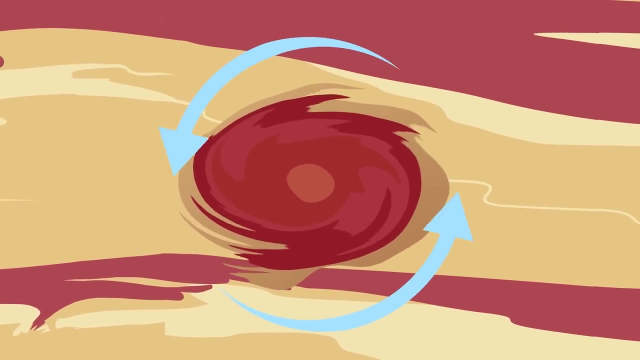 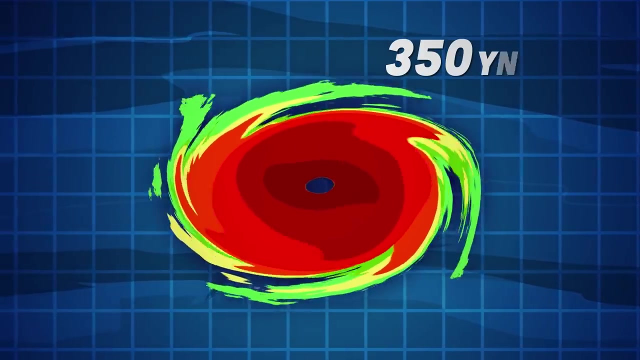 could have been in a different belt they saw in their years. astronomer cw pritchett rediscovered on a date the great red spot. in 1878 he looked closely in the southern hemisphere, a spot spinning counterclockwise and it was made clear the high pressure system was definitely a storm that lasted. 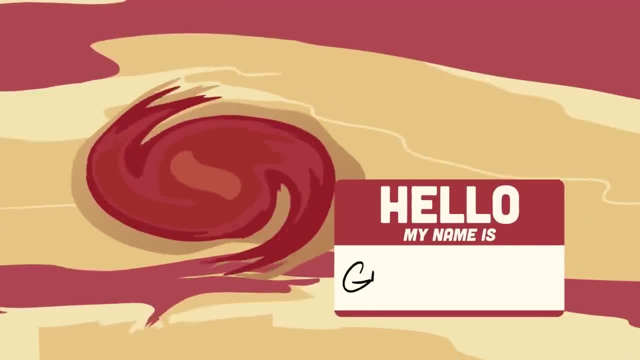 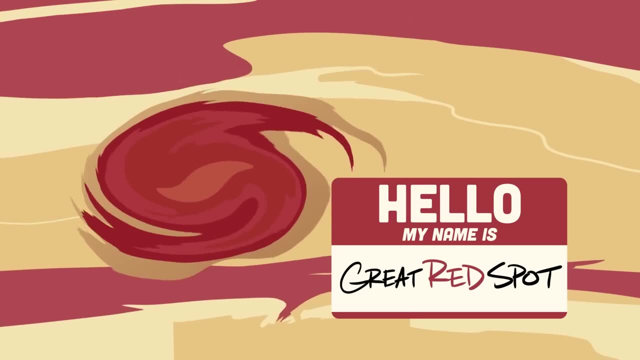 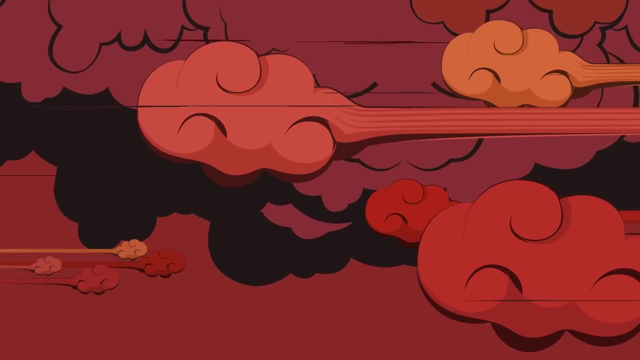 over 350 years since it was formed, the great red spot. it was officially named since astronomers telescopes did take aim. it produces wind speeds of up to 100 kilometers per second and it was up to 150 miles per hour, but from a distance looks like red beauty with power. jupiter's dry. 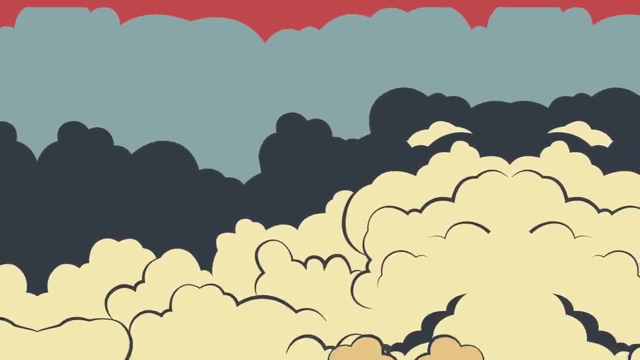 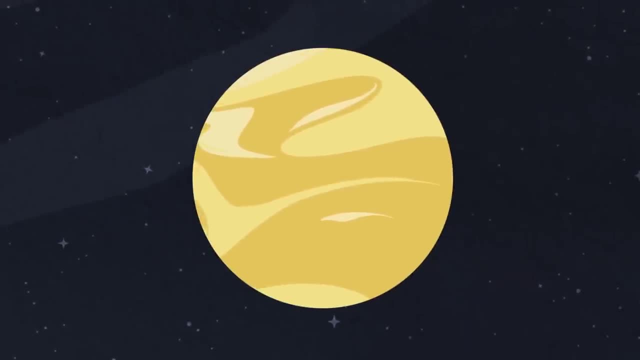 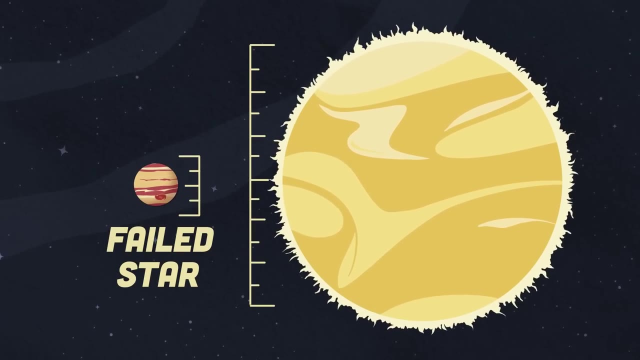 atmosphere is made up of elements i name hydrogen, helium, ammonia and methane. these same elements are what made up the sun. so why didn't jupiter become a star on its run? jupiter's not massive enough, so it's called a failed star. there's not enough internal pressure to create the fusion. 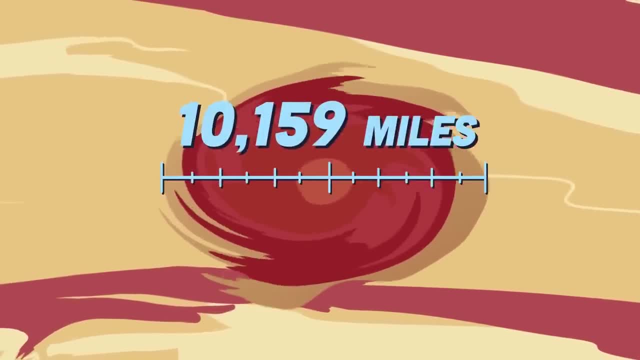 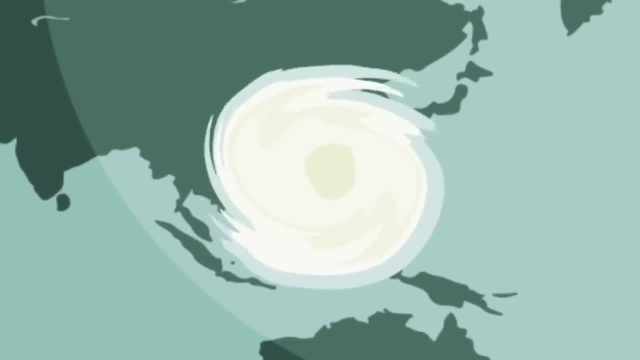 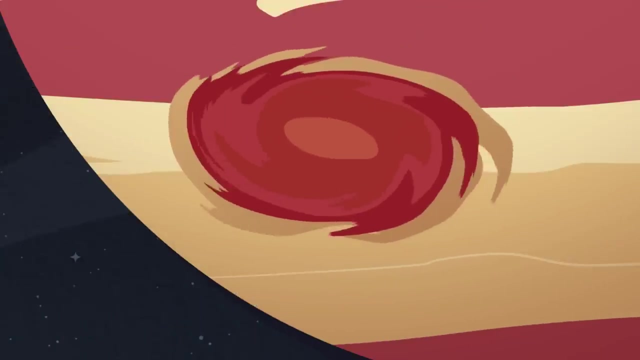 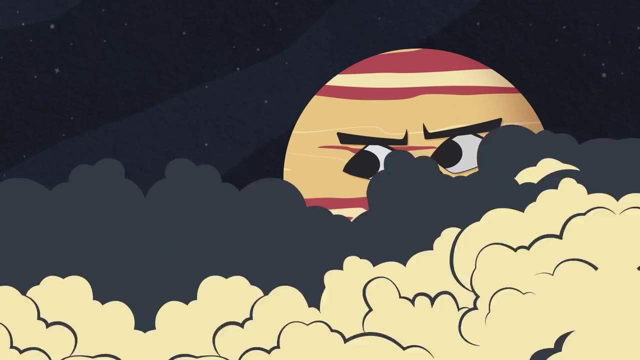 it's bizarre: 10 159 miles wide. it's so massive you could fit two earths inside. the great red spot is like a hurricane on the earth, but much more powerful and larger since its birth. one of the biggest storms in our solar system is the great red spot on the fifth planet from the sun. 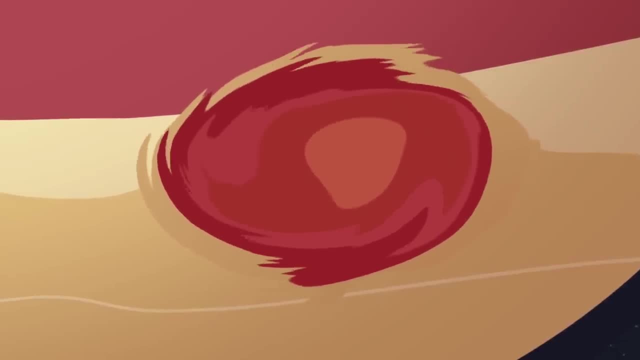 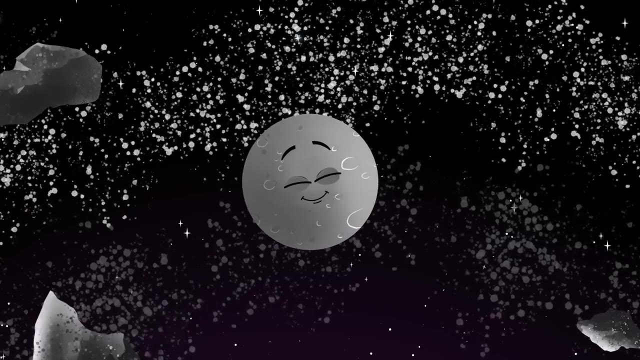 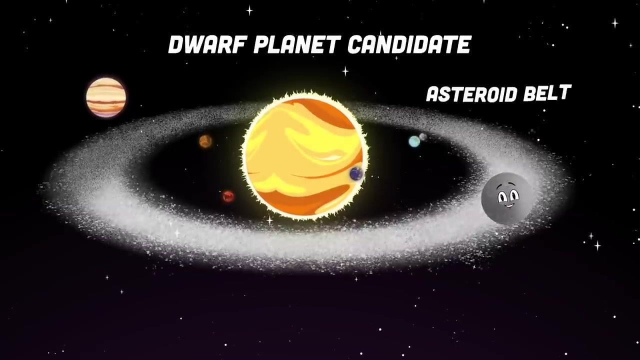 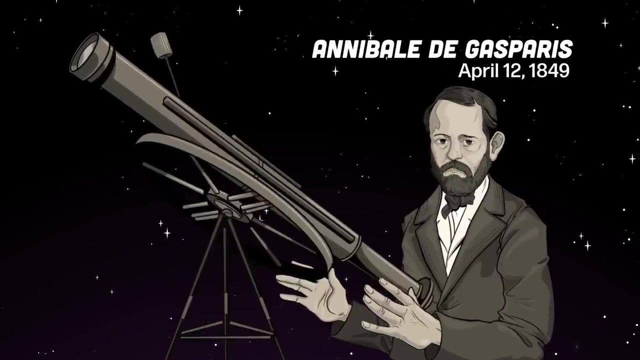 jupiter's high pressure region is persistent and long, with wind speeds that would dwarf earth, storms that are strong. my name's ig, a minor planet, designation 10. hygieia, a dwarf planet candidate in the asteroid belt. it's nice to meet you. discovered by annie belle de gasparissa on the 12th of april in 1849. i did. 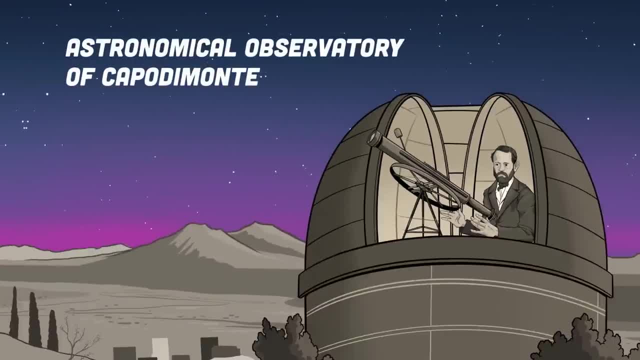 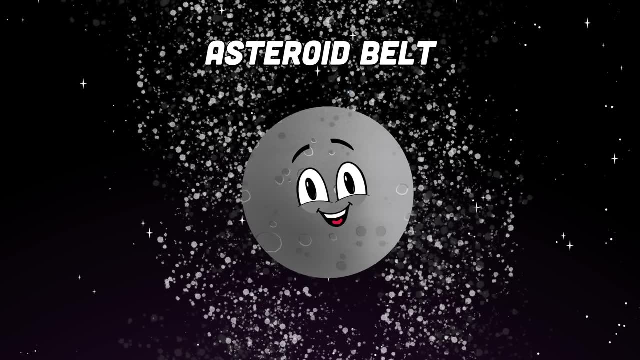 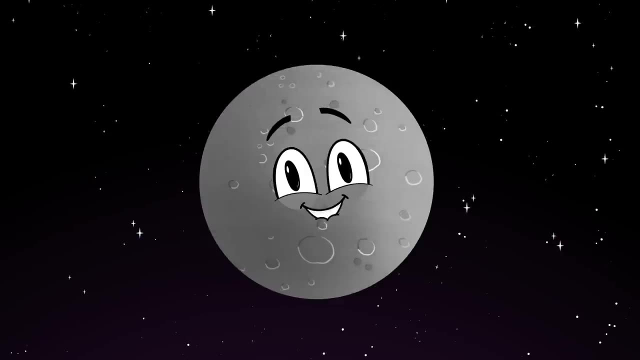 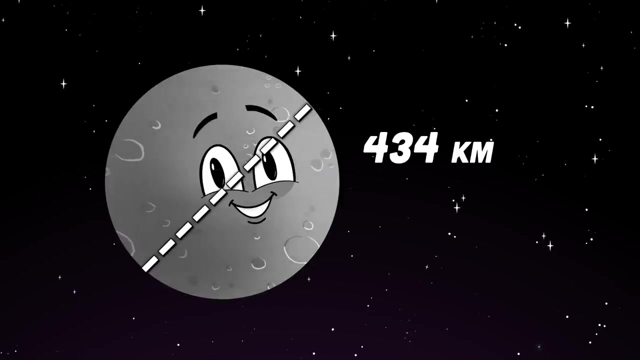 teach ya, discovered at the astronomical observatory of capa de monte, is where i was first seen. i'm located in the main asteroid belt between jupiter and mars is where i am felt. i do have a diameter of 270 miles or 434 kilometers, all the while i have a mass which is three percent of 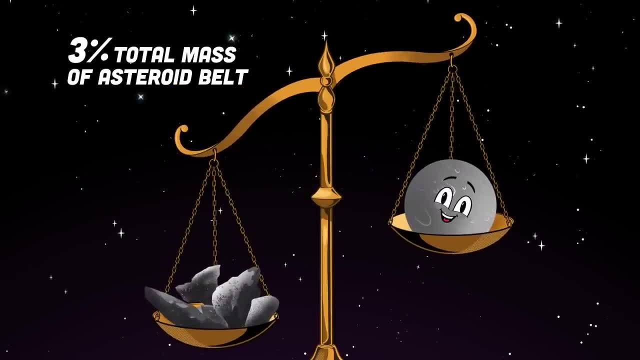 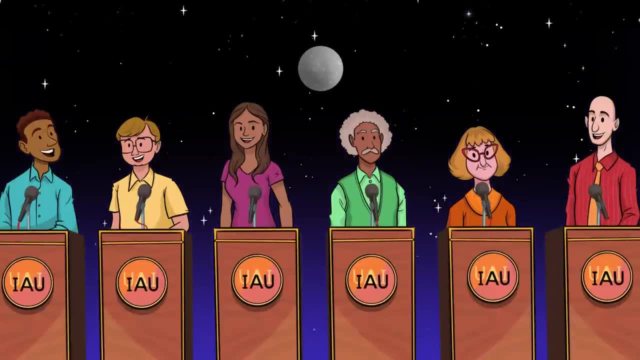 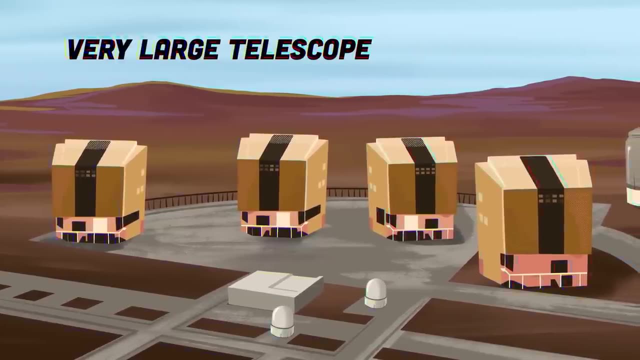 the total mass of the asteroid bella and the fourth largest asteroid by volume and mass in your system, delt. it's possible i'm a dwarf planet, but no one knows for sure. so the iau has classified as an asteroid until they're assured. observations with a very large telescope in 2018 revealed that. 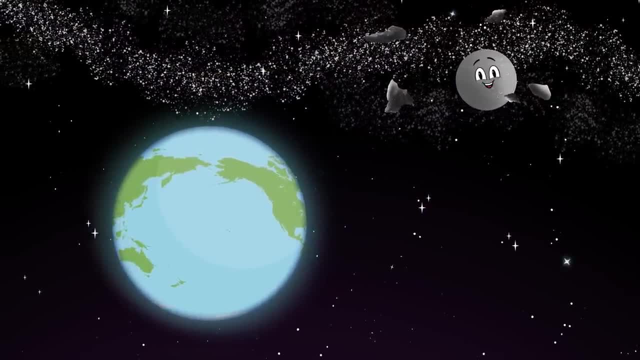 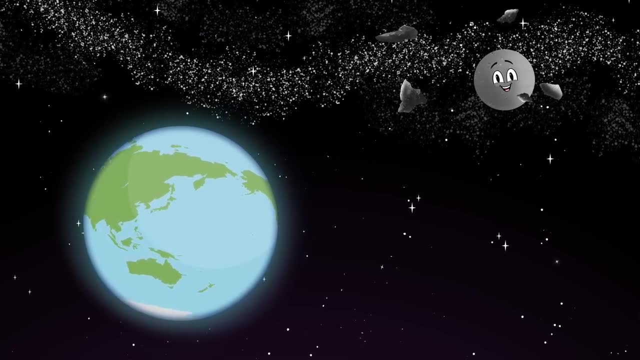 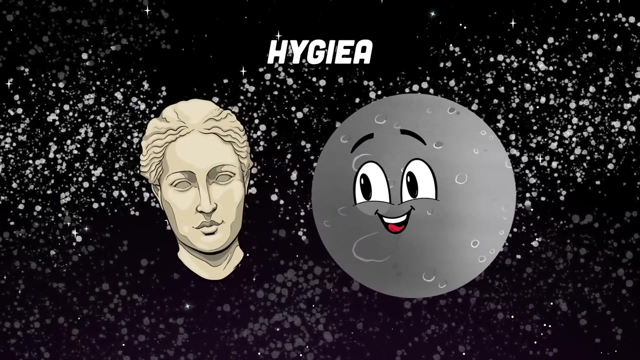 i'm nearly spherical, in which i'm so keen. i have a dark surface when observed from the earth. this is because of my position in the outer main belt. of course, i was named hygieia after the goddess of health, which is a greek goddess as well as roman. i tell it takes me 2033 earth days to orbit. 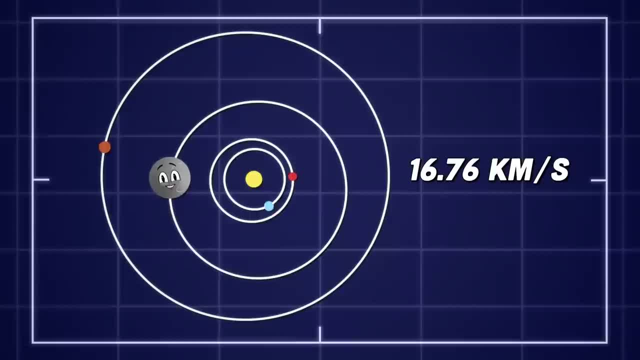 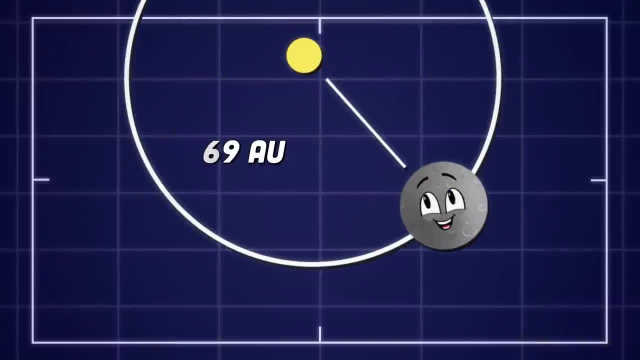 the sun at 16.76 kilometers per second. i come as close as 2.79 au to the sun on my run and reaching as far as 3.49 au from the sun. i'm 1.78 au from earth's orbit. at my closest point there's an. 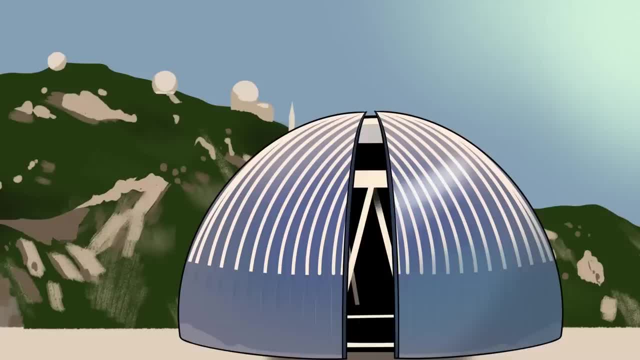 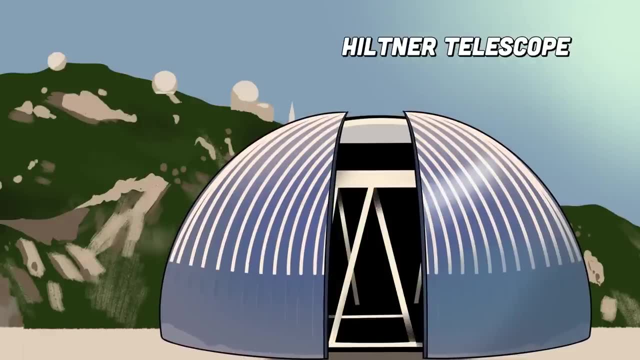 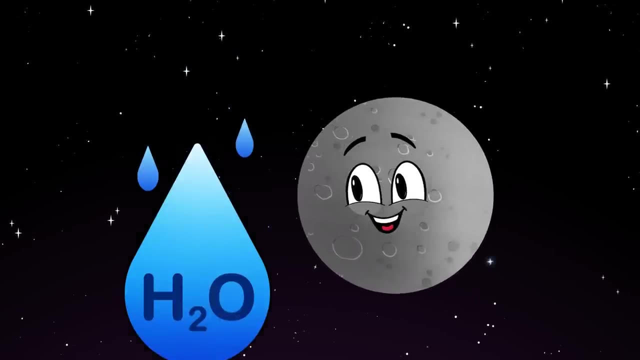 extremely wide berth between hygieia and earth is my point. hygieia's small main belt asteroid spectroscopic survey is observed with a 2.4 meter heltner telescope. primarily, this mass to observation indicates i may contain water and iron, but wait also nickel, ammonia, cobalt and nitrogen. 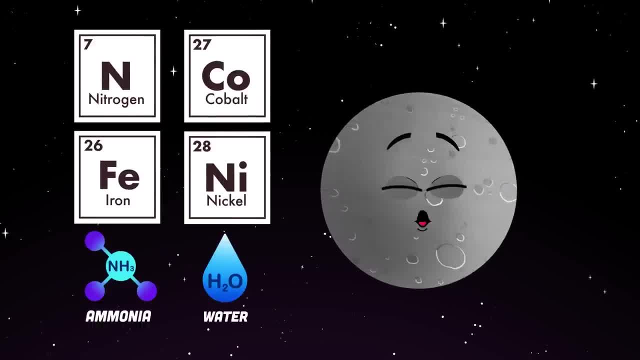 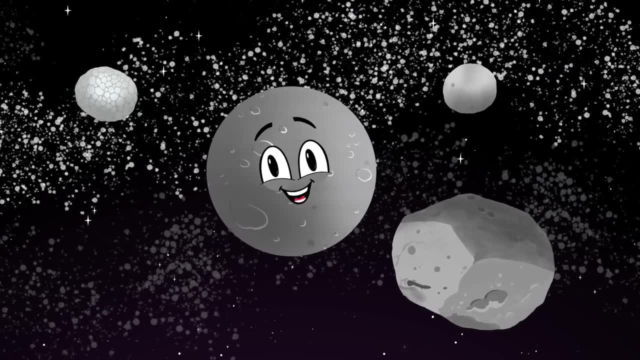 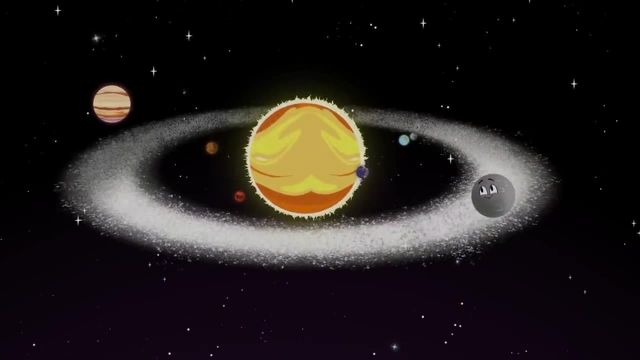 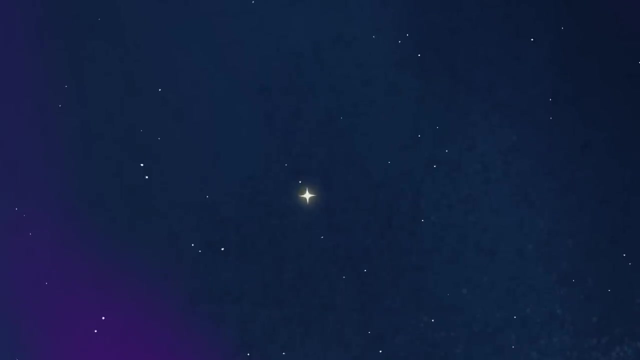 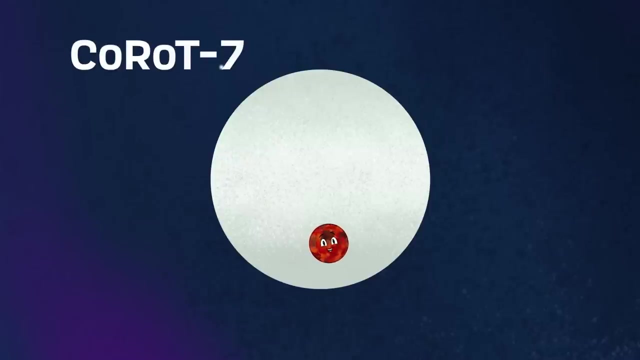 that's a lot of new information about me. for the win, my properties are the least known out of the big four objects in the main belt humans have explored. i'm an exoplanet orbiting the star carol 7, you see, in the constellation of monoceros. my name is carol. 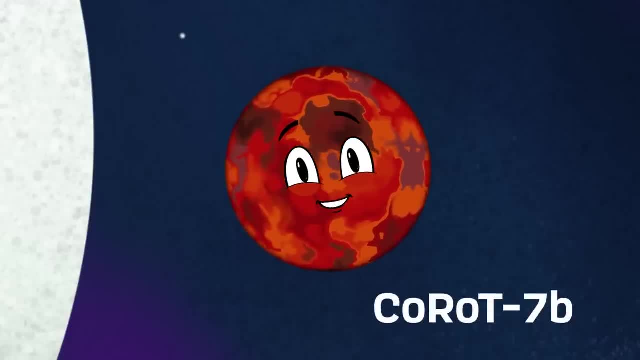 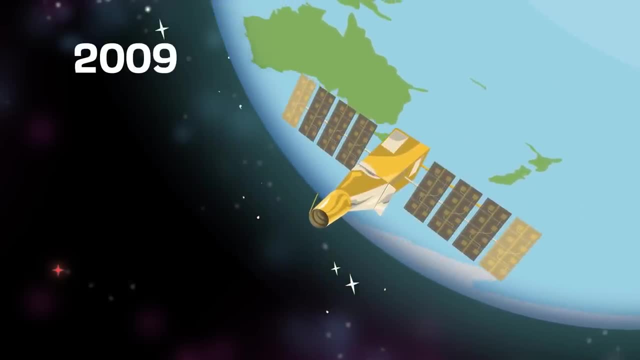 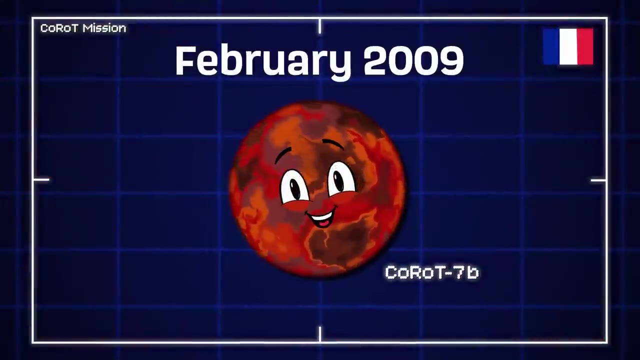 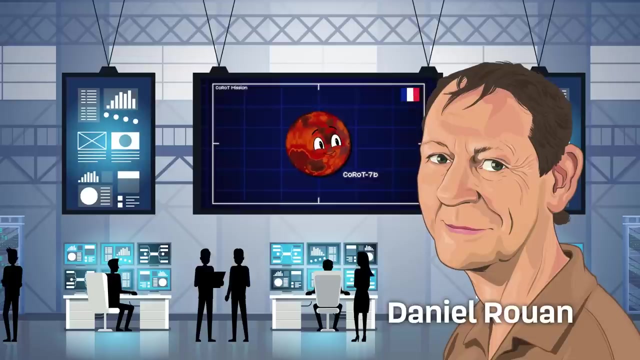 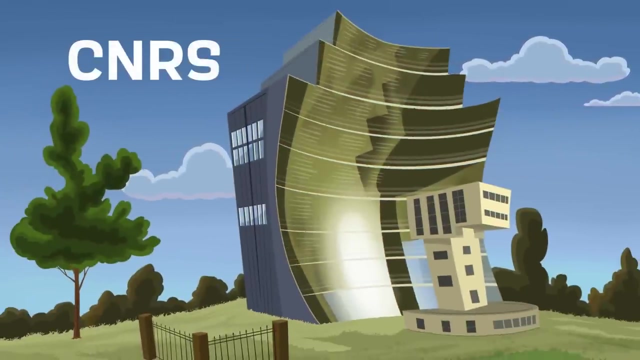 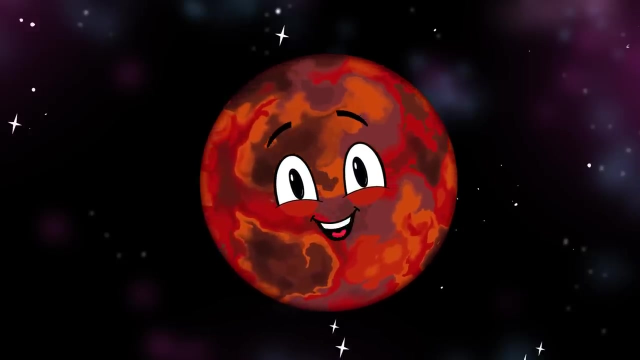 7b. i was first detected photometrically in 2009 by the french led coro mission. in the month of february i refined. i was discovered by a french astrophysicist named daniel new НАРЫЧИВОЙ. 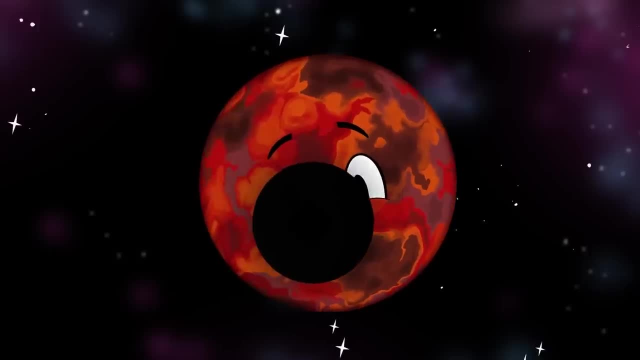 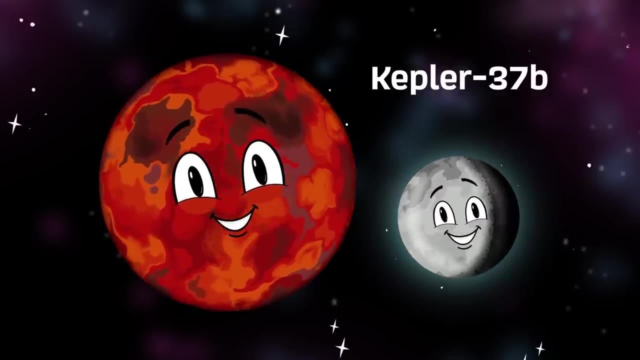 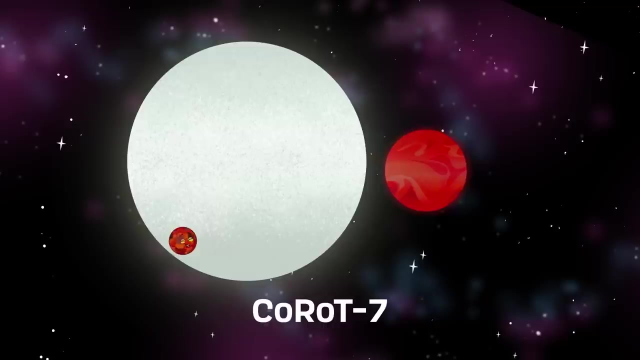 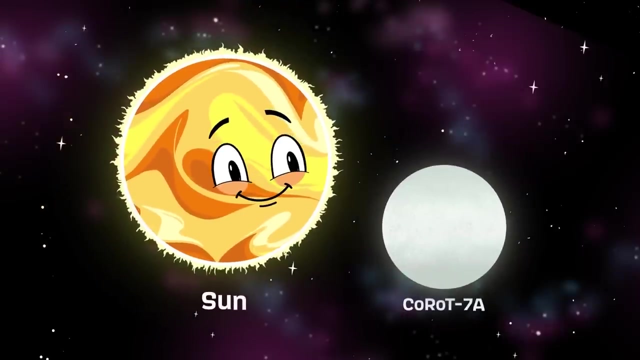 RO plant of the exoplanet that was given the name Kepler's 37b. I'm to orbit in a binary star system called Karo 7. here, Karo 7a is the g-type main sequence star, smaller and cooler than your sun, so we're. 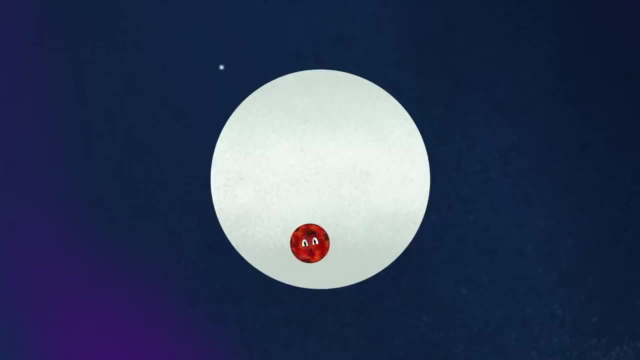 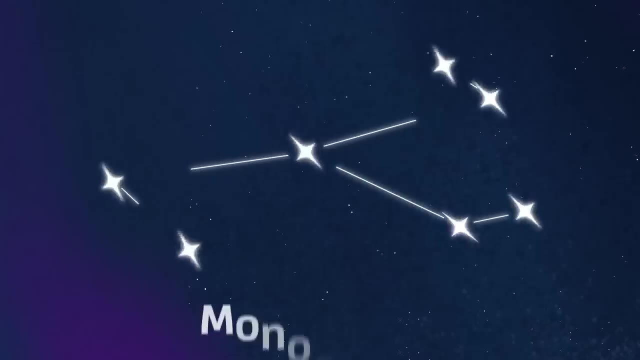 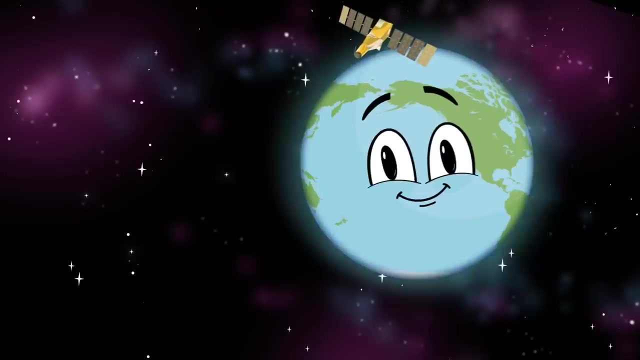 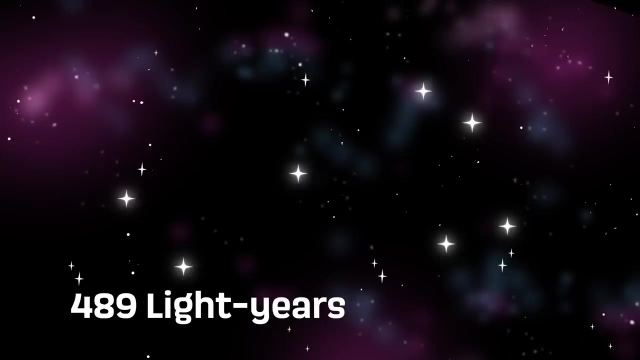 clear. I'm an exoplanet orbiting the star Karo 7. you see, in the constellation of Monoceros, my name is Karo 7b. when you travel 489 light years from the earth to the constellation of Monoceros, you'll 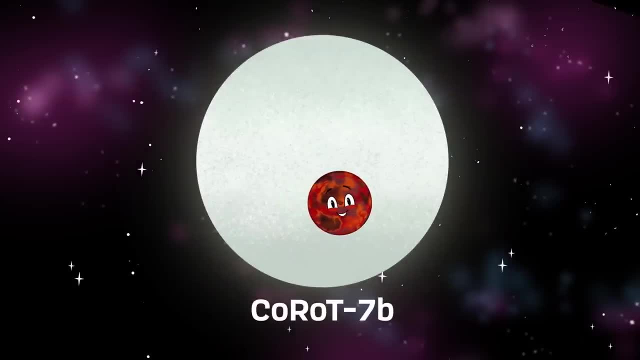 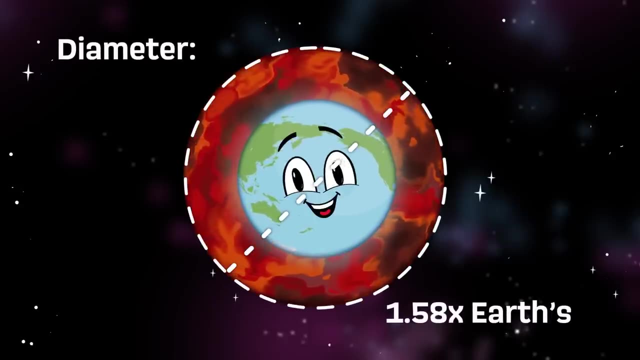 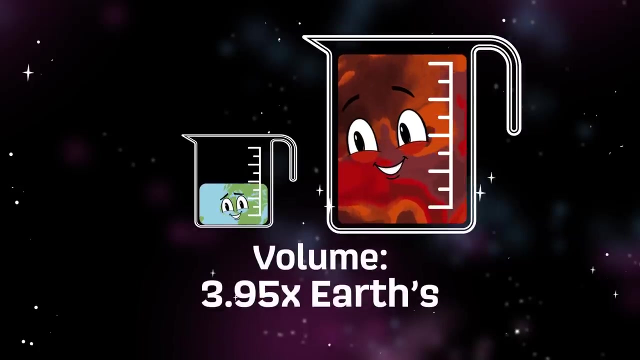 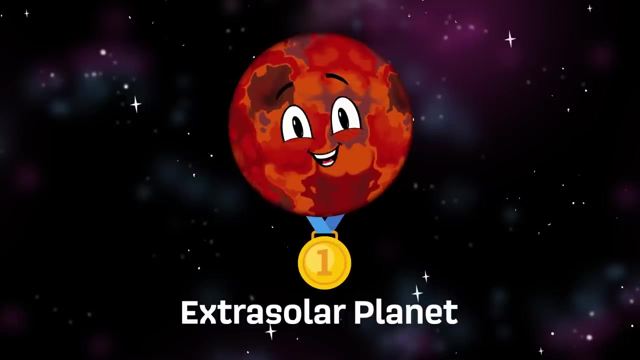 find Karo 7b. since its birth. I have a diameter measured at 1.58 times that of the earth. that means I have a volume 3.95 times earth. I was the first extrasolar terrestrial planet to be found. I have a very short. 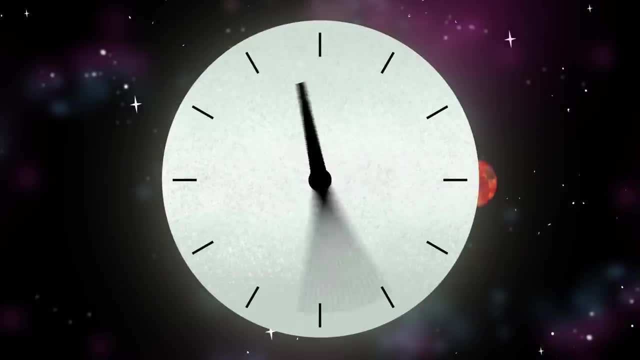 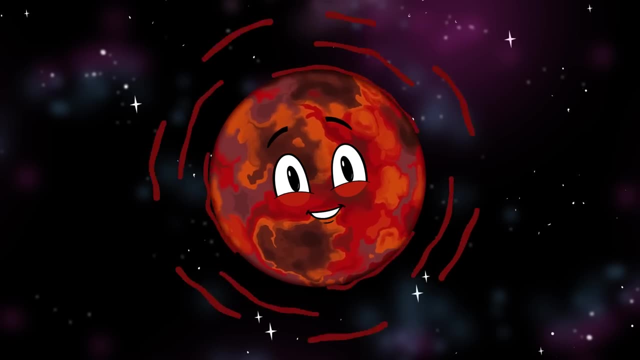 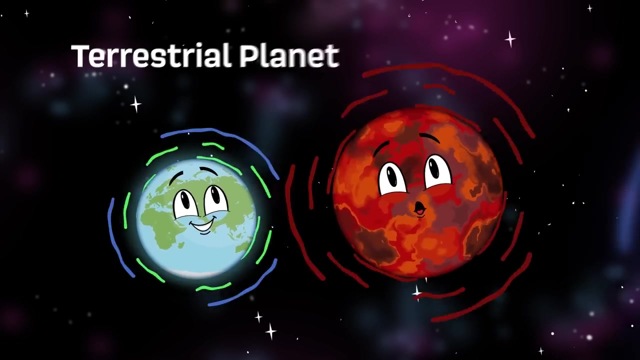 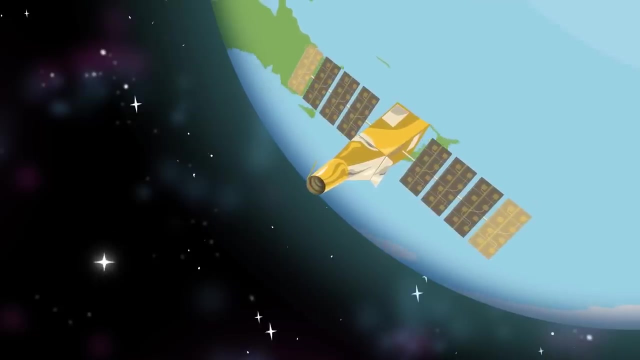 orbital period every 20 hours my star I spin around. the density of my planet is about the same as the earth. that's why you know I am a terrestrial planet and not a gas giant. for what that is worth, astronomers watched my host star from earth and contacts thought: no surprise. 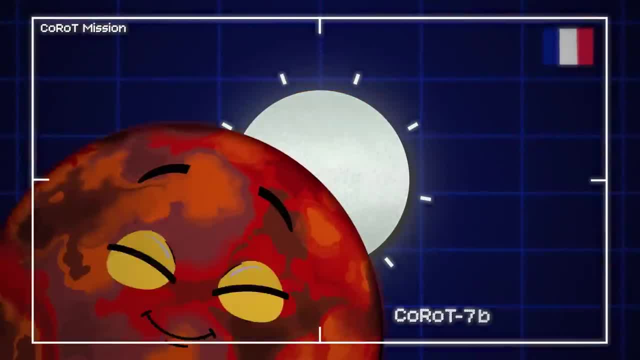 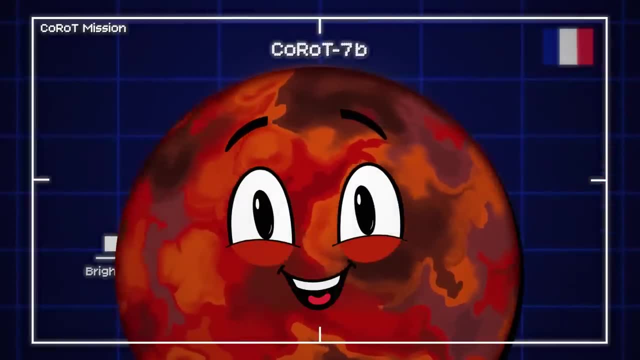 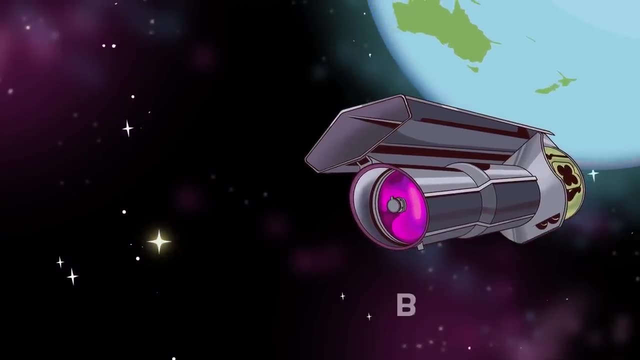 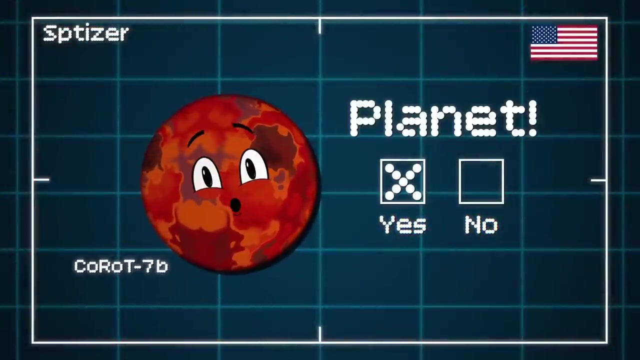 minute trouser shift photos and go 我 Dipping brightness. together with my star size Estimate allows the calculation of my planet size. After I was discovered. An independent validation was supplied By the Spitzer Space Telescope, Which confirmed I am a planet bonafide. My mass is still unconfirmed. 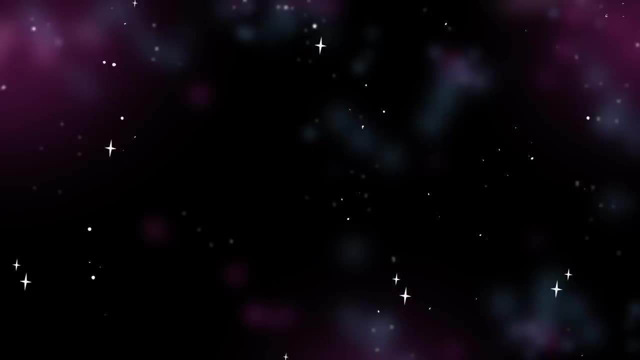 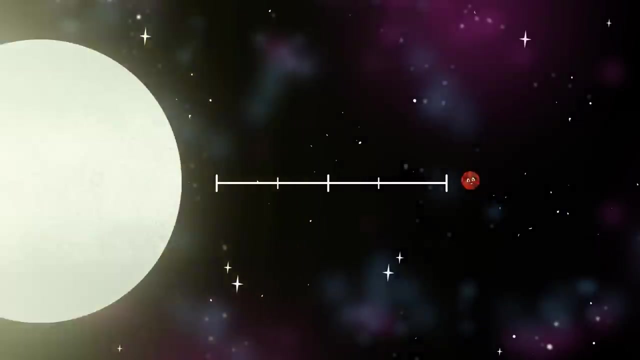 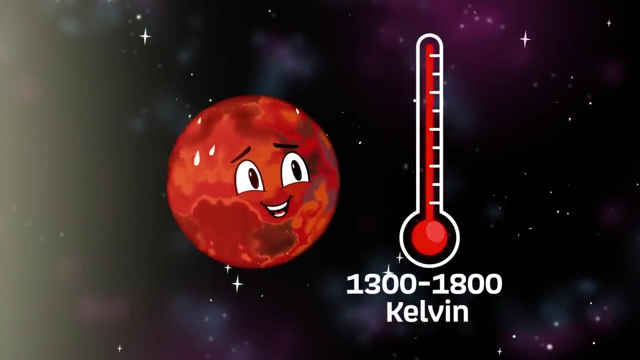 But it does range in between Two and eight Earth masses. This is all that they have seen. I orbit my star much closer than planet Mercury does To your star. I have a temperature of 1300 to 1800 K K meet Kelvin. the name is bizarre. 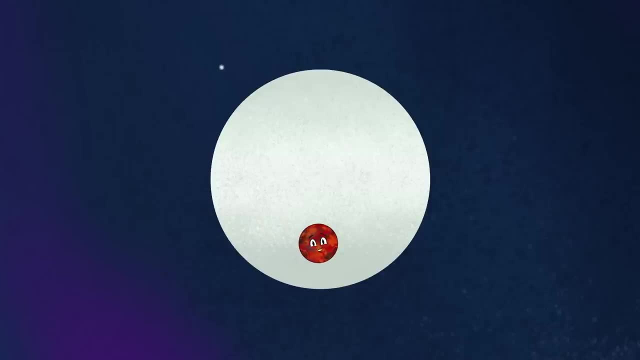 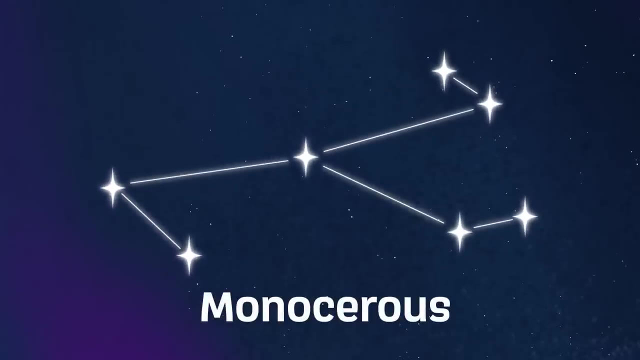 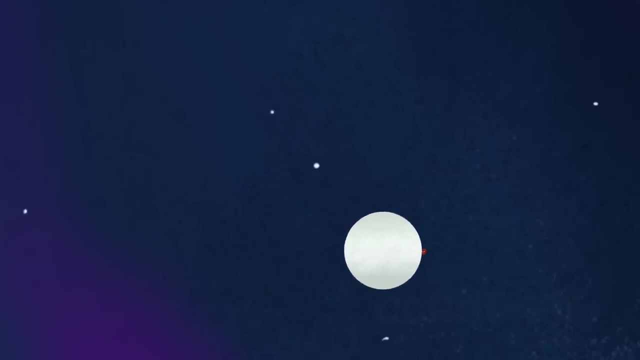 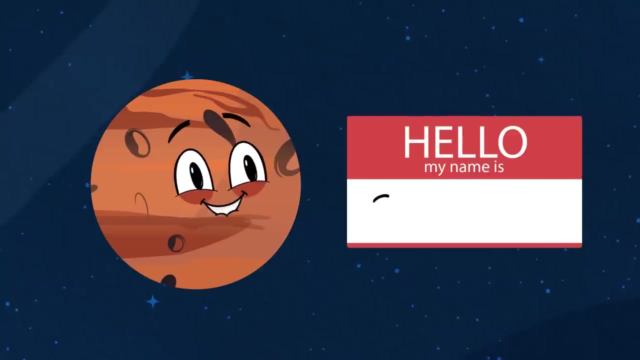 I'm an exoplanet orbiting the star Karo-7, you see, In the constellation of Monoceros. My name is Karo-7b 174567 Varda, Here to introduce myself. I have a provisional designation of 2003 MW-12. 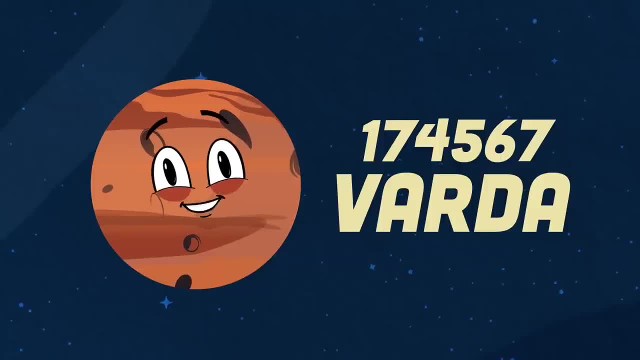 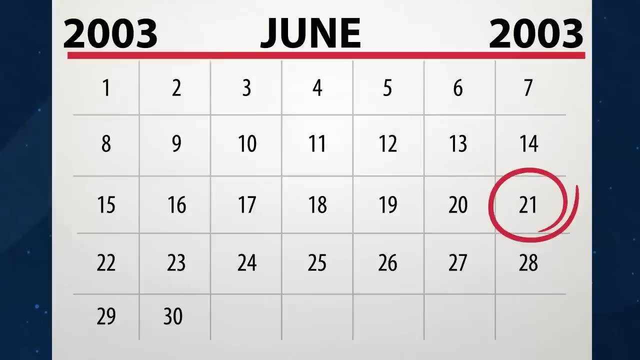 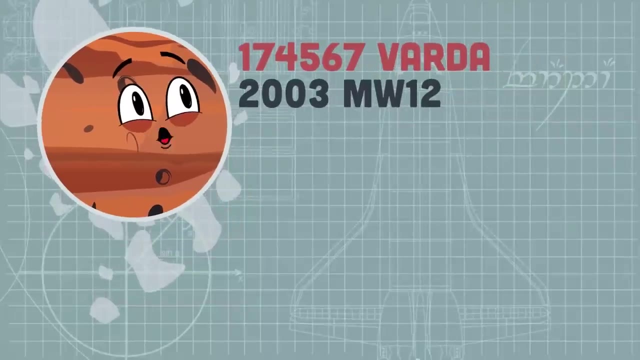 174567 Varda Here to introduce myself, A binary trans-Neptunian planetoid from the Kuiper Belt Discovered on the 21st of June in 2003. I was provisionally designated 2003 MW-12. you see The astronomer who discovered me on that day. 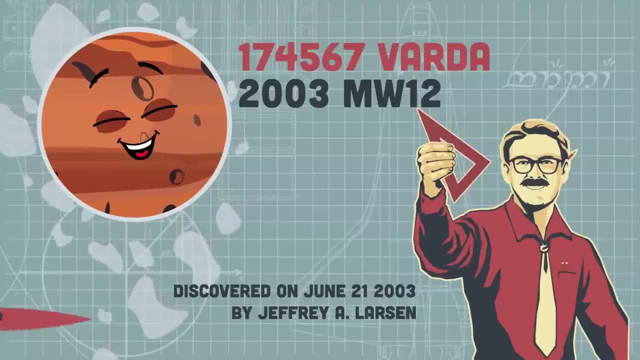 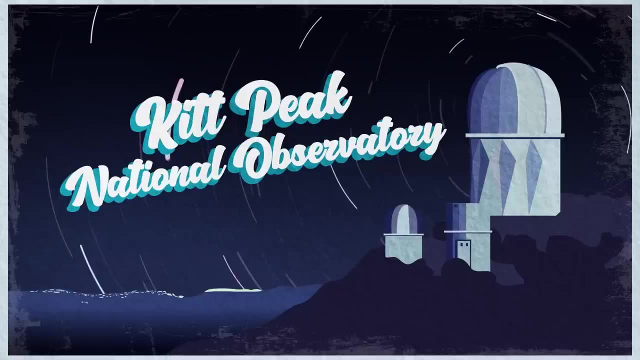 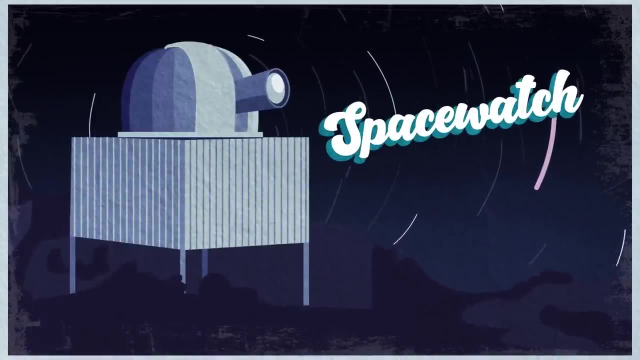 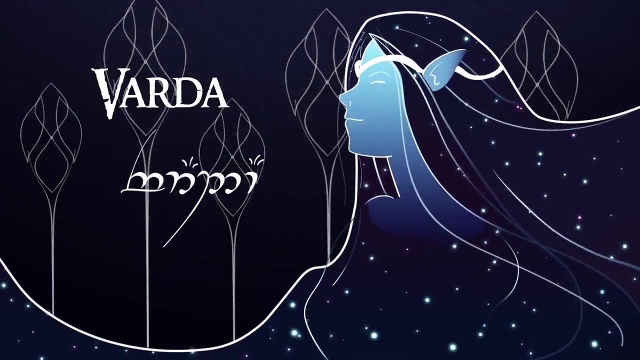 Is Jeffrey Larson. Now let's get on our way. I was discovered at the K-P-N-O, Which is the Kitt Peak National Observatory. Now, you know, The Space Watch Telescope Is what they used to see me, One of the major telescopes in the observatory. I was given the name of Varda in 2014. 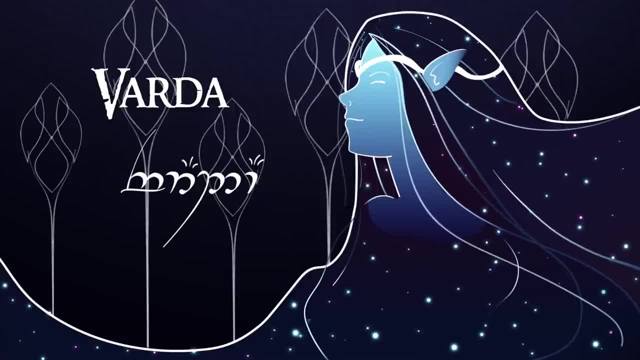 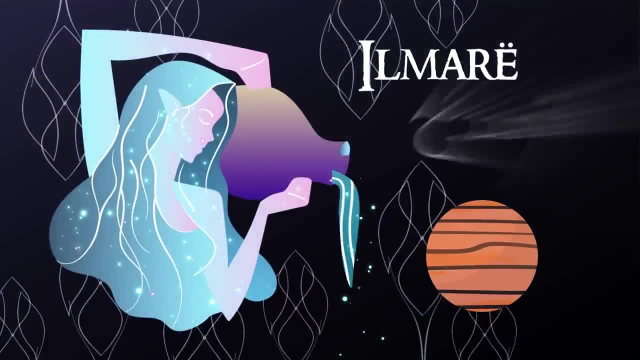 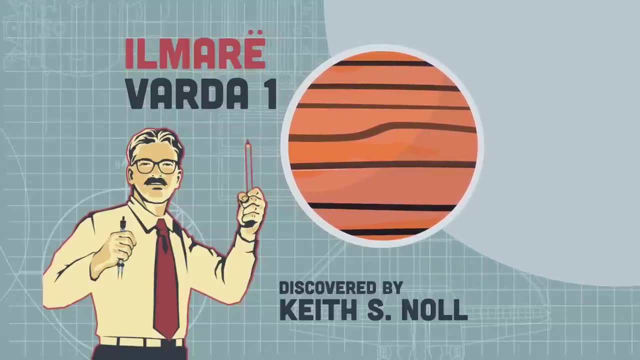 I've turned the creator of the stars And is the Valar Queen. Astronomers found one known satellite. It was named E-Mater Or Varda 1 on the night. It was discovered by Keith S Knoll, A planetary astronomer at NASA. you should know. 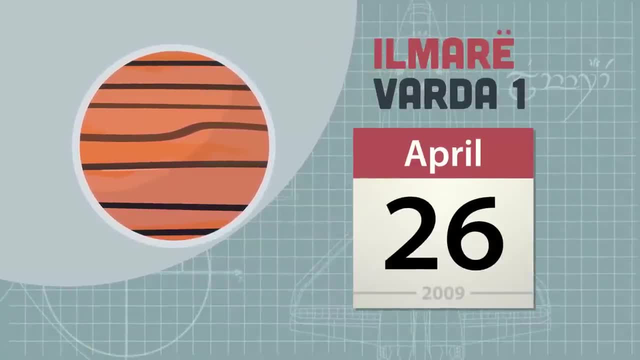 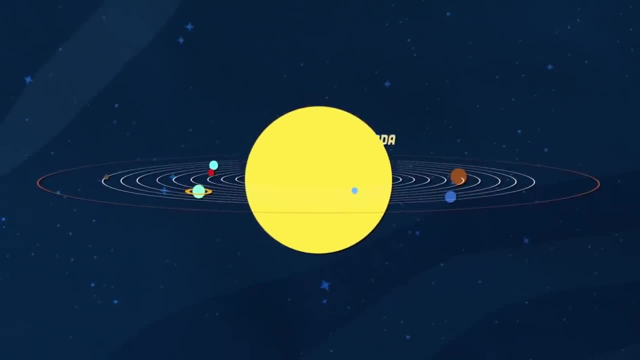 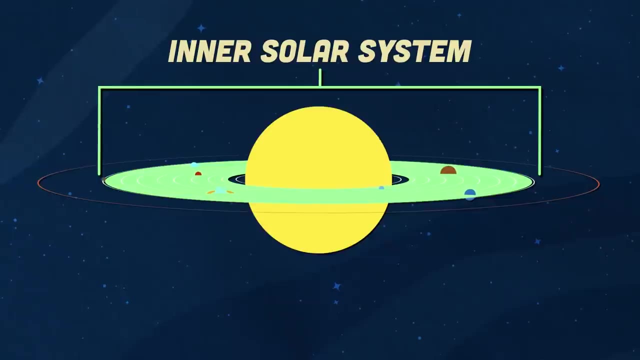 E-Mater was discovered in 2009, On April 26th, But I don't know the time Now. I take 313 years To orbit the sun And I will never enter the inner solar system. This orbit translates over 114,000 days In November 2096. 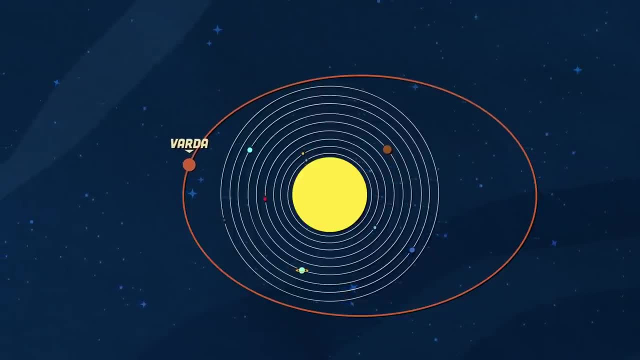 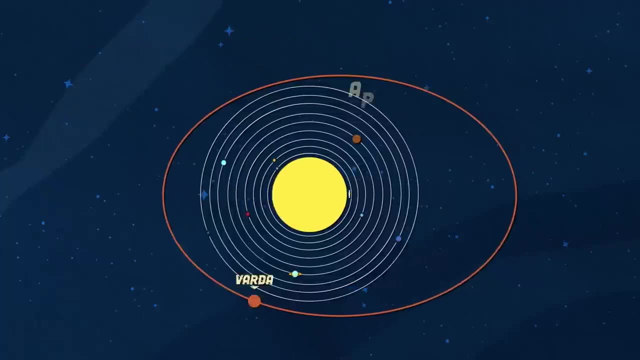 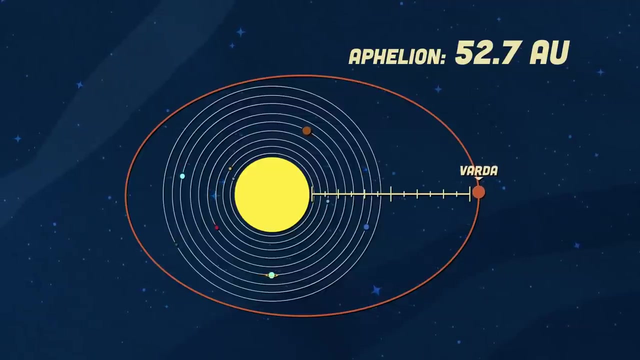 It's my perihelion's day. I'm a certain distance when I orbit the sun: 39.5 AU is my distance at perihelion. 52.7 AU is the distance of my aphelion. That's the furthest I orbit on my run round the sun. 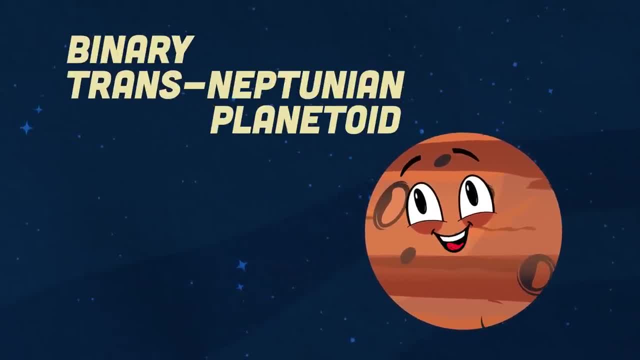 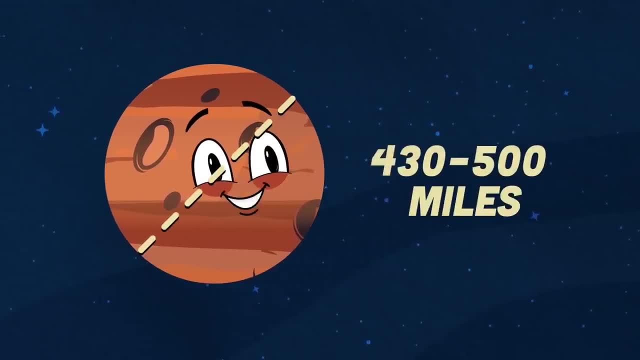 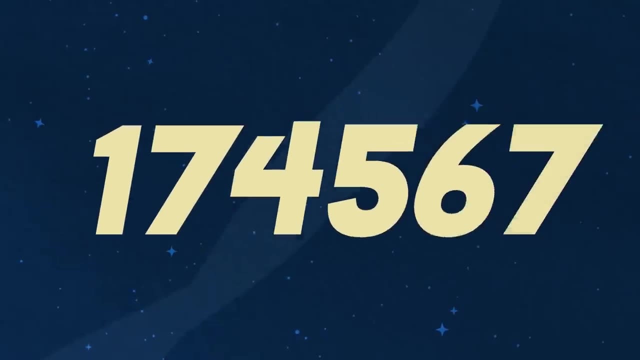 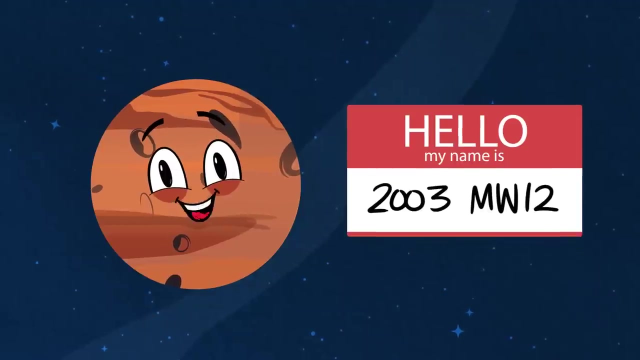 A binary trans-Neptunian planetoid fell Of the hot classical population in the Kuiper belt. I have a diameter of 432,500 miles. I'm still debated a dwarf planet all the while. 174567 Varda. here to introduce myself, I have a provisional designation of 2003 MW12. 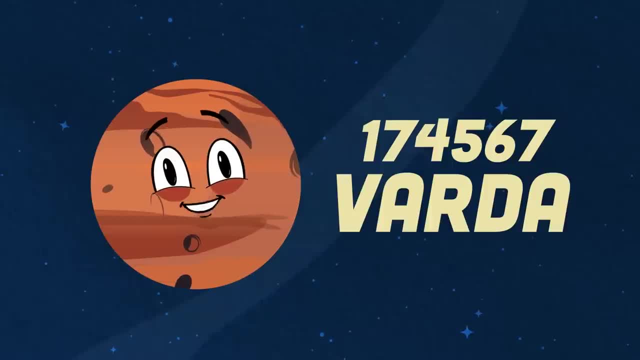 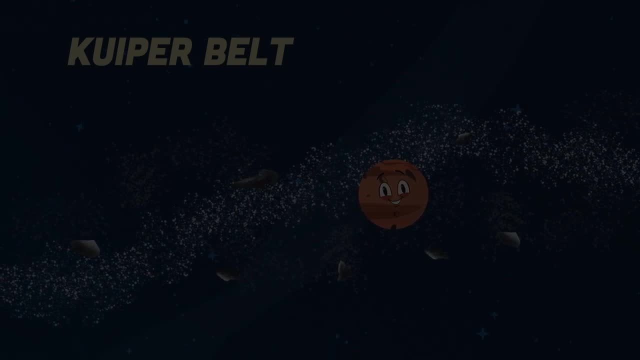 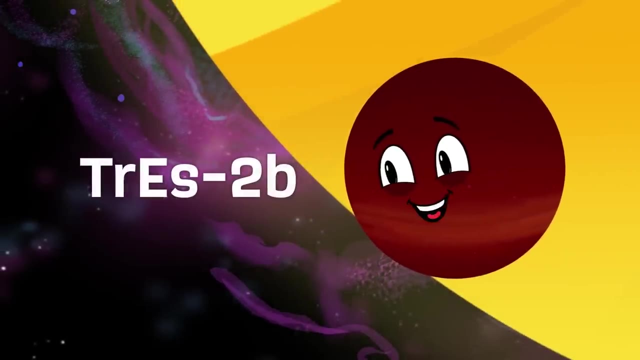 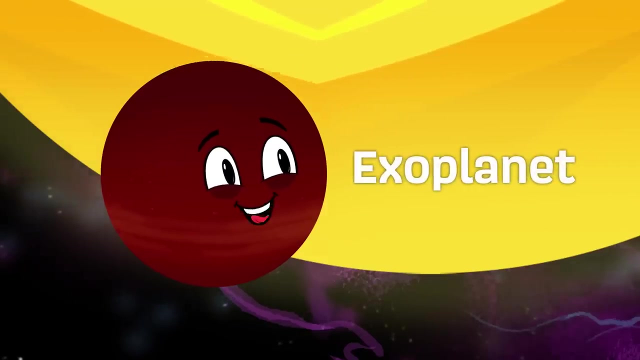 174567 Varda here to introduce myself, A binary trans-Neptunian planetoid From the Kuiper belt. My name is T-R-E-S-2-B. I'm a gas giant too far away to see. I'm the darkest exoplanet ever identified. 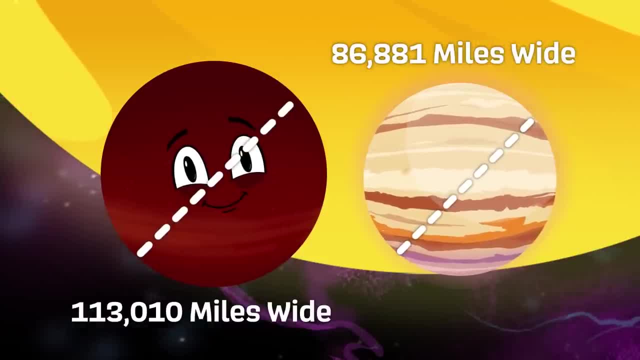 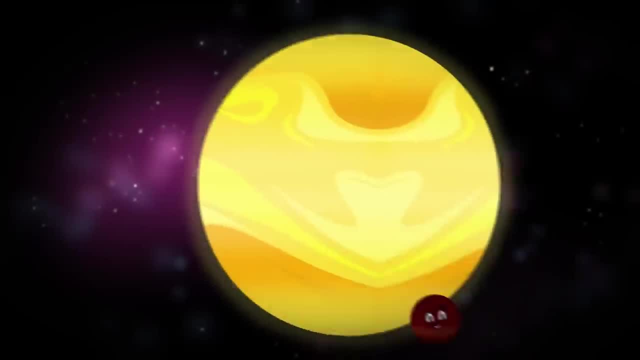 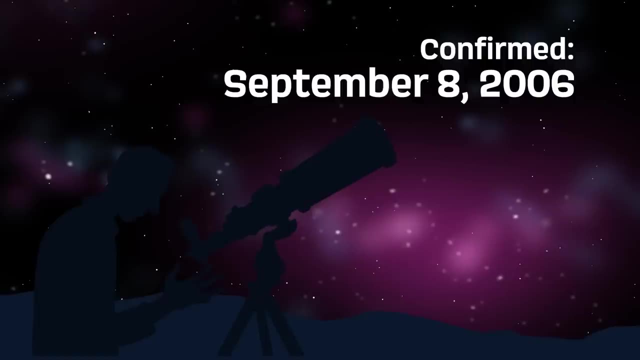 I'm a bit bigger than Jupiter. I'll describe With the discovery date of August 21st in 2006 Is when they noticed me at first. I was confirmed a planet. on September 8th In 2006, officially my birthday, I was discovered by an astronomer. 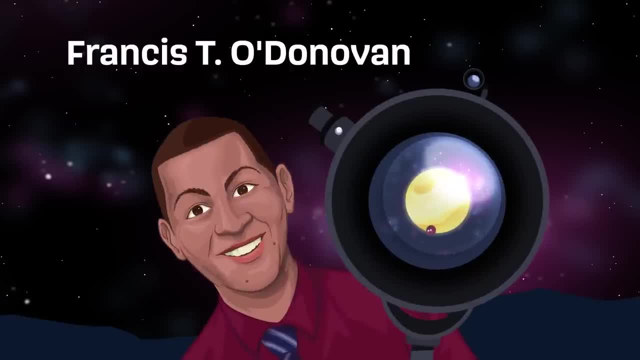 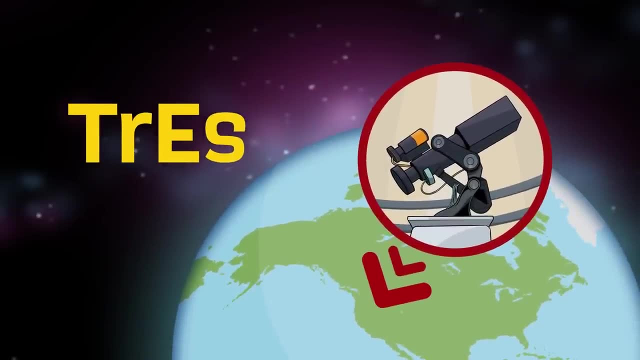 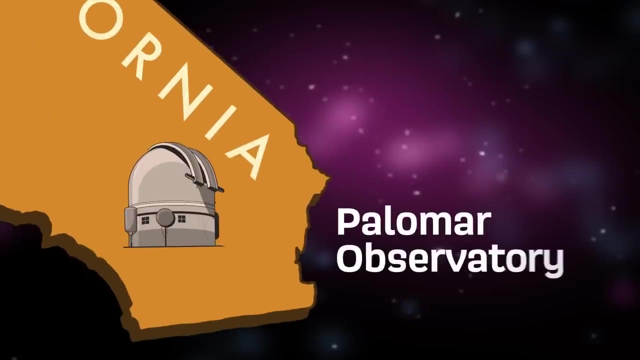 Named Francis T O'Donovan, That is for sure. First seen on the Transatlantic Exoplanet Survey, Or you could call it TRES, It's an acronym I say This all happened in California, You will see, At the famous Polymer Observatory. My discovery also took place at the Low Observatory. 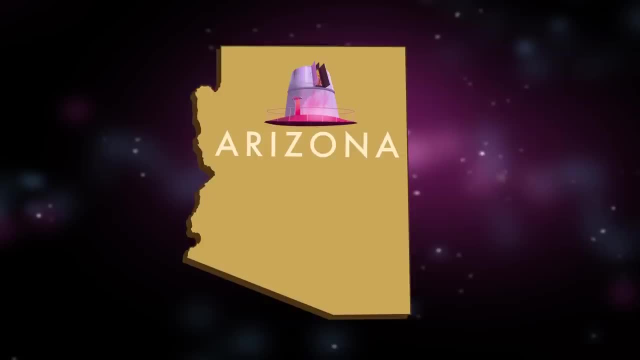 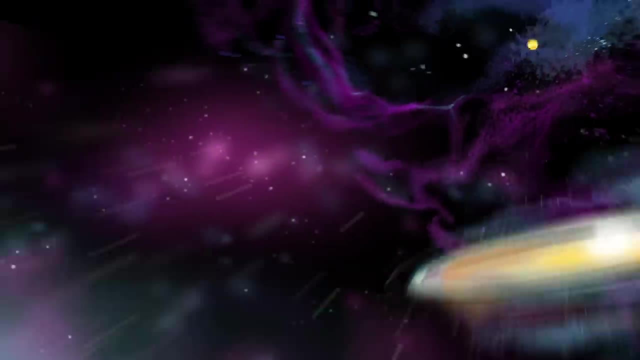 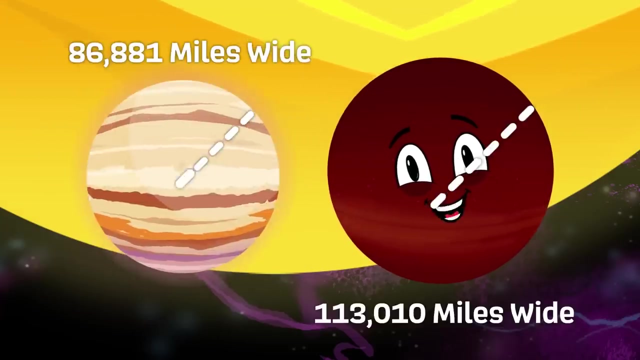 Located in Arizona. Now here's more about me. My name is T-R-E-S-2-B. I'm a gas giant too far away to see. I'm the darkest exoplanet ever identified. I'm a bit bigger than Jupiter. I'll describe GSC 03549-02811. 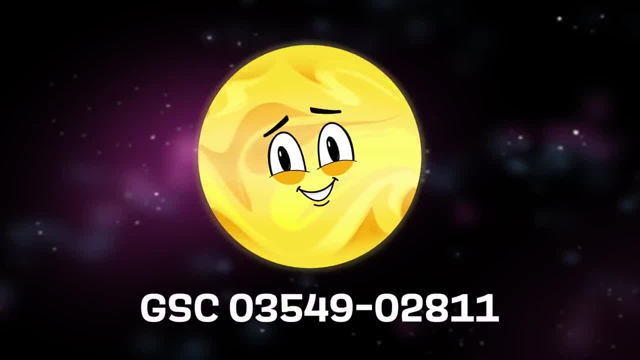 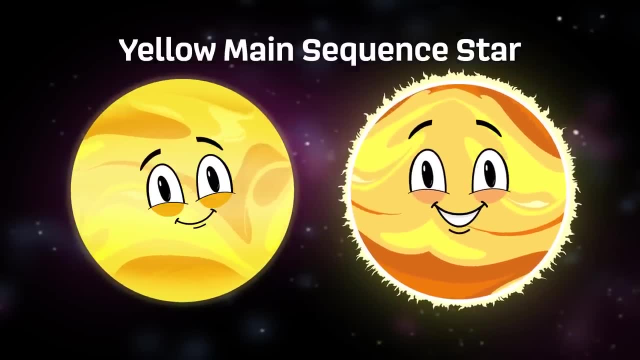 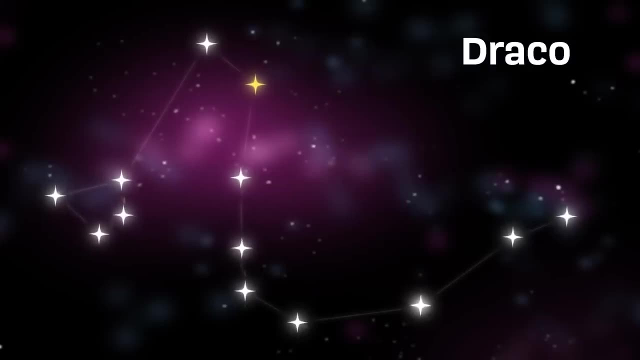 Is the star that I orbit, And a long named one. My parent star is a yellow main sequence star, Similar to your sun. Just to keep you on par, I belong to a constellation In the far northern sky. Its name is Draco, which is Latin for dragon, I imply. 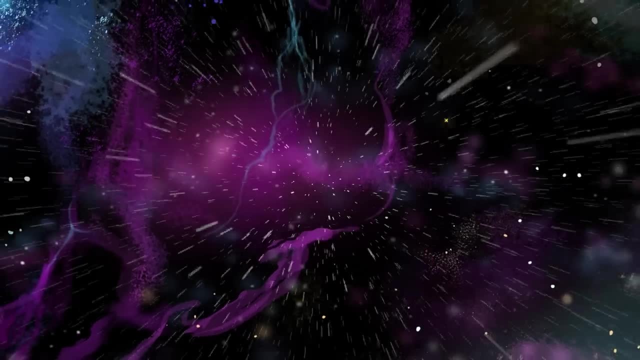 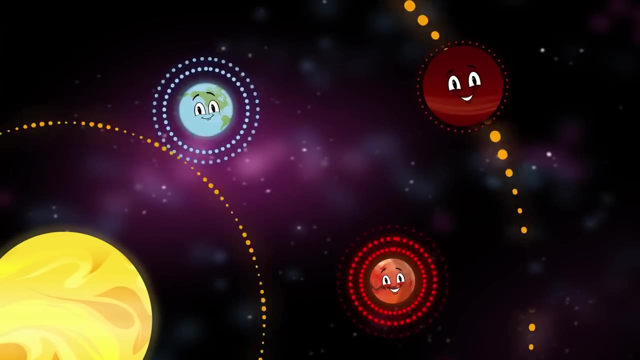 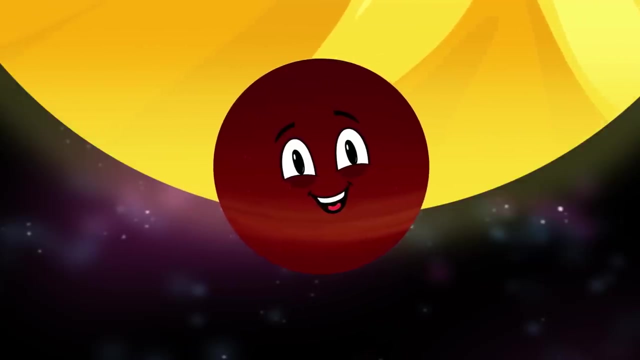 I'm 750 light years away From your solar system. That's where I'll stay. I'm thought to be the darkest known exoplanet, Reflecting less than 1% of any life that does hit. My mass, and radius does indicate I'm a gas giant with a bulk composition similar to Jupiter. 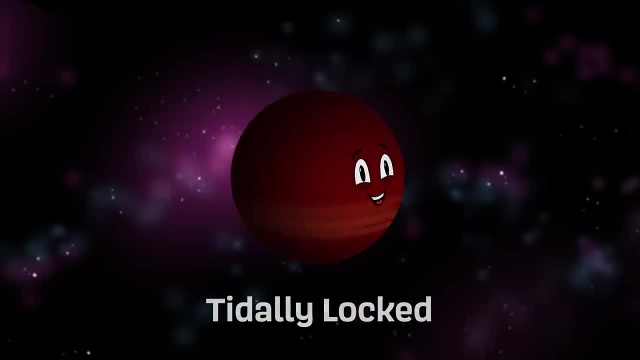 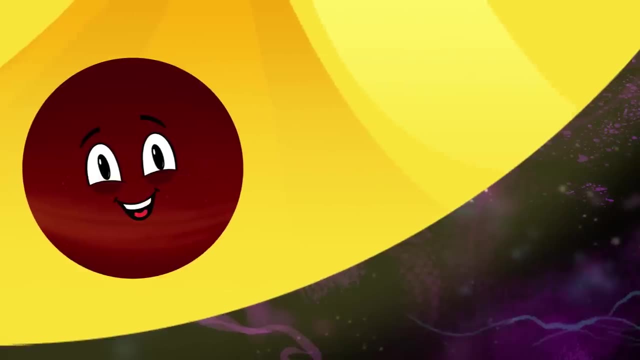 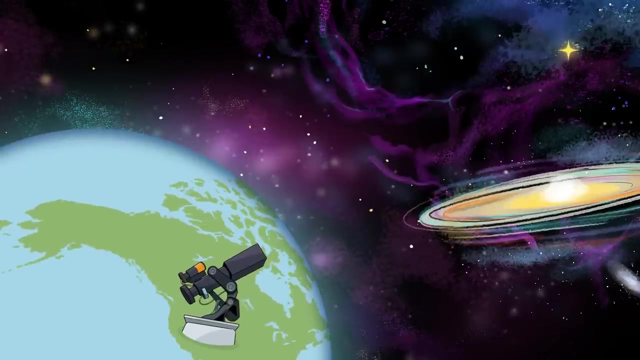 You're super giant. I'm likely to be tidally locked to my parent star. I'm extremely dark and completely bizarre. My name is T-R-E-S-2-B. I'm a gas giant too far away to see. I'm the darkest exoplanet ever identified. 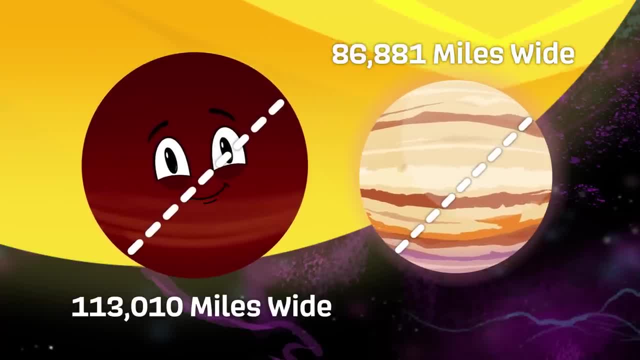 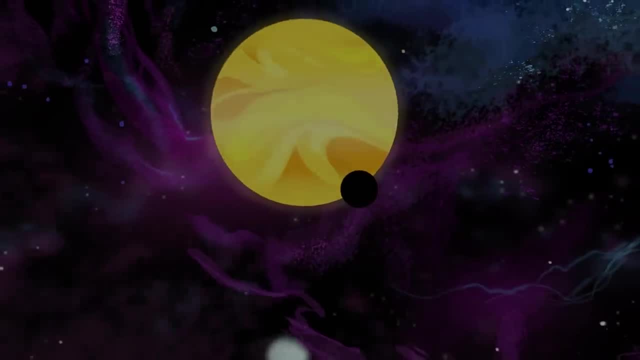 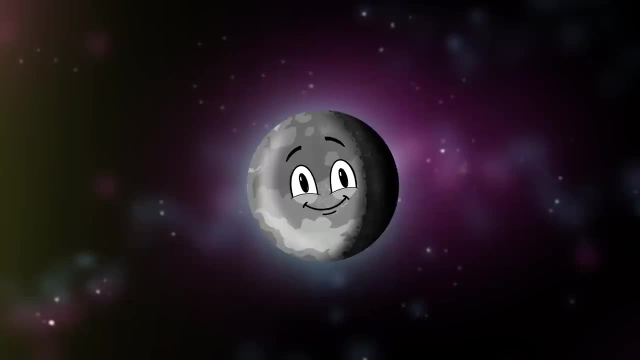 I'm a bit bigger than Jupiter. I'll describe. GSC 03549-02811 Is the star that I orbit And a long named one. GSC 03549-02811 Is the star that I orbit. I'm extremely dark and completely bizarre. I'm an extrasolar planet called Kepler 37b. 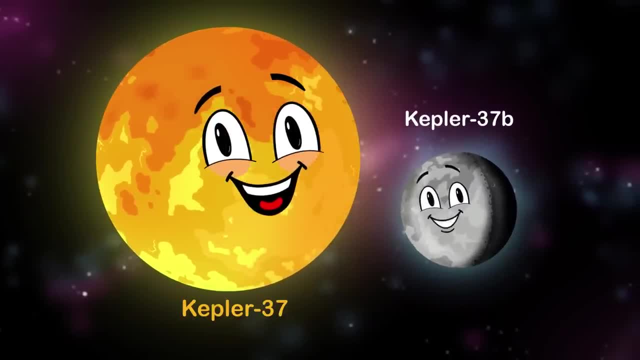 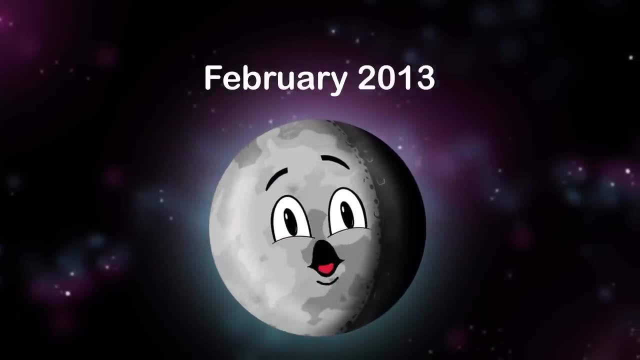 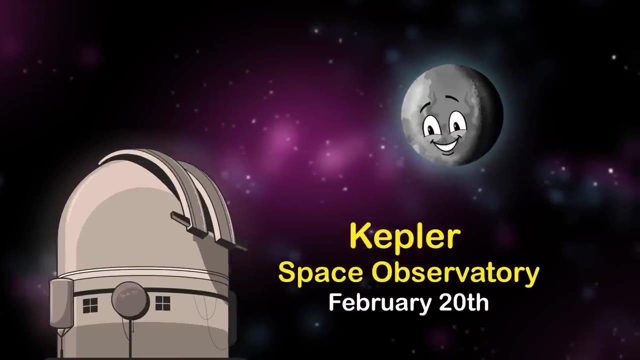 Orbit in Kepler 37. that's my host RUC. I was discovered in the month of February in 2013. Now let's learn more about me. My discovery site is Kepler Space Observatory. On the 20th in the month of February, The Kepler Space Telescope did make my discovery. 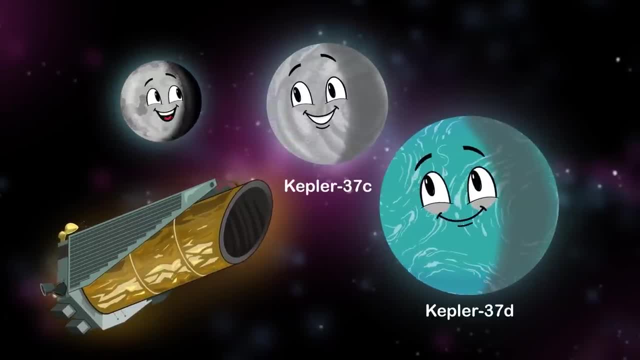 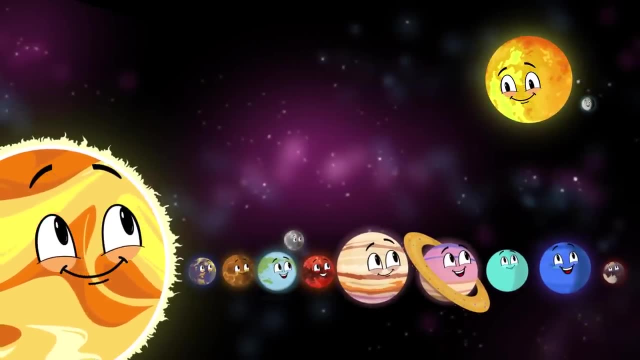 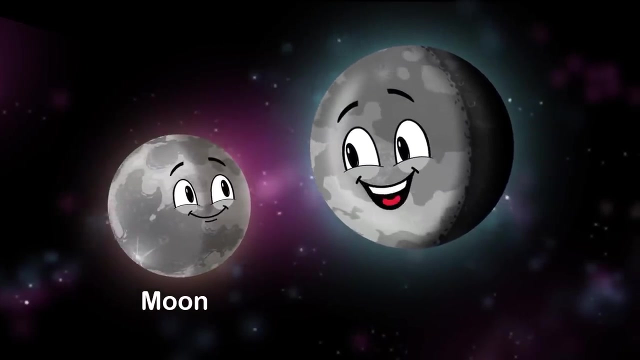 Along with two other planets, Kepler 37 C and D. To date, I am the smallest planet discovered around. I made sequence star outside the solar system I am found. I have a radius slightly bigger than your moon, But I'm slightly smaller than Mercury. You've learned this in this tune. 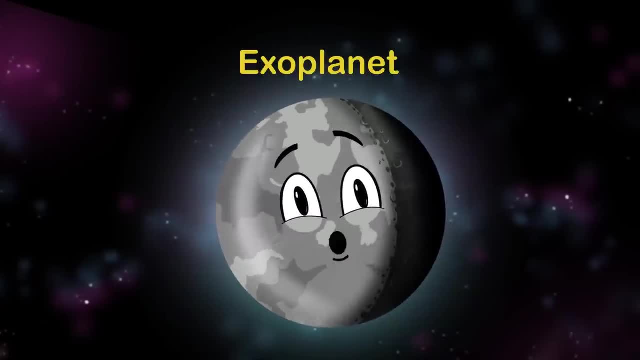 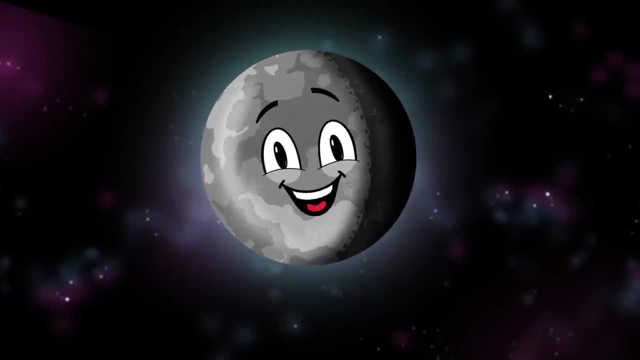 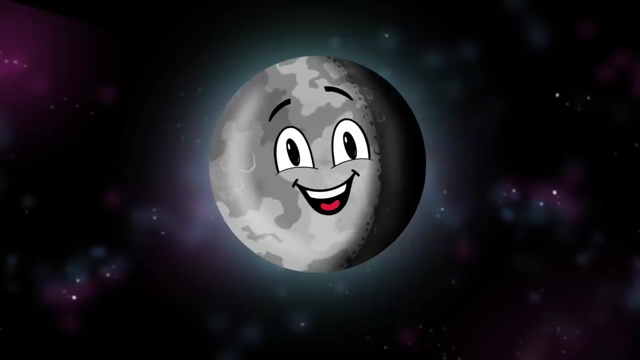 I'm classified as an exoplanet, also ace of Earth. This means that I'm substantially less massive than Venus and Earth. I'm an extrasolar planet called Kepler 37b Orbit. in Kepler 37 that's my host, RUC. I was discovered in the month of February in 2013. 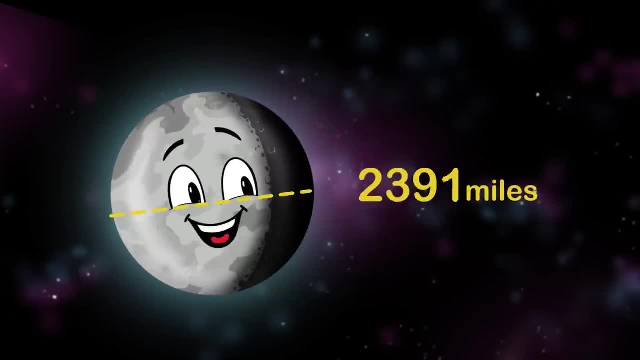 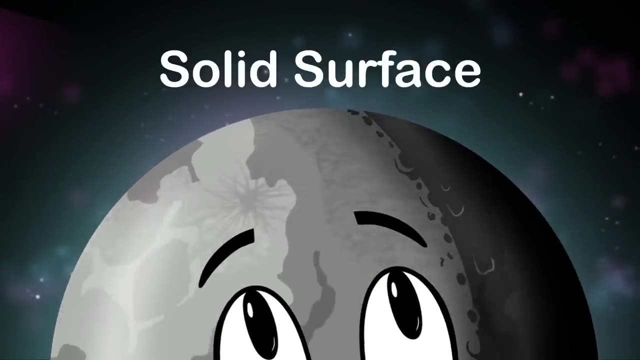 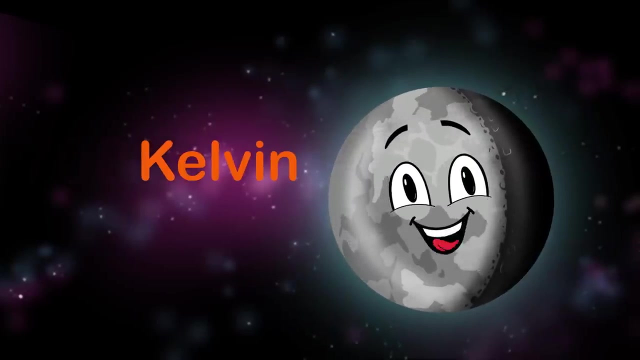 Now let's learn more about me. I do have a diameter of 2400 miles. I'm likely a rocky planet with a solid surface, though I have a surface temperature around 700 K. The K does mean Kelvin in the International System of Units. today I orbit my G star. it's called Kepler 37. 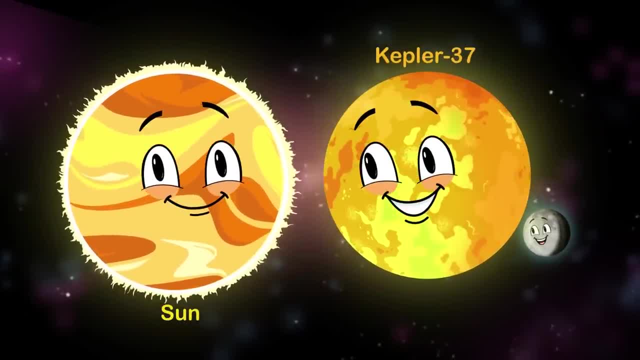 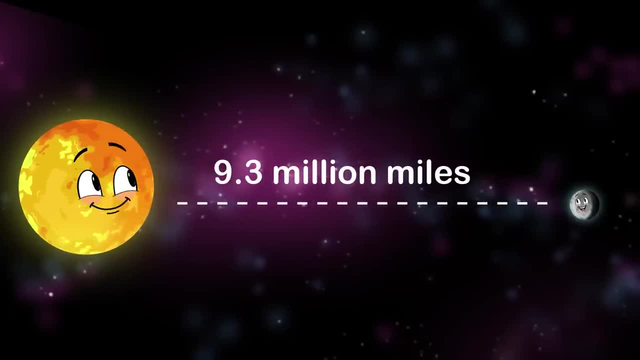 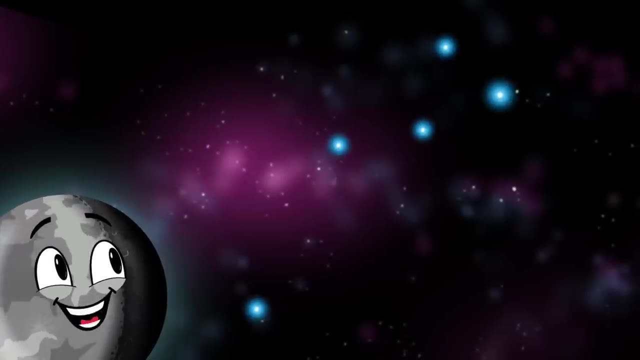 Here. it's similar to your Sun, as you can see when it did appear. I orbit my parent star at 9.3 million miles away, With an orbital period every 13 days. If you're looking for me in the dark of the night sky, You can find me in the constellation Lyra. please stop by. 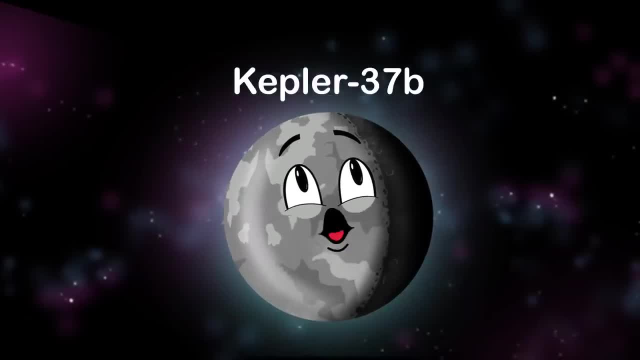 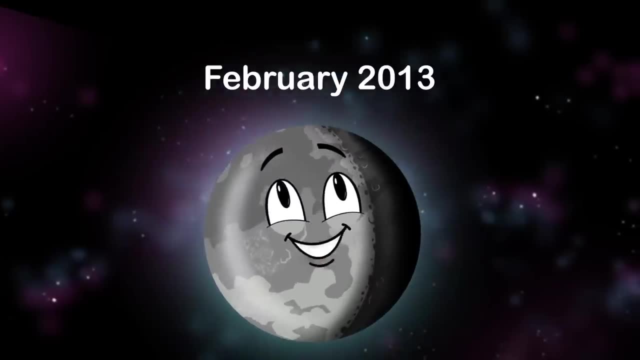 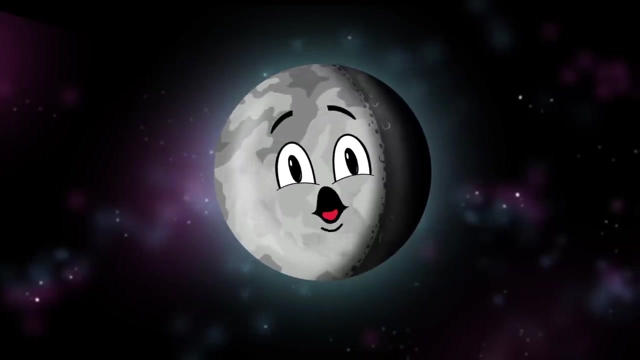 I'm an extrasolar planet called Kepler 37b. Orbit in Kepler 37. that's my host, RUC. I was discovered in the month of February in 2013. Now let's learn more about me. I'm an extrasolar planet called Kepler 37b. 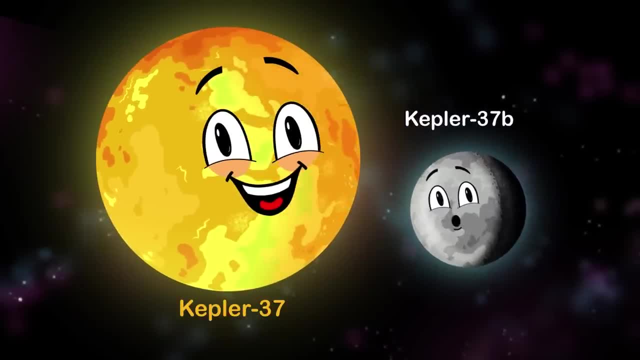 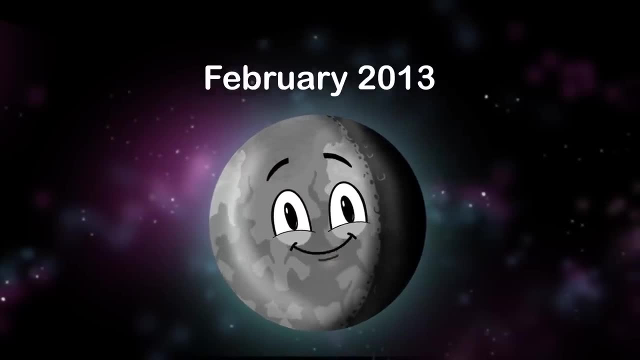 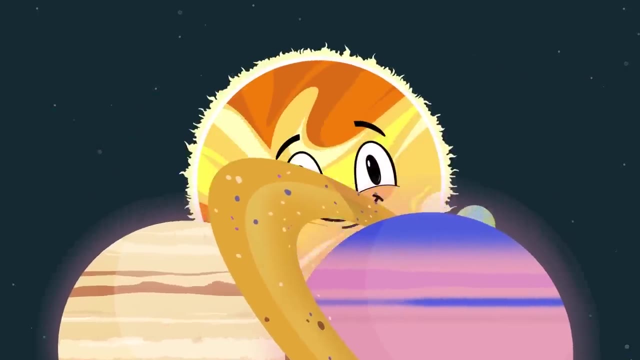 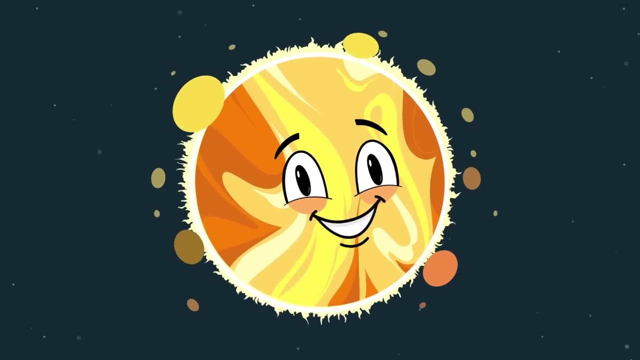 Orbit in Kepler 37. that's my host RUC. I was discovered in the month of February in 2013. Now let's learn more about me. I am the Sun, the center of your solar system. I do erupt intense, high energy radiation. This radiation I expel is called the solar flare. 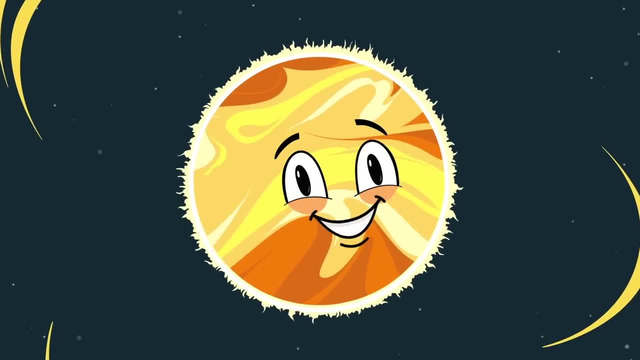 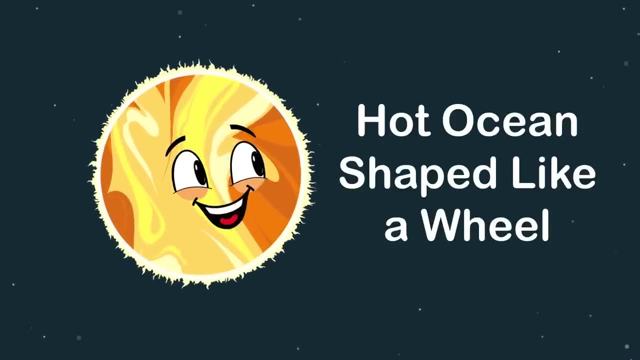 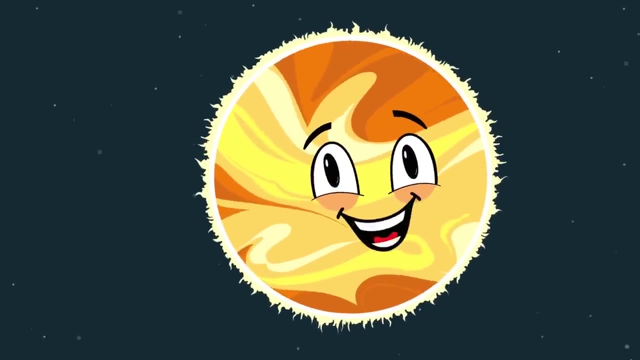 You'll learn about them in this song and why you should care. The Sun is a ball of plasma like an extremely hot ocean shape Like a wheel. This plasma is pushed around in shape by the Sun's magnetic field. When the Sun's plasma swirls around by its magnetic field, 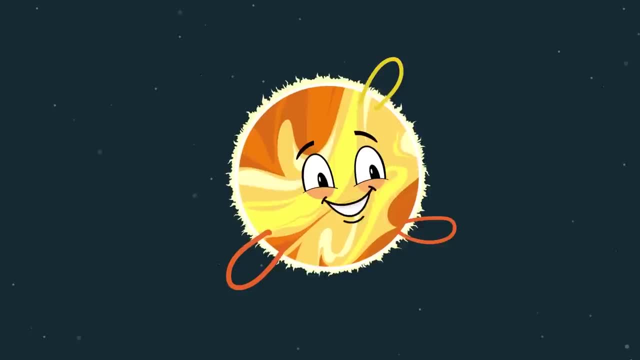 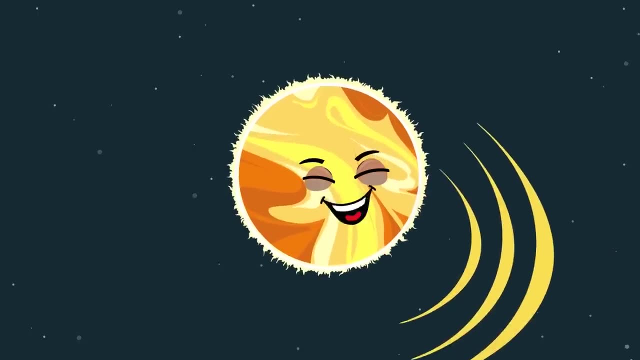 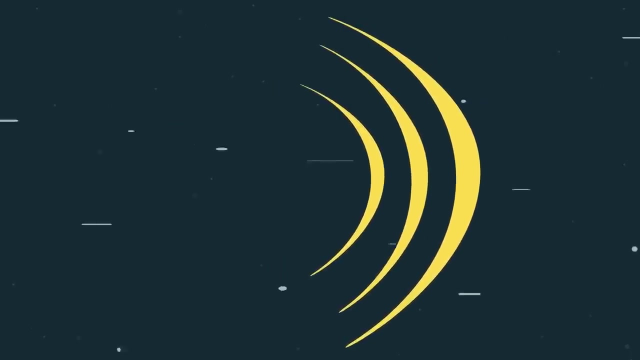 It gets twisted and releases energy around sunspots. they are real. This energy released is caused by magnetic knots. When one of these knots breaks, It releases solar flares. so you are taught. Solar flares are waves of high energy radiation Shot through the solar system in which we are all one. 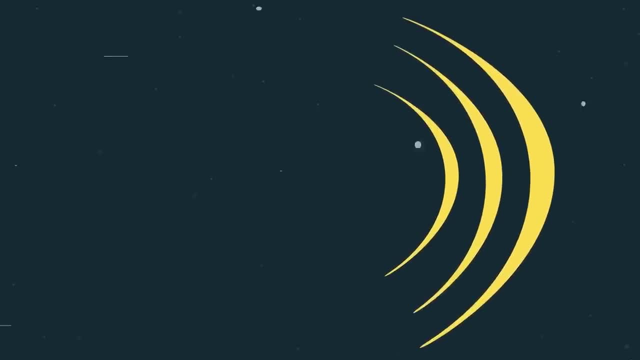 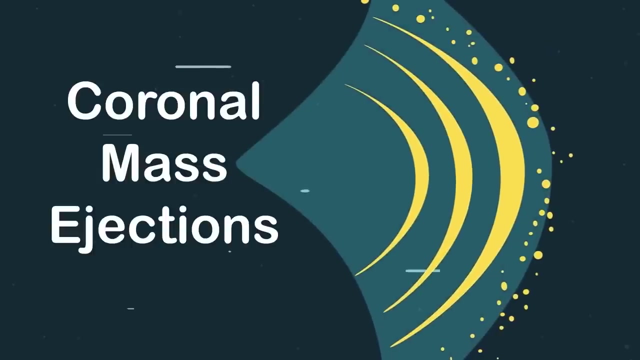 These solar flares race through space At the speed of light, Creating a solar proton storm. These storms are no delight. When millions of tons of plasma are thrown from the Sun's atmosphere, These storms are called Chlorinal mass ejections. as you see right here, These CMEs reach speeds of 5.6 mmph. 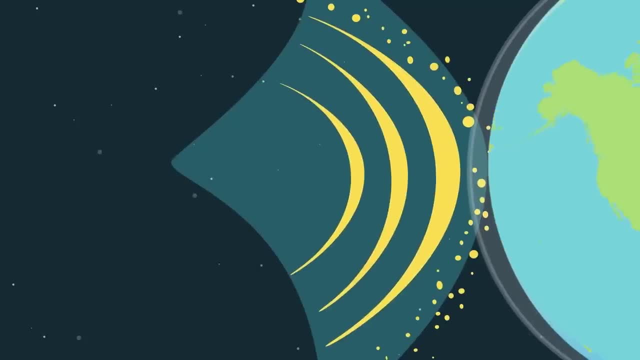 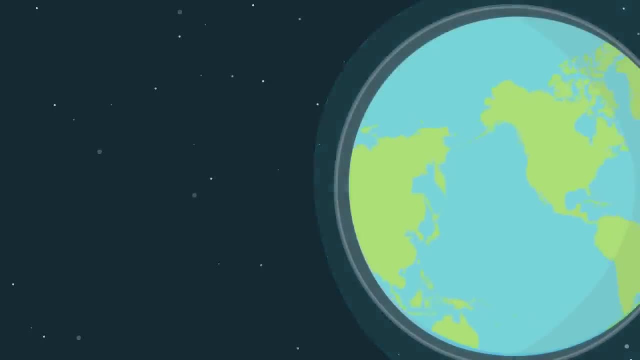 When they hit Earth, it doesn't hurt living beings. even with such power, The Earth's atmosphere protects life from the biggest solar storm- The biggest solar storms- by absorbing the impact, So beings on the surface are safe from harm. When a CME is too big, it creates a solar super storm. 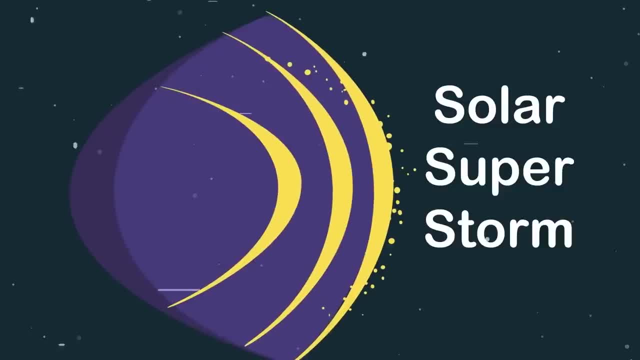 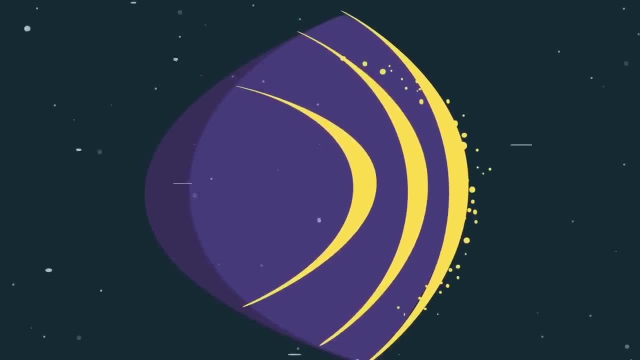 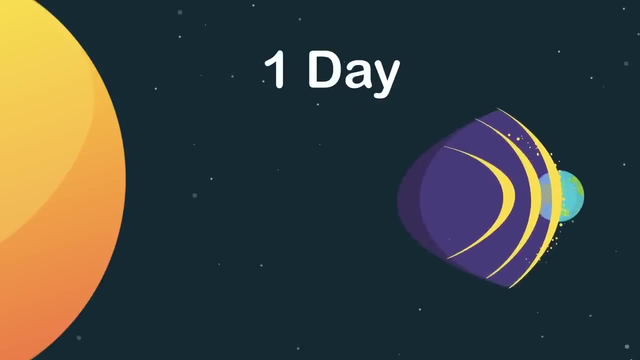 That occur once or twice a century. so you've been warned. If a solar super storm did happen in this day and age, It would shoot billions of tons of plasma from the Sun. I do say If this type of CME traveled across space towards the Earth, It would reach you in one day. 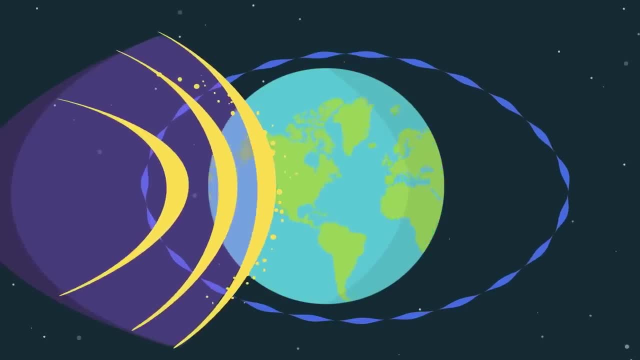 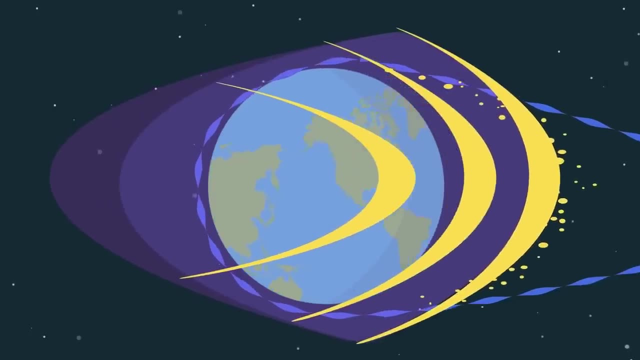 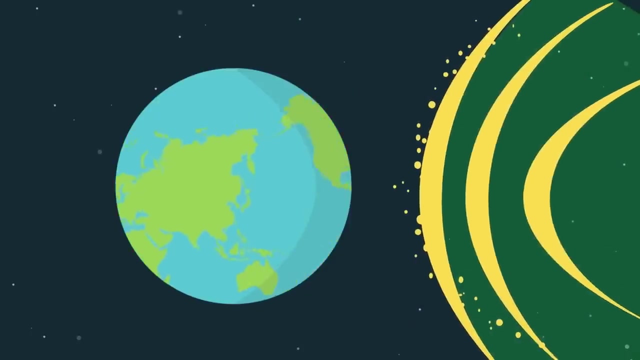 Yeah, that's fast. But what that is worth? Its shock wave would compress Earth's magnetic field, making it frail. The two magnetic fields would merge, stretching Earth's field into a thin tail. This stretched tail can't contain this energy anymore. When it snaps, it releases explosive energy towards the Earth that it stored. 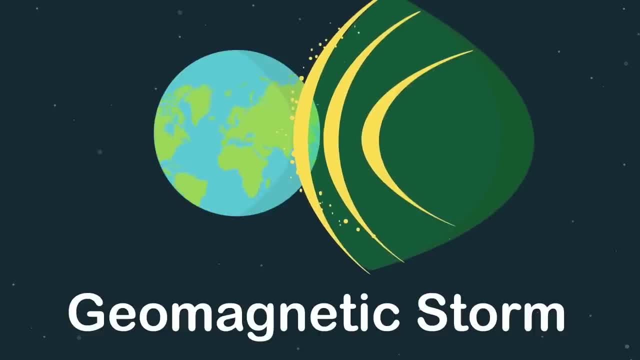 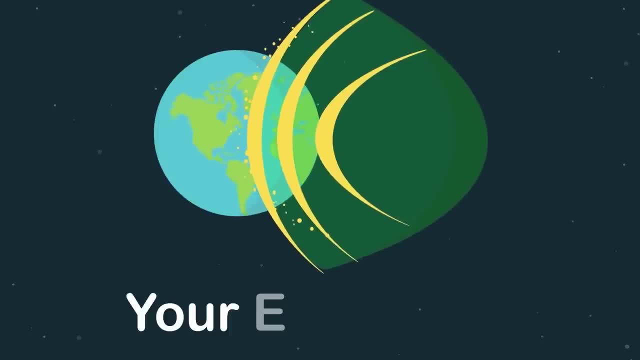 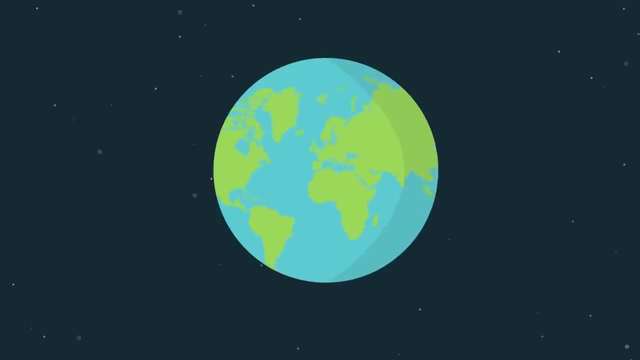 This creates something very rare called the geomagnetic storm. Normally, no living thing on Earth would even know it had formed. The only thing it would affect Is your electricity, Because you rely on this so much. it would disrupt human life, you see, Because Earth is covered in millions of electric wires and transformers. 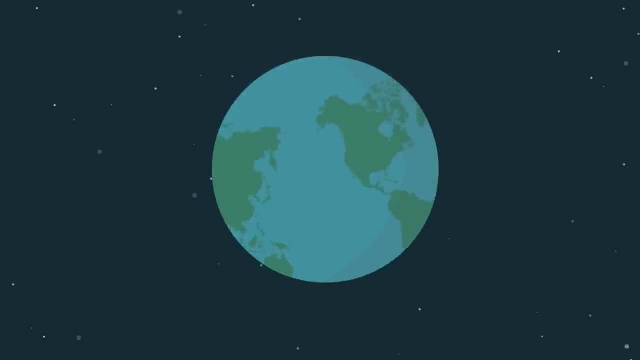 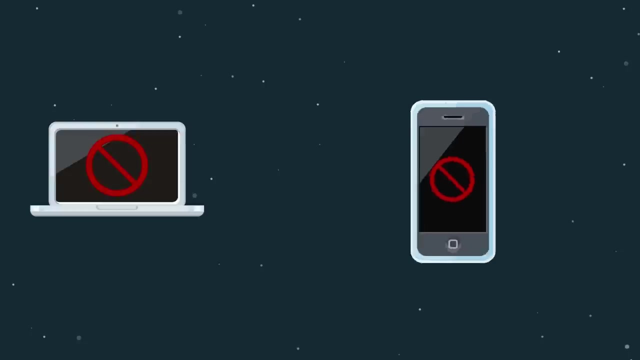 This geomagnetic storm would shut down the power. Humans would be overturned. If one of these storms hit the Earth, electricity and internet would not work. All things powered by electricity would turn off, along with all networks. Computers wouldn't work, along with phones and electronic devices. No refrigerators or any other house. 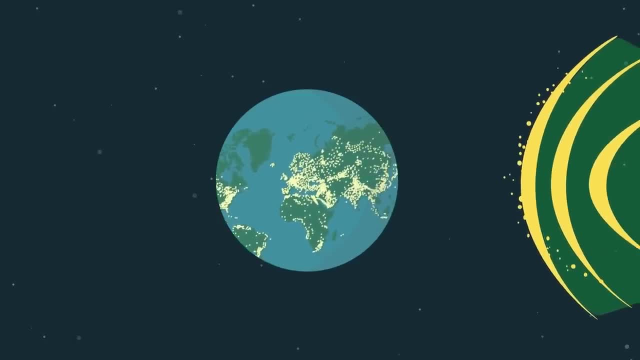 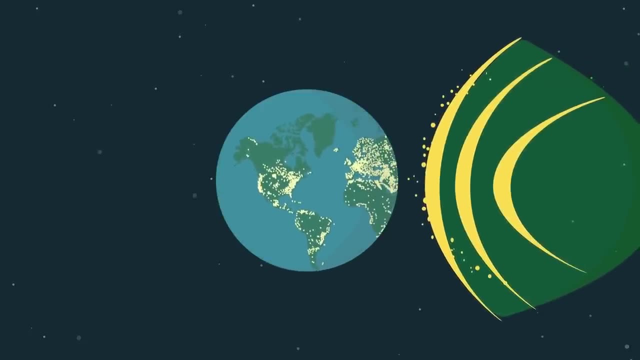 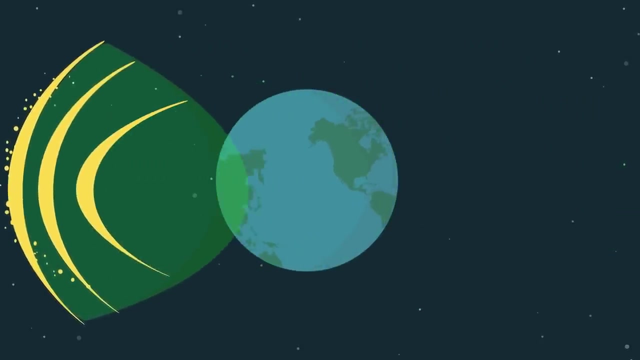 No household appliances. Even though we can't stop these terrible solar storms, Their nasty side effects can be prevented by how we are warned. Engineers would have a day or two to unplug major power grids Until the solar storm passes Earth, preventing blackouts. we forbid Humans need to prepare for these types of storms. 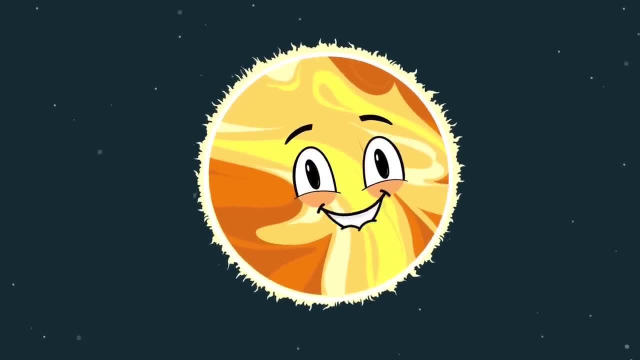 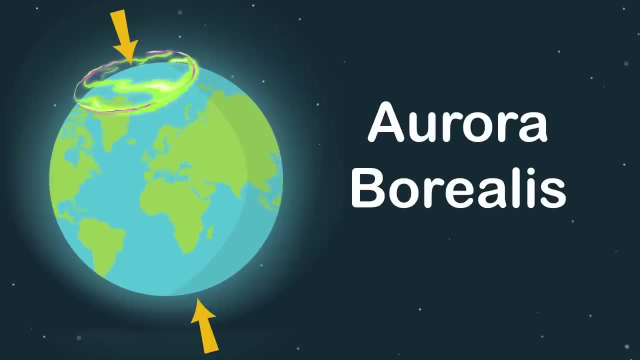 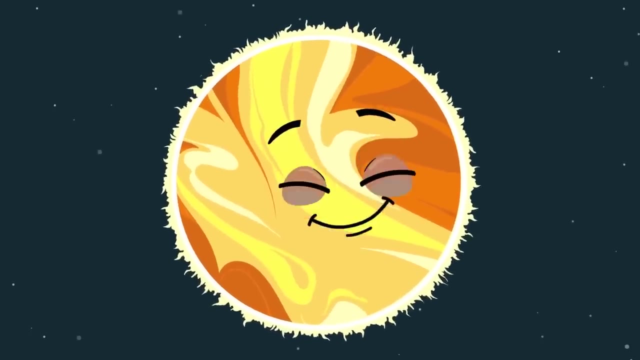 To prevent being thrown back to the stone age before they form. A cool event humans experience from any solar storm Is the aurora borealis at the two poles is where they perform. I'm the life giving sun. you all need me to live, But I am unpredictable. so solar storms I give. 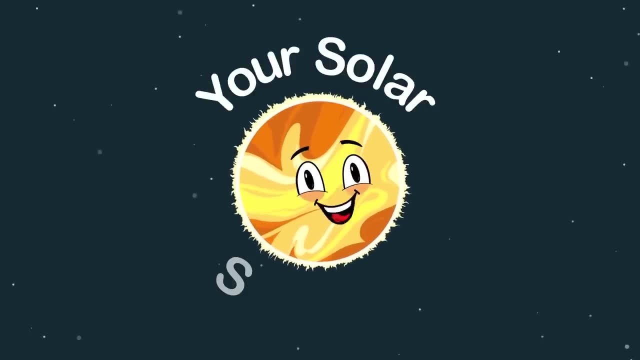 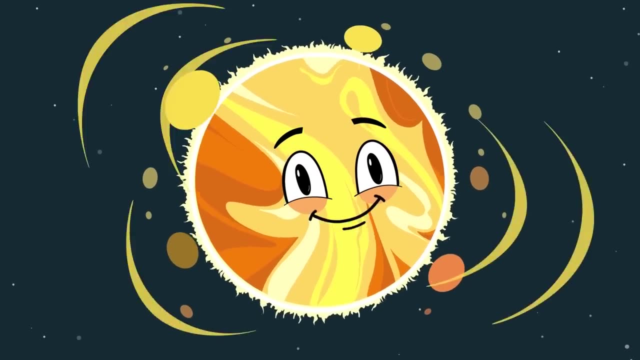 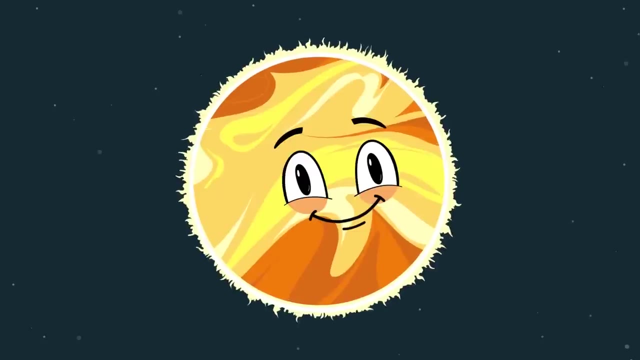 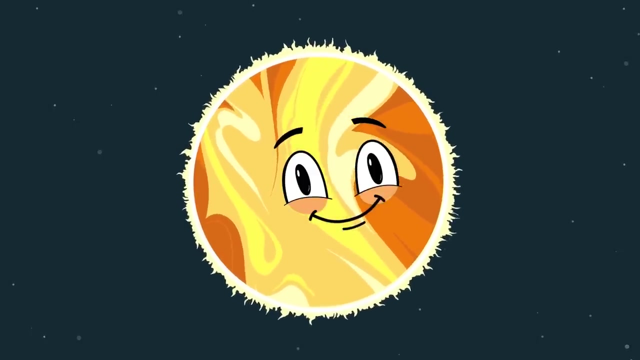 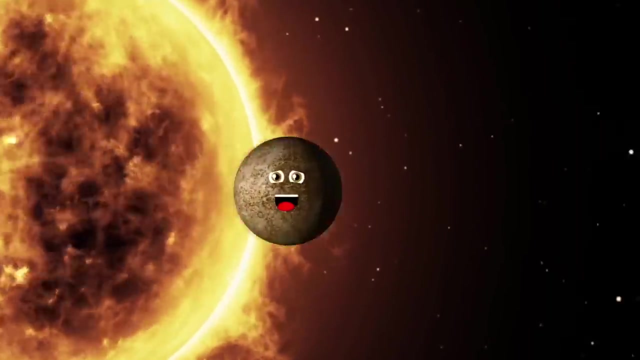 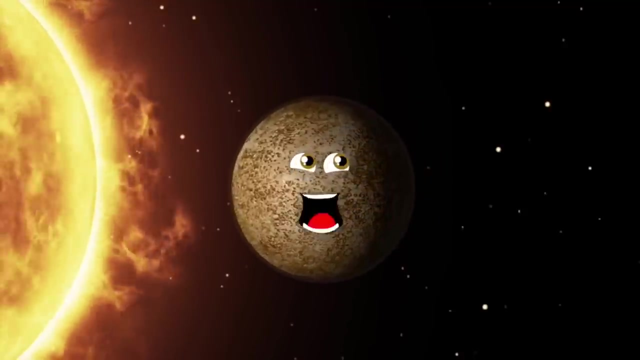 I am the sun, the center of your solar system. I do erupt intense, high energy radiation. This radiation I expel is called the solar flare. You'll learn about them in this song and why you should care. I am the first planet from our sun. you see, My name is Mercury. nothing orbits faster than me. 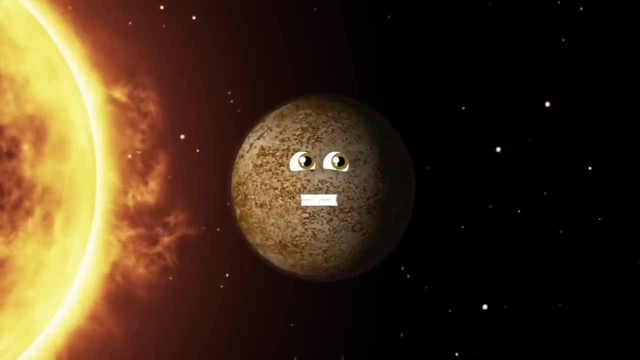 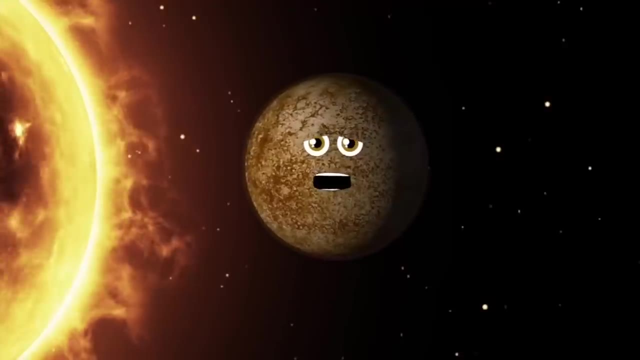 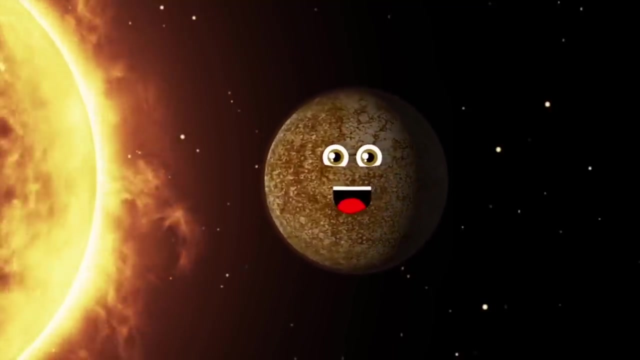 The smallest planet with the second hottest degree. My name is Mercury. No one is smaller than me. Messenger of the gods is what Mercury means. The Romans gave me my name Cause I'm the fastest they'd seen. A bit bigger I'd be than the Earth's moon. that you see. 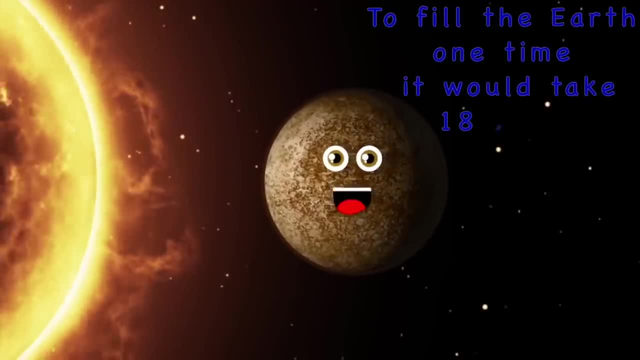 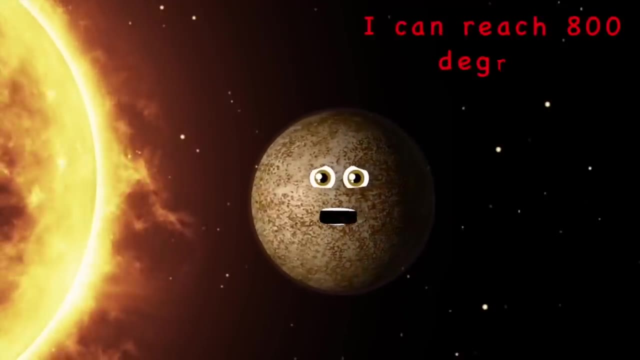 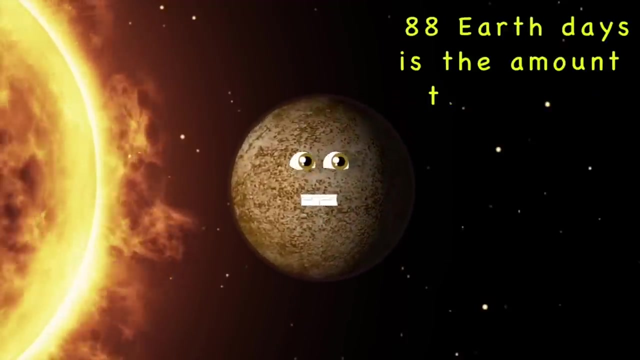 To fill the Earth one time it would take 18 of me. I am the first planet from our sun that beams, But I'm the second hottest. I can reach 800 degrees. 88 Earth days is the amount that I take To orbit our sun once. that makes one year on me. 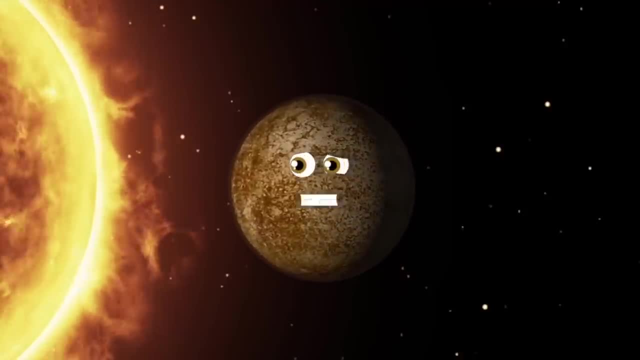 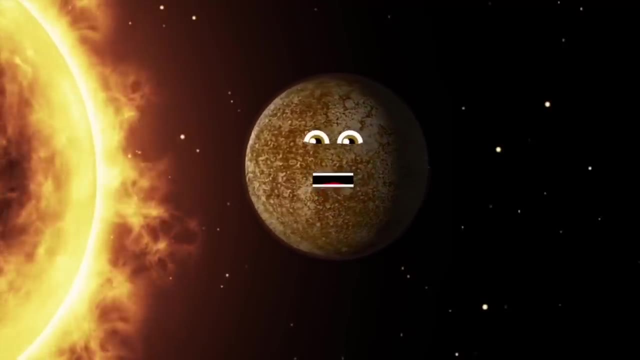 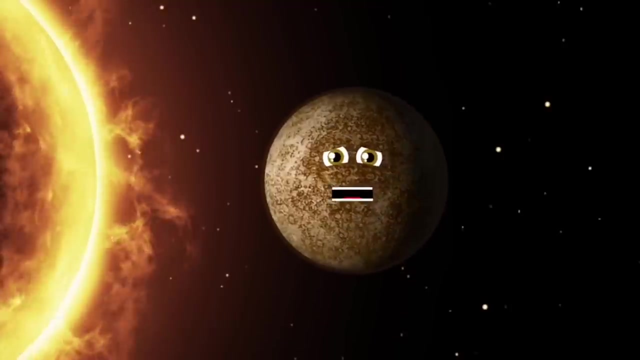 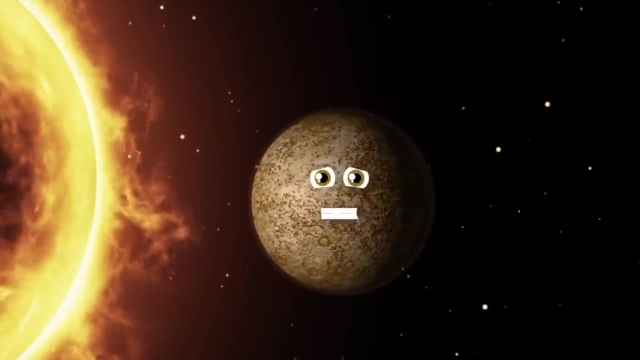 I am the first planet from our sun. you see, My name is Mercury. nothing orbits faster than me. The smallest planet, with the second hottest degree. My name is Mercury. no one is smaller than me. 59 Earth days equals one day on me. My surface is made of stone covered in craters, you see. 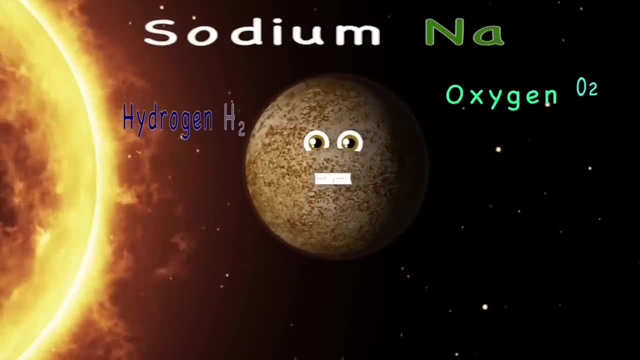 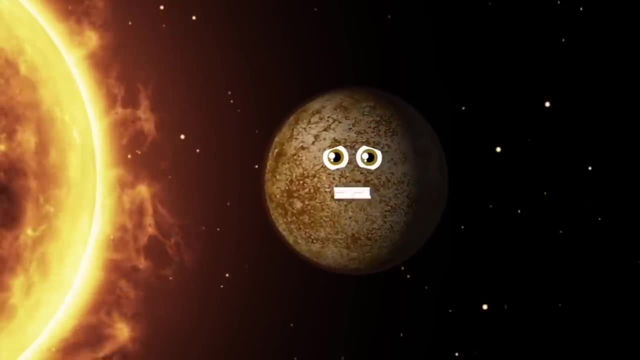 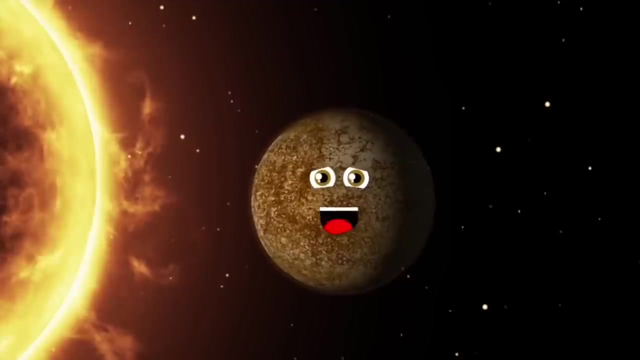 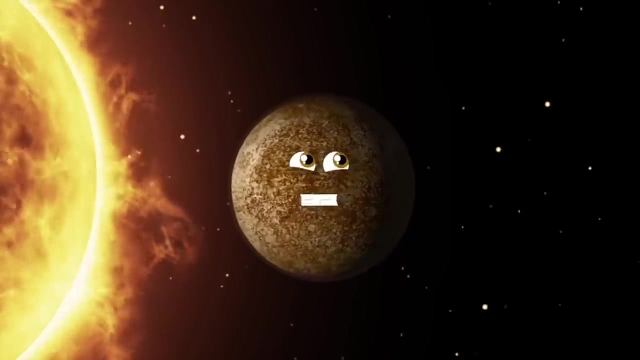 Oxygen, sodium, hydrogen, helium and potassium Make up my exosphere. I have no moons and I have no rings, But I'm the second densest planet. amongst other things, I am the first planet from our sun. you see, My name is Mercury. nothing orbits faster than me. 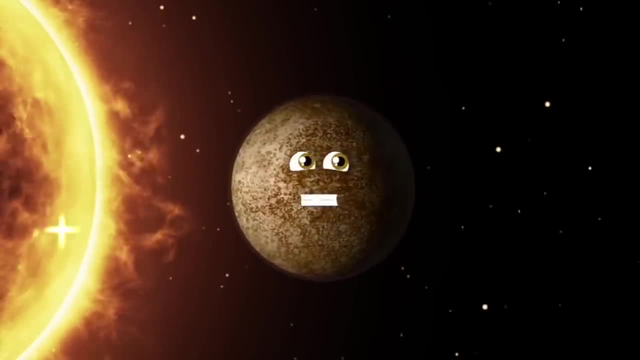 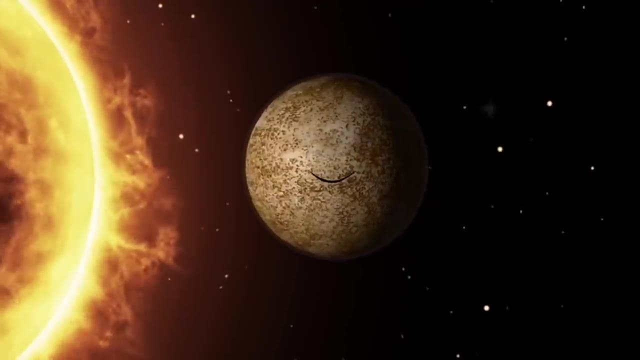 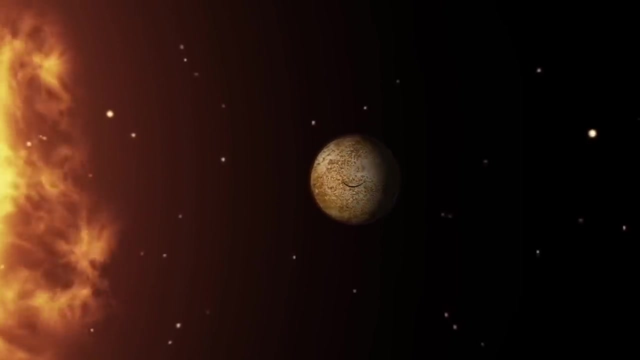 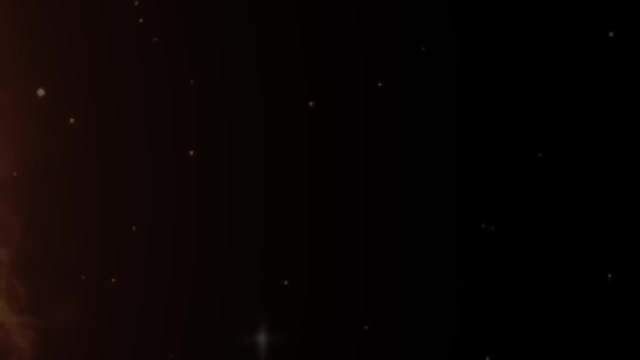 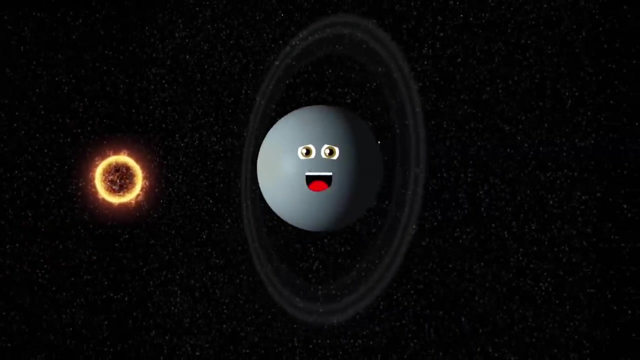 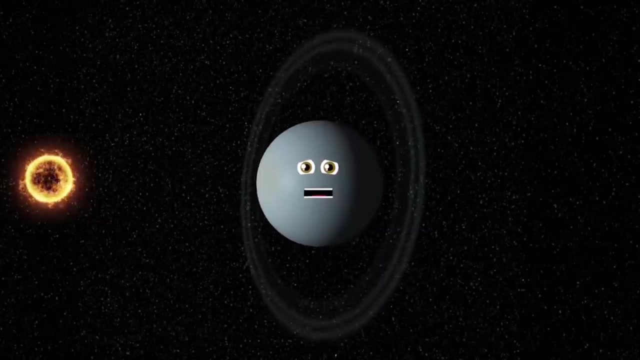 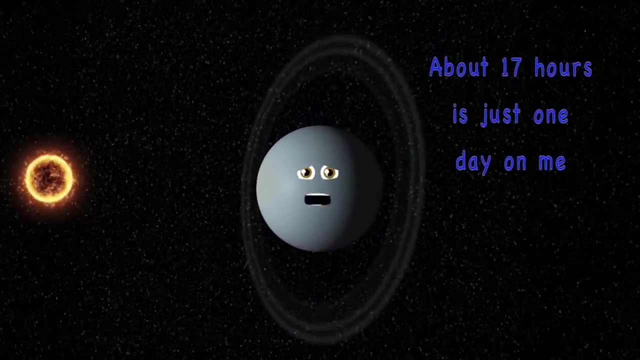 The smallest planet with the second hottest degree. My name is Mercury. no one is smaller than me. I am Uranus and I have 13 rings. now Come sing along and learn about me. Oh, I am Uranus, the seventh planet from the sun. About 17 hours is just one day on me. 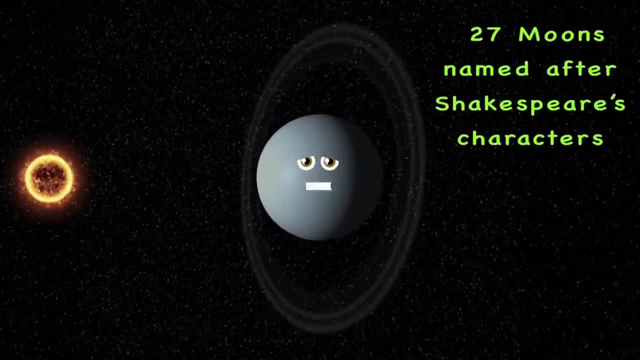 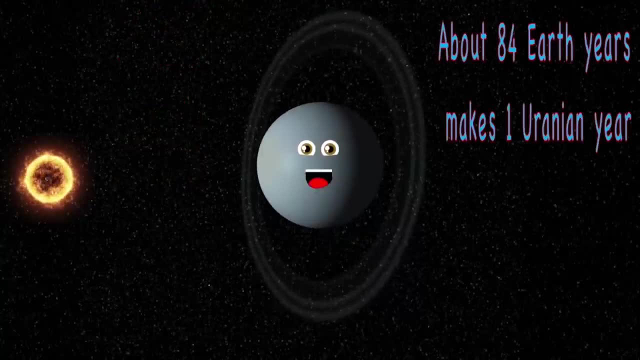 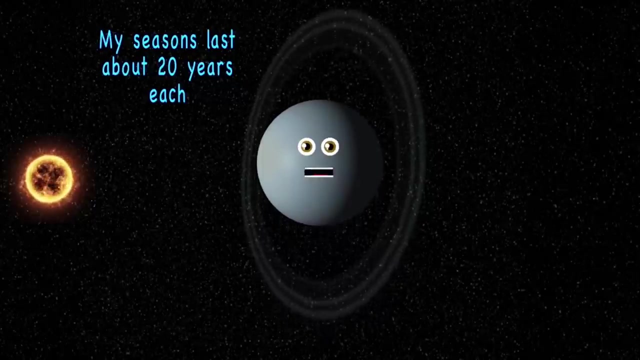 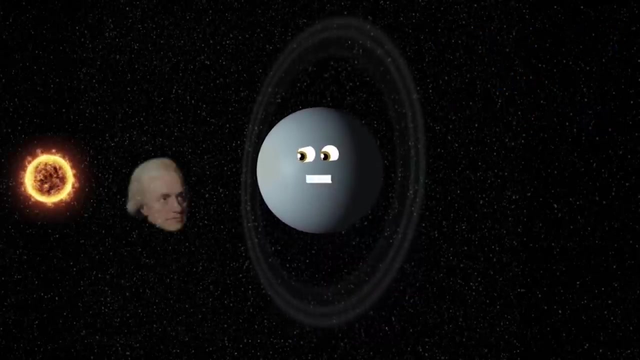 I have 27 moons named after Shakespeare characters And I have 13 rings. that you can clearly see About 84 Earth years makes just one Uranian year, And my seasons last about 20 years each. Negative 350 is my average degree And William Herschel did discover me. 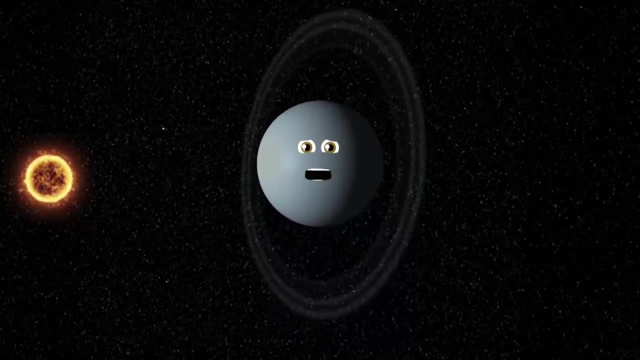 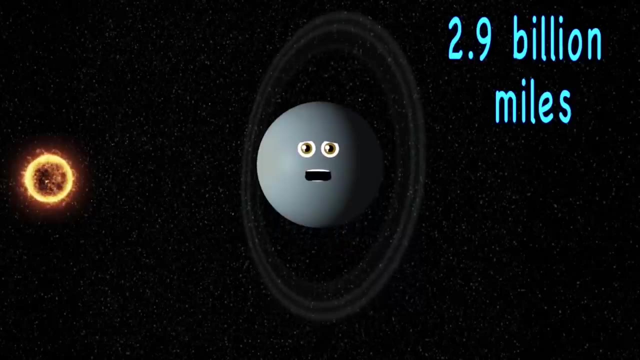 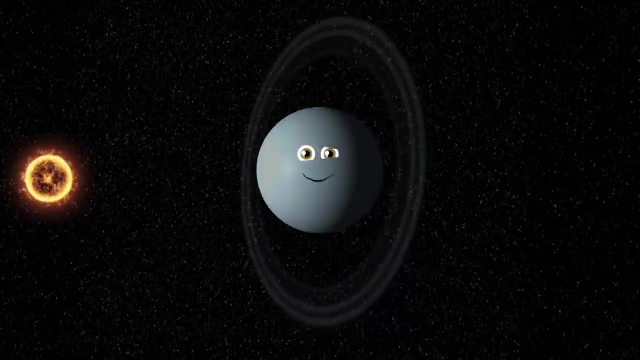 I am Uranus and I have 13 rings. now Come sing along and learn about me. 2.9 billion miles is my distance From our sun and I am an icy giant- It's so cold on me. My atmosphere is mostly made up of the following three: 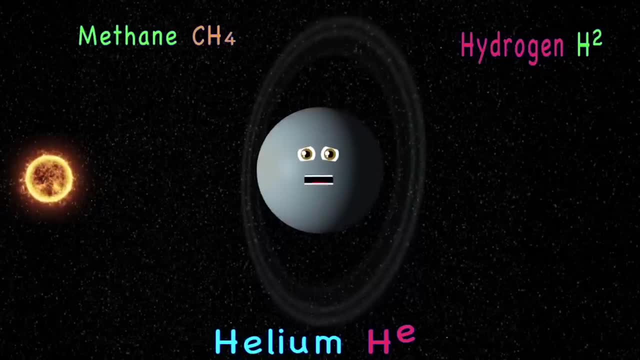 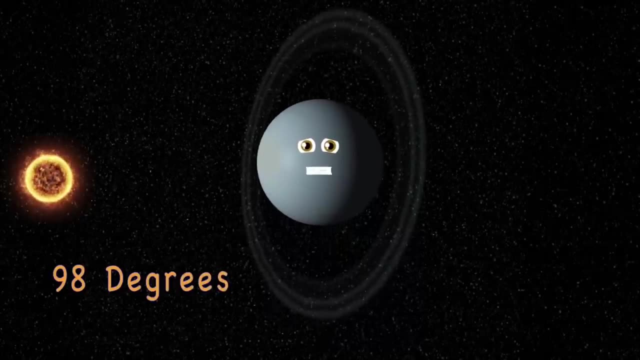 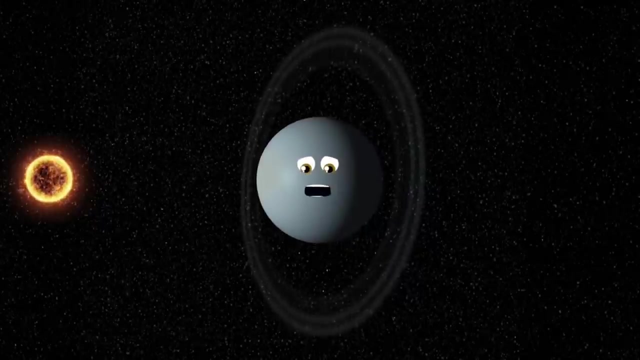 Hydrogen, methane and helium H-E. The tilt of my axis is at 98 degrees. It's one of the steepest tilts in our galaxy. Most of my mass is made up of the following three: Water, methane and ammonia, And H3. I am Uranus and I have 13 rings now. 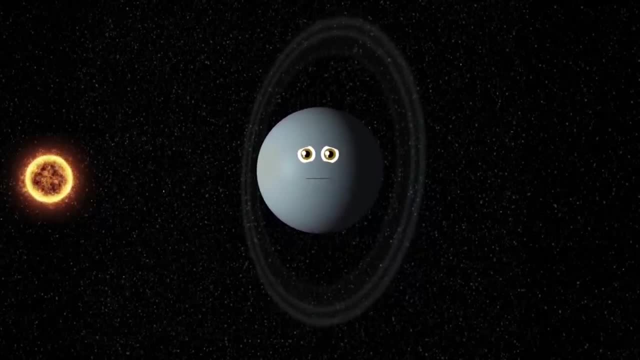 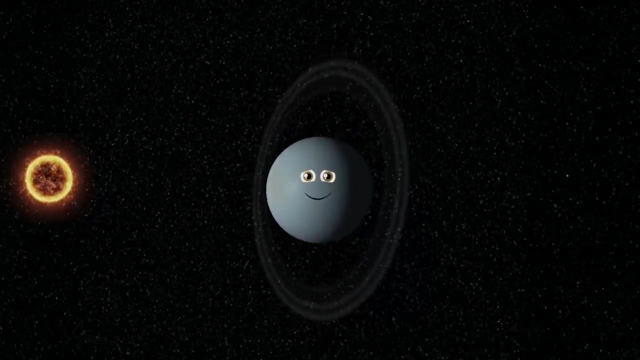 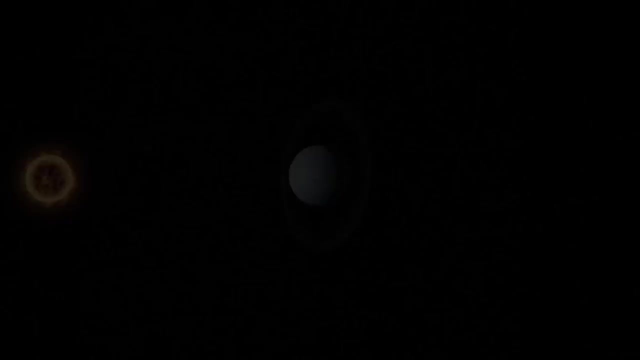 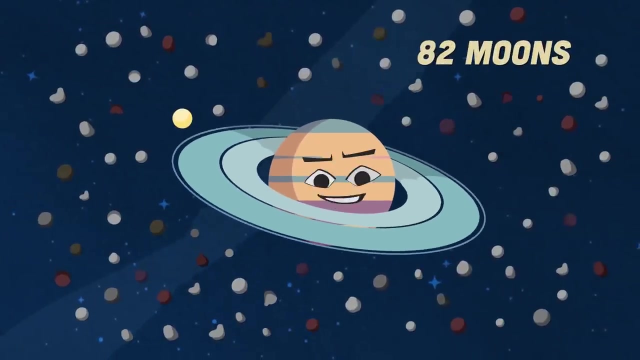 Come, sing along and learn about me. I'd like to thank you for learning about the planets on this page. Go subscribe to us please, no matter what your age. I'm Saturn and I have 82 moons From the date of this song's release. There may be more soon. 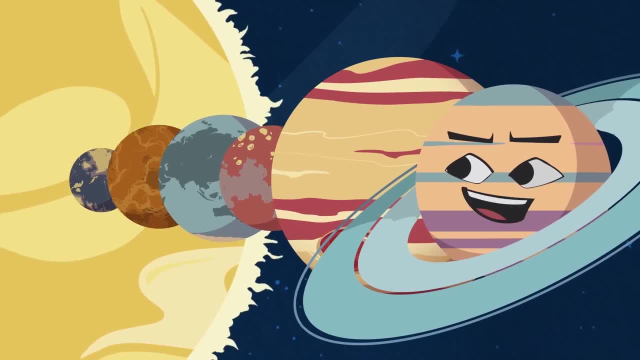 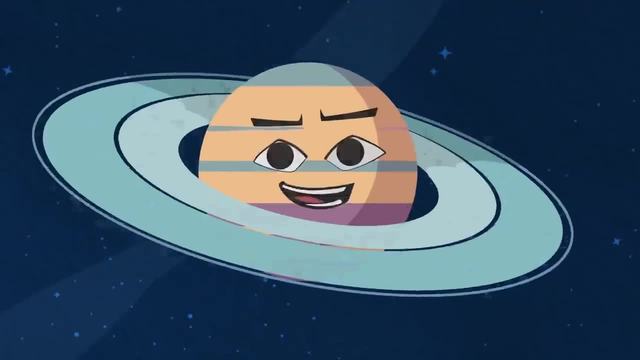 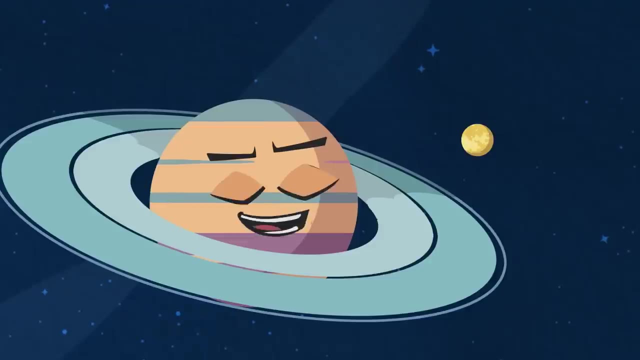 Saturn's the sixth planet from the sun, With rings that surround my planet system. These rings are made of pieces of comets and asteroids Or shattered moons- my rings you can avoid. As of the date of this video, I have 82 moons. Since 1655, my first moon tightened. 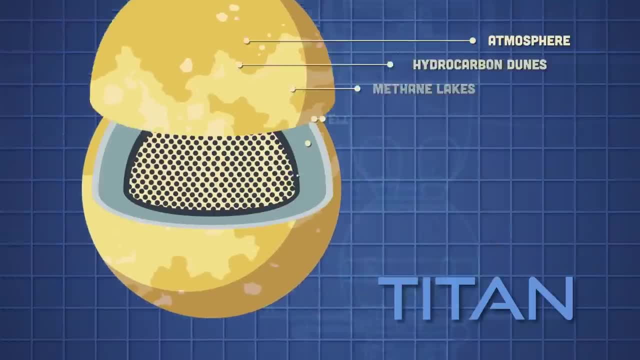 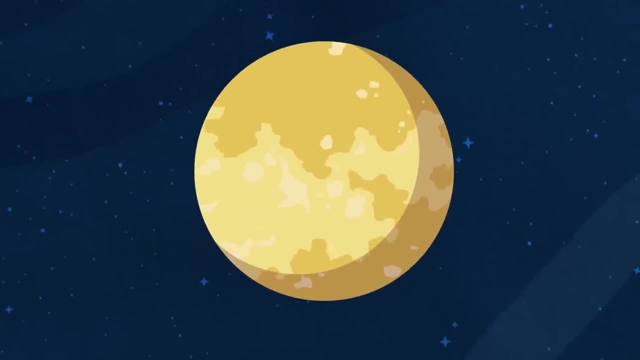 Was discovered. it's true, My largest moon is Titan, The cold and icy orb With a golden, hazy atmosphere you can't ignore. Titan is the second largest moon in the solar system After Ganymede, orbiting Jupiter where it's fun. In the future, you will learn more about my moon, Titan. When NASA launches the Dragonfly mission, It will launch in 2027 With an eight bladed drone, like craft Called the quadcopter, Making short flights around Titan's surface on its path During the 2.7 year baseline mission. I do confess Dragonfly will study how far pre-life chemistry may have progressed. 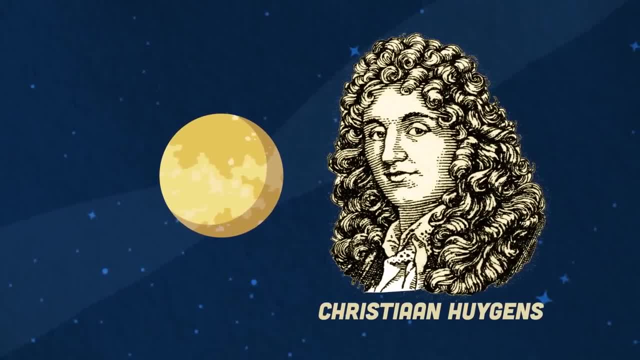 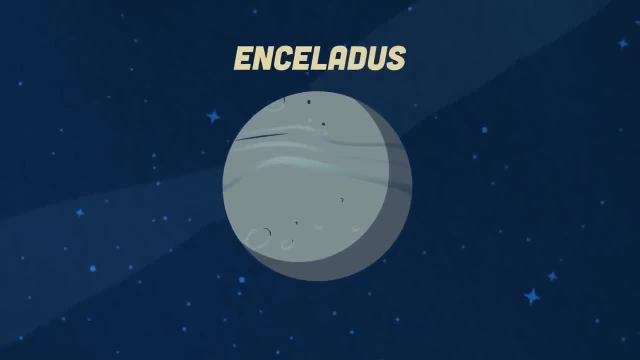 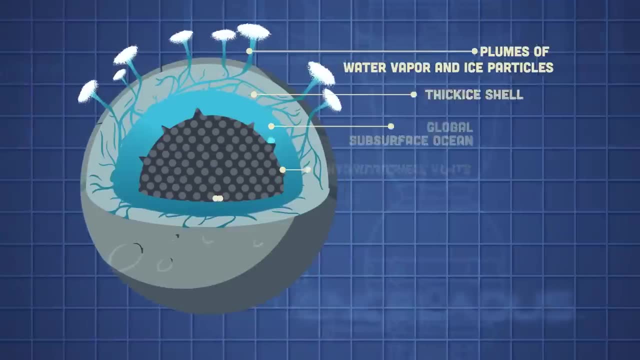 Christian Huygens made the discovery Of my largest moon, named Titan. You have seen, Enceladus is the sixth largest moon of Saturn. It's a tenth of the size of Titan, But still present. as it turns. There's a global ocean of liquid salty water beneath its crust. 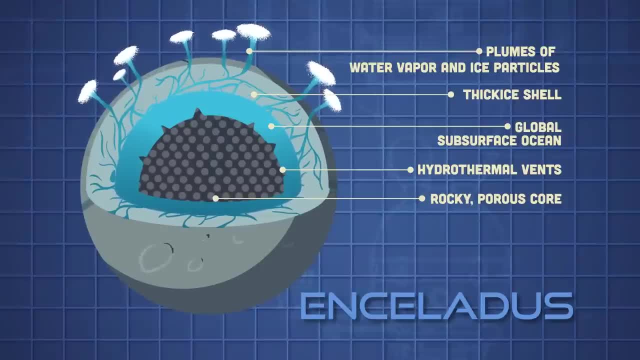 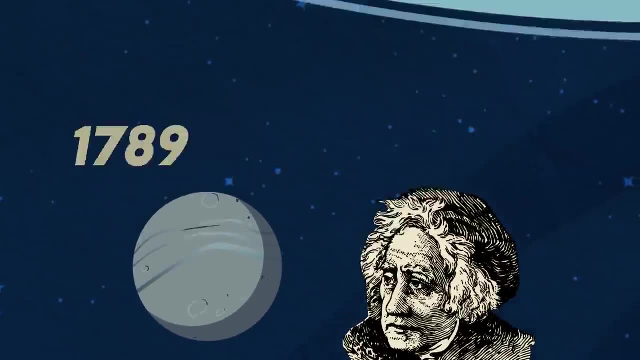 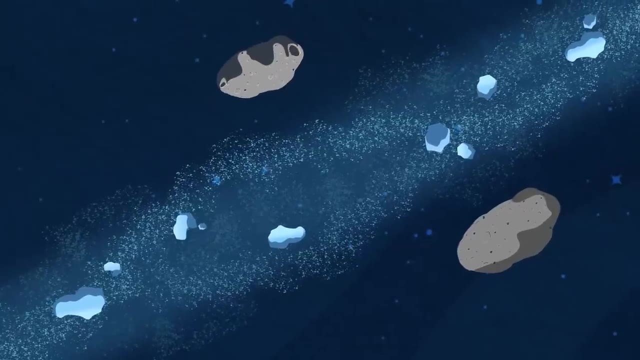 That jets icy particles into space in which it does gush. William Herschel discovered Enceladus, My moon, in 1789. Maybe you will discover more soon. Here's Prometheus and Pandora. They act as shepherds Flocking icy particles into an aeroband, I'm sure.